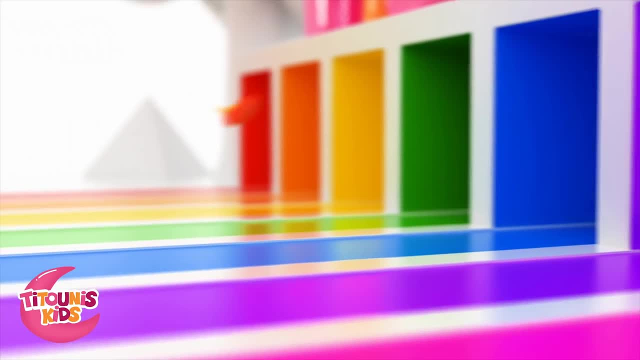 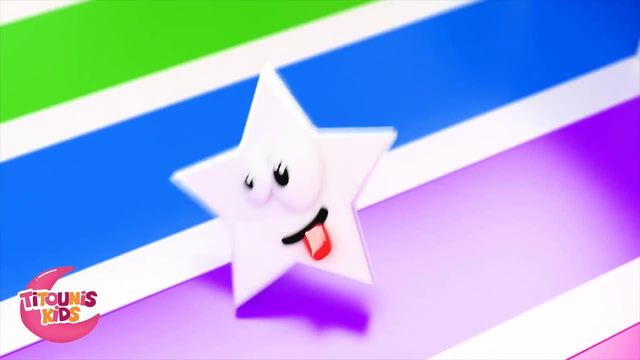 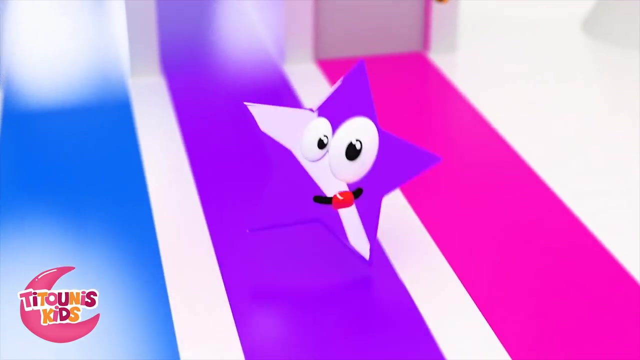 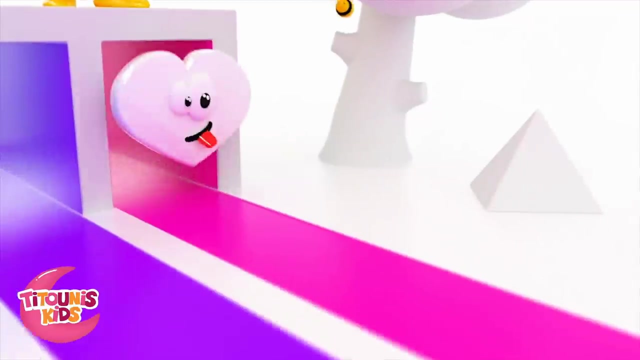 Rhombus rhombus. I have a rhombus Star star, a purple star Star star. I love the color purple. This little star is bright and purple Star star. I love the color purple. I have a star Heart heart. I have a pink heart. 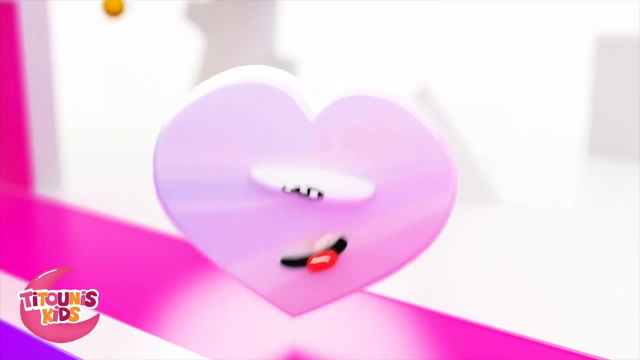 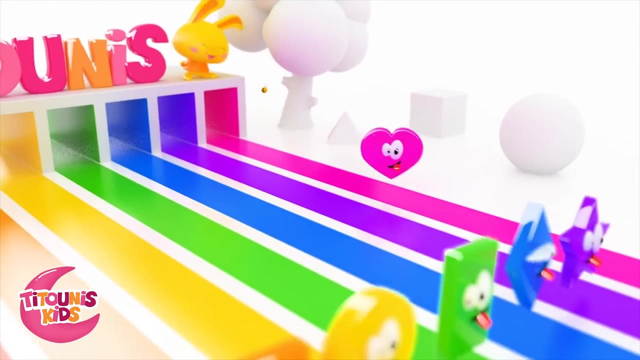 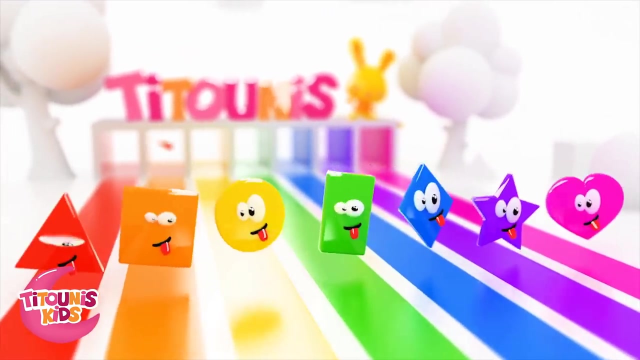 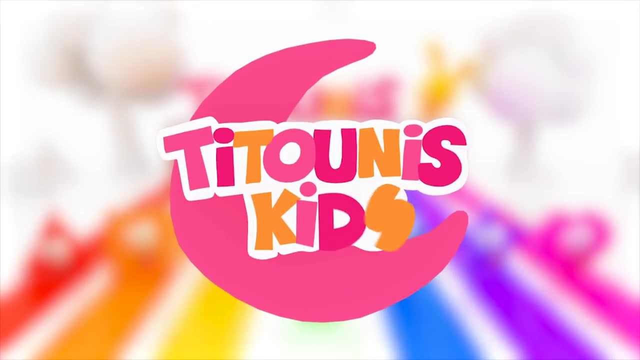 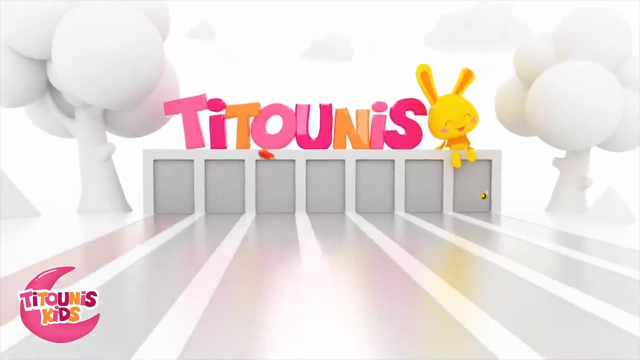 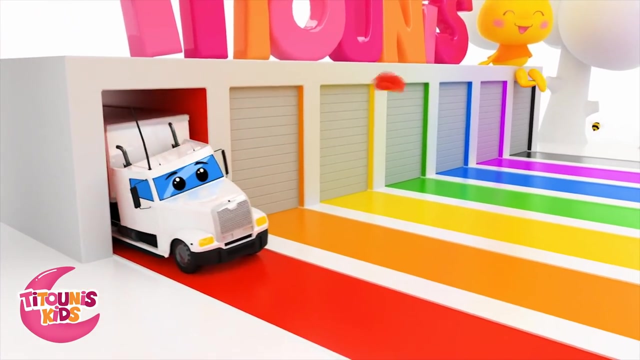 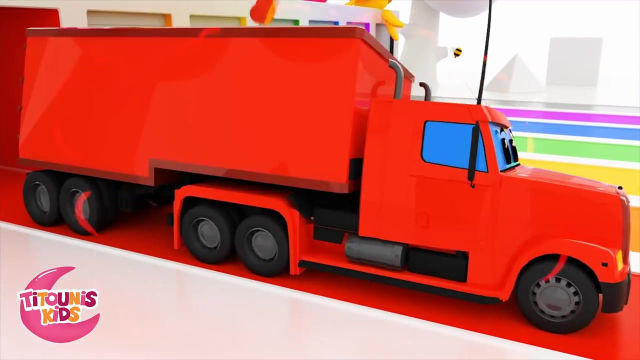 Heart heart. I love the color pink. This little heart is bright and pink Heart heart. I have a heart: Red, red, red, red. I have a red truck: Red, red, red, red. I love the color red. With this little truck I never get sick. 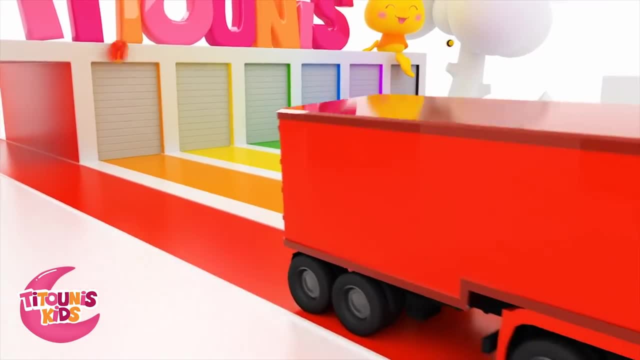 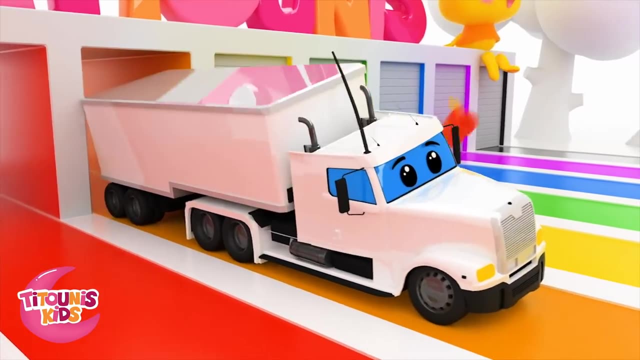 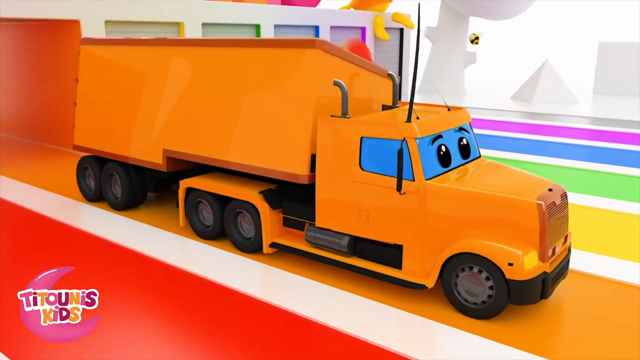 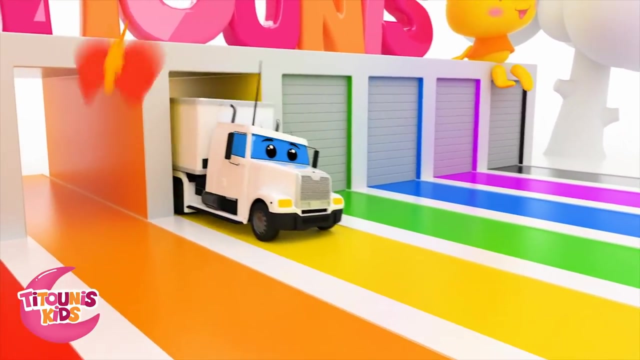 Red, red, red, red- I have a red truck. Orange, orange- I have an orange truck, Orange, orange- I love the color orange. With this little truck I never get sick. Orange, orange- I have an orange truck. Yellow, yellow- I have a yellow truck. 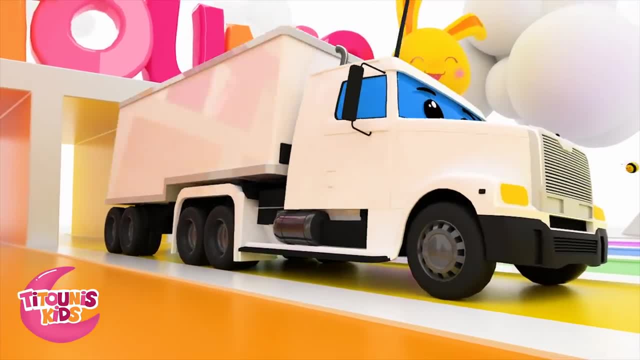 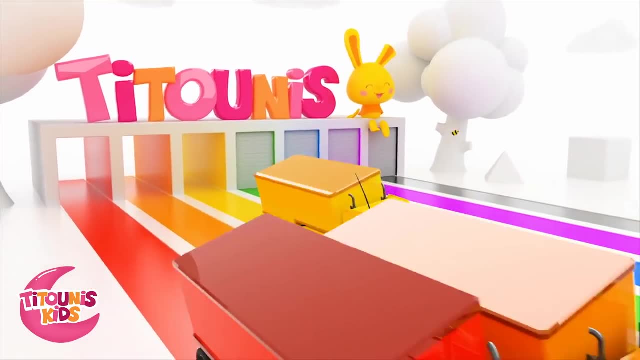 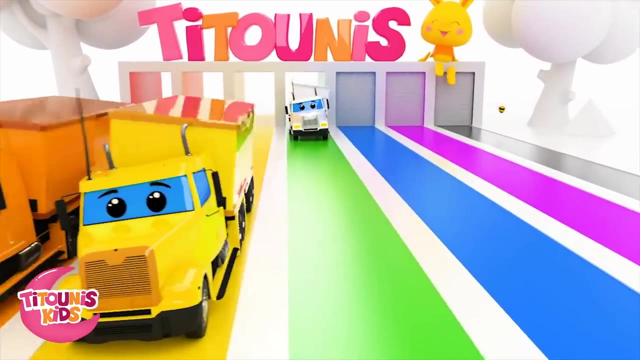 Yellow, yellow. I love the yellow one. With this little truck I never get sick, I never get stuck. Yellow, yellow, I have a yellow truck. Green green, green green. I have a green truck. Green, green, green green. I love the color green. 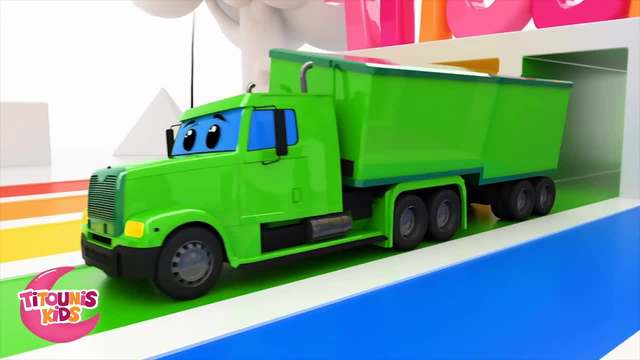 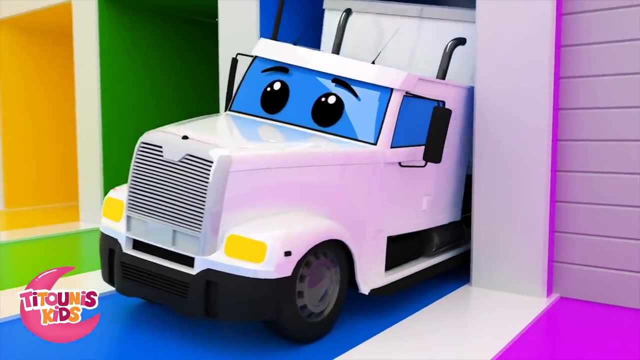 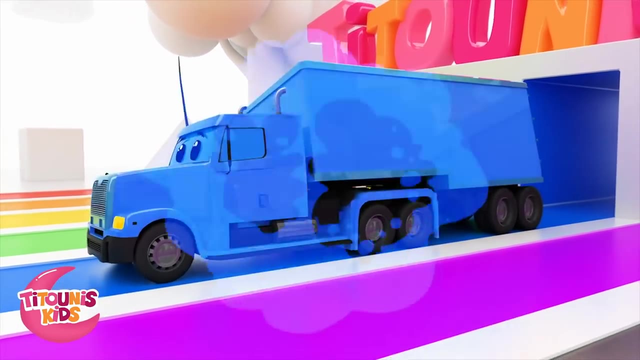 With this little truck, I never get stuck. Green, green, green, green- I have a green truck. Blue blue, blue, blue, I have a blue truck. Blue, blue, blue, blue, Blue, blue, blue- I love the color blue. With this little truck, I never get stuck. 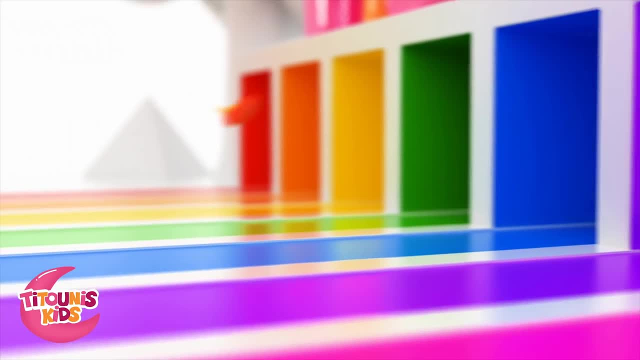 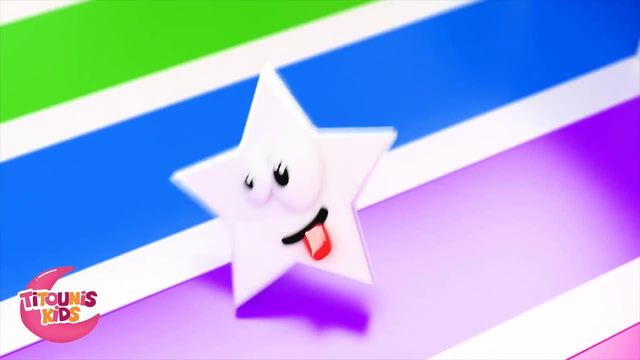 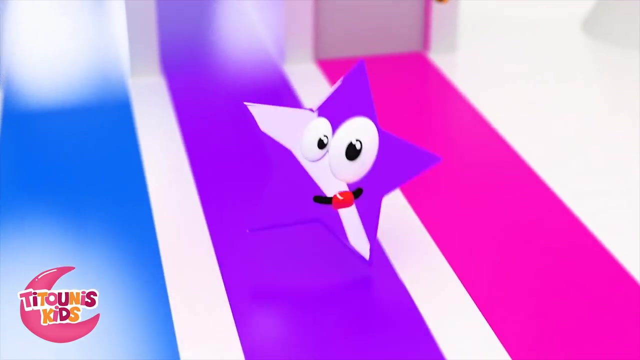 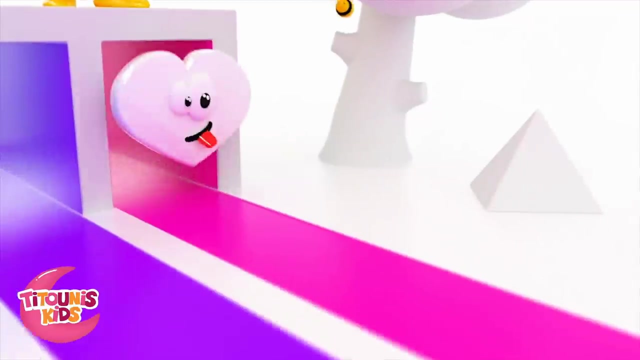 Rhombus rhombus. I have a rhombus Star star, a purple star Star star. I love the color purple. This little star is bright and purple Star star. I love the color purple. I have a star Heart heart. I have a pink heart. 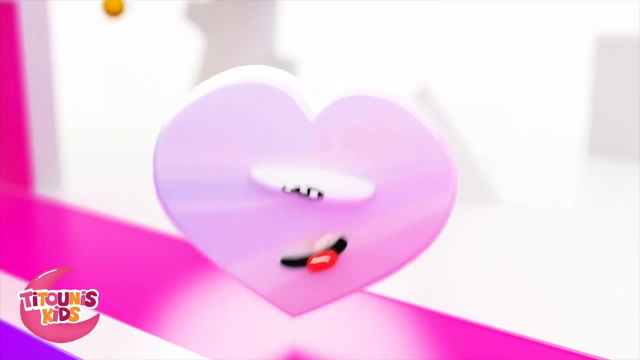 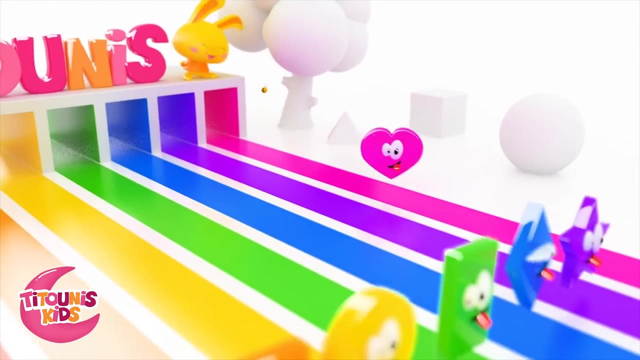 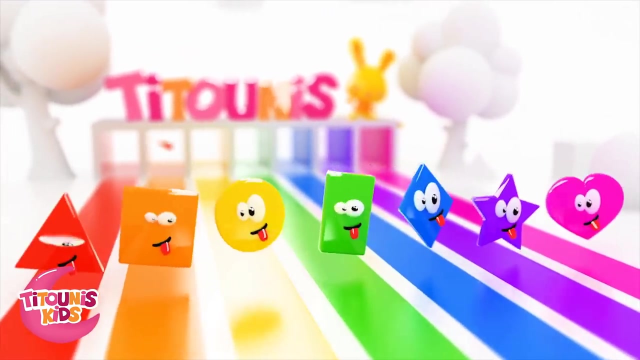 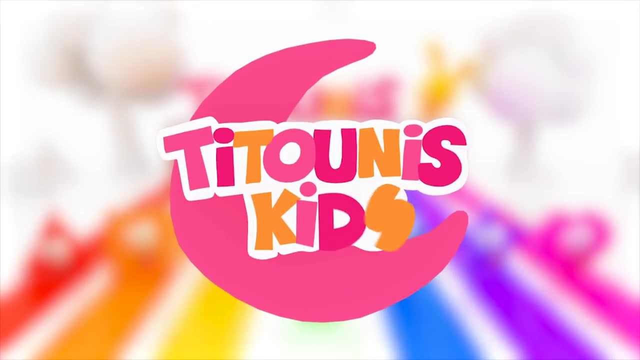 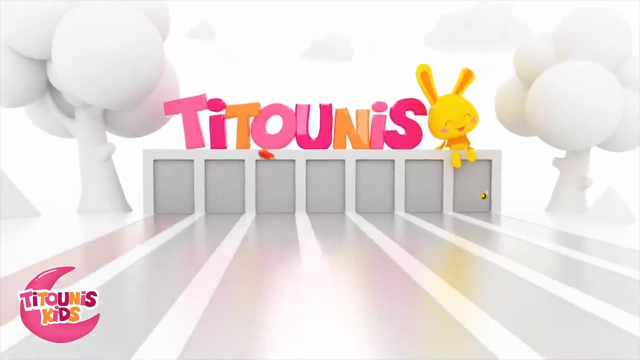 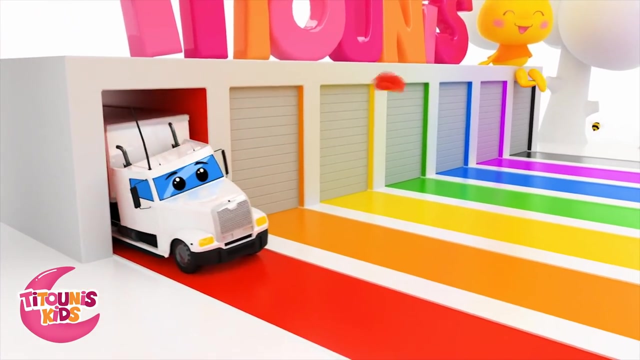 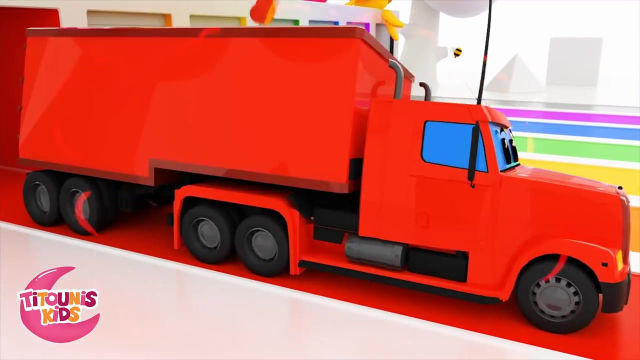 Heart heart. I love the color pink. This little heart is bright and pink Heart heart. I have a heart: Red, red, red, red. I have a red truck: Red, red, red, red. I love the color red. With this little truck I never get sick. 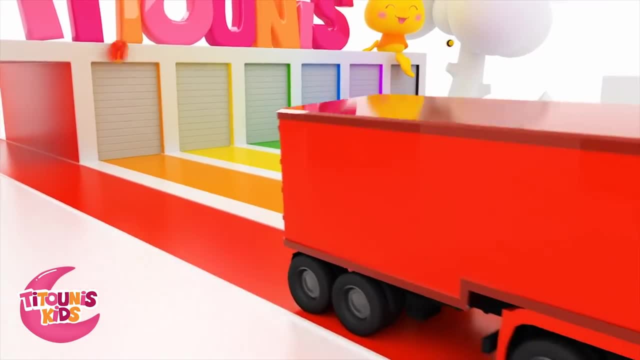 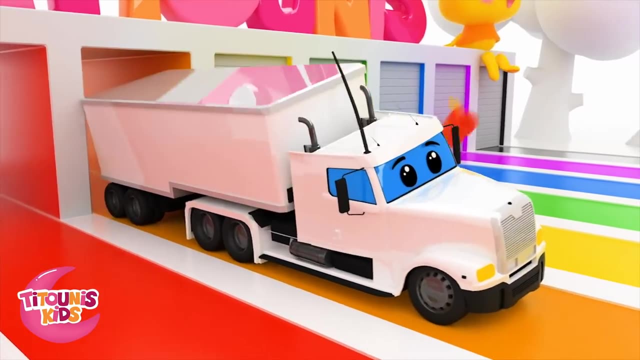 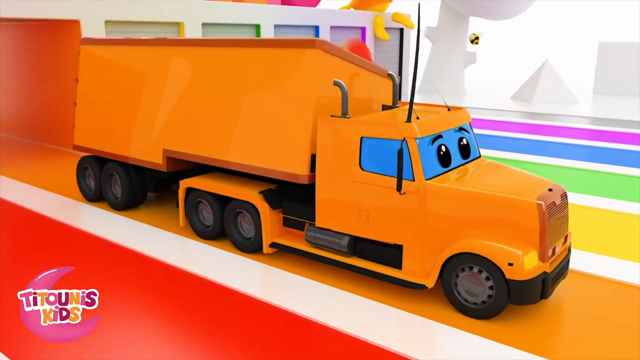 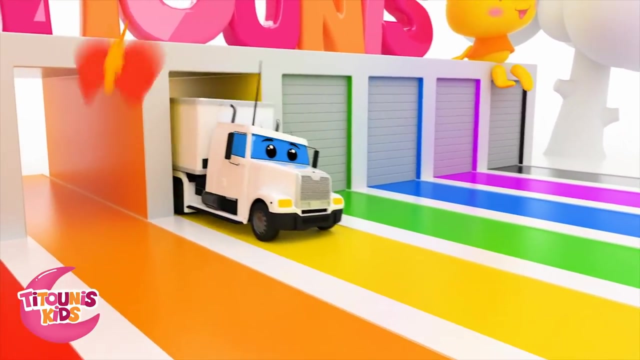 Red, red, red, red- I have a red truck. Orange, orange- I have an orange truck, Orange, orange- I love the color orange. With this little truck I never get sick. Orange, orange- I have an orange truck. Yellow, yellow- I have a yellow truck. 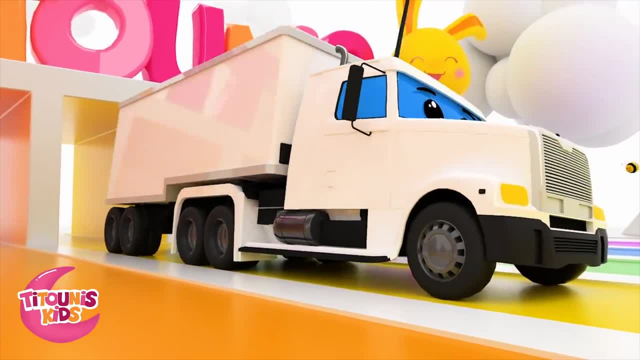 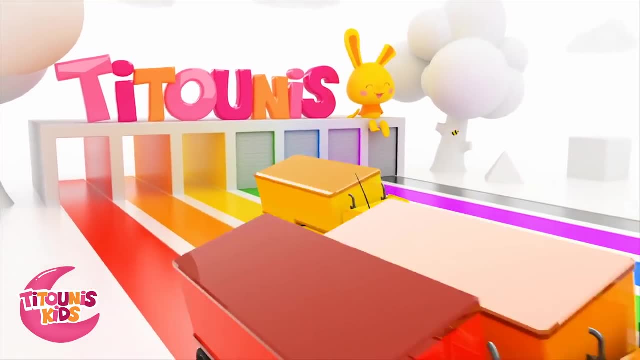 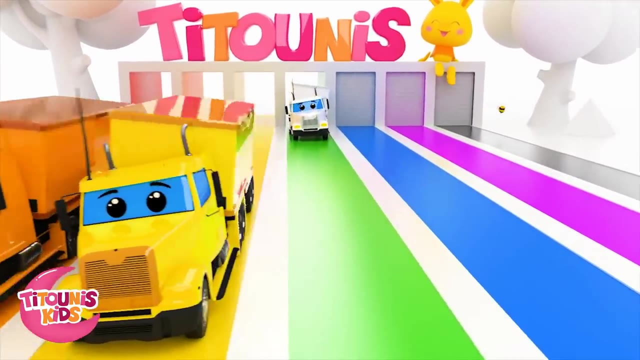 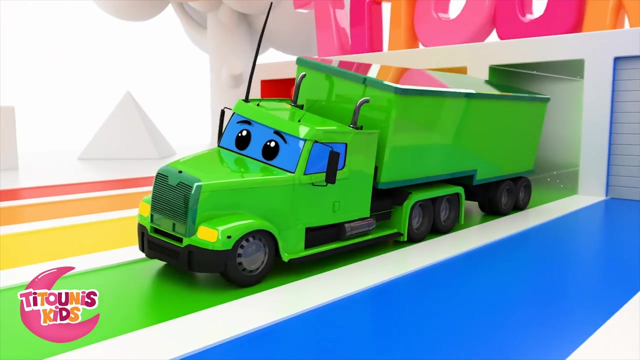 Yellow, yellow- I love the yellow one. With this little truck, I never get sick. Yellow, yellow- I have a yellow truck. Green green green- I have a green truck. Green green green- I love the color green. With this little truck, I never get sick. 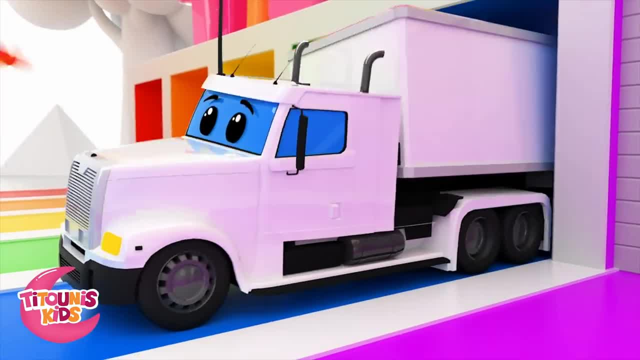 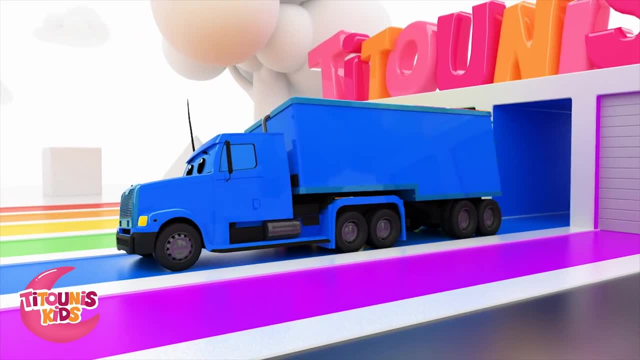 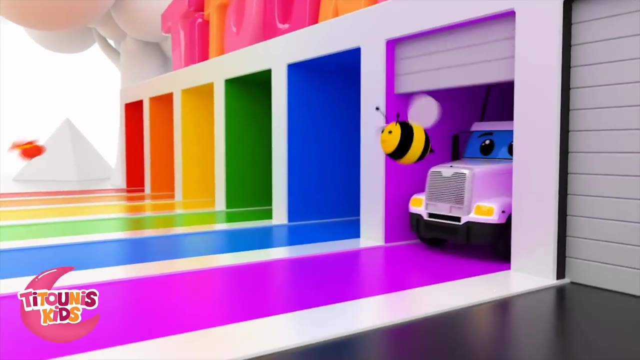 Green, green, green- I have a green truck. Blue blue, blue, blue- I have a blue truck. Blue blue- I love the color blue. With this little truck I never get stuck. Blue, blue, blue, blue- I have a blue truck. Purple, purple: I have a purple truck. 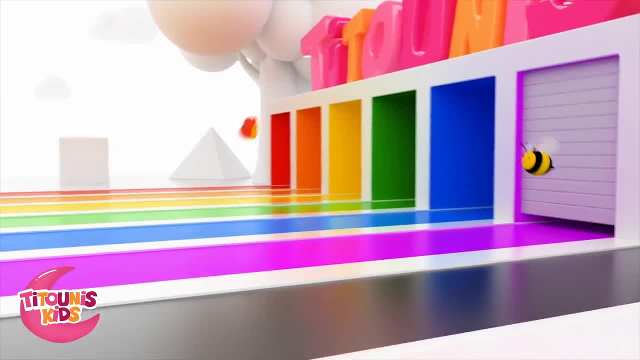 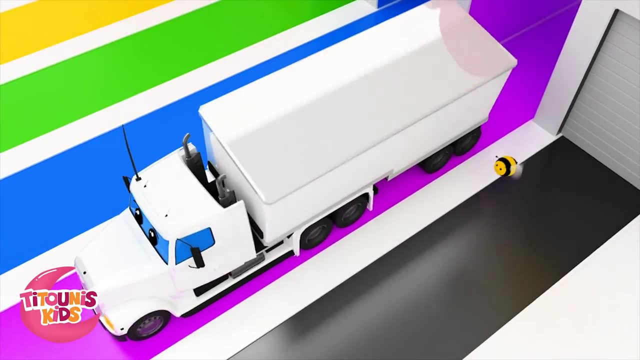 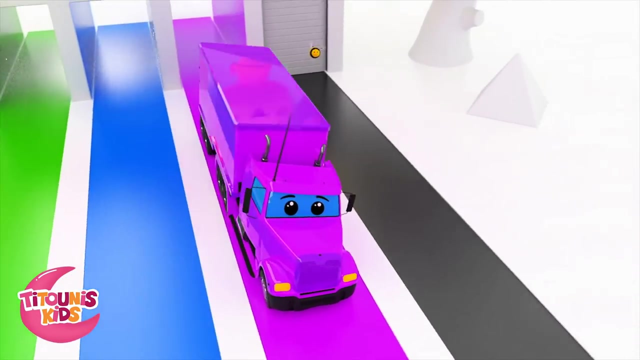 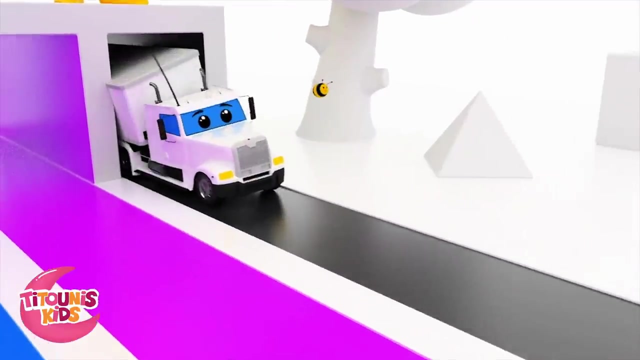 Blue, blue, blue blue. I have a blue truck. Purple purple: I have a purple truck, Purple purple. I love the purple one. With this little truck I never get stuck. Purple purple: I have a purple truck. Black, black, black, black: I have a black truck. 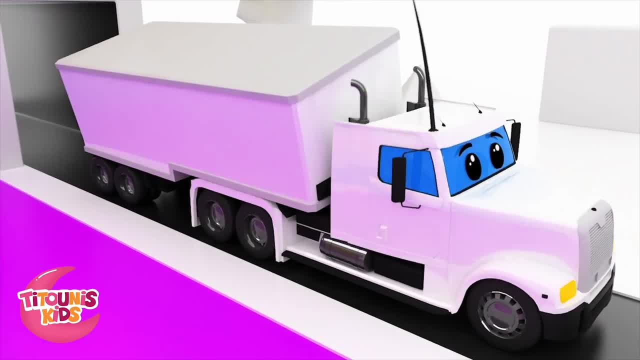 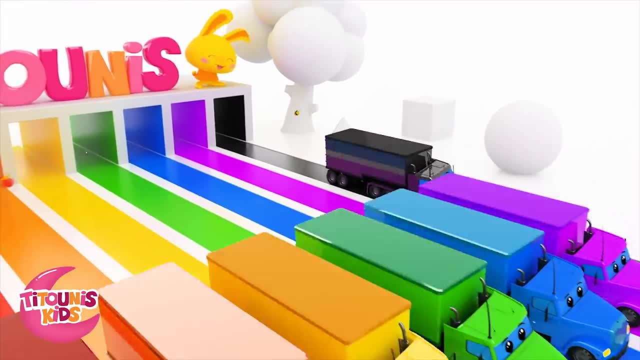 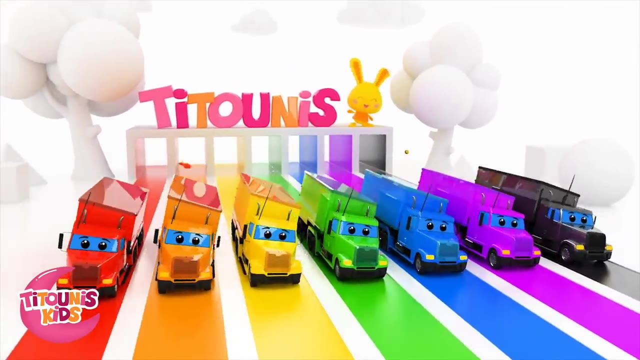 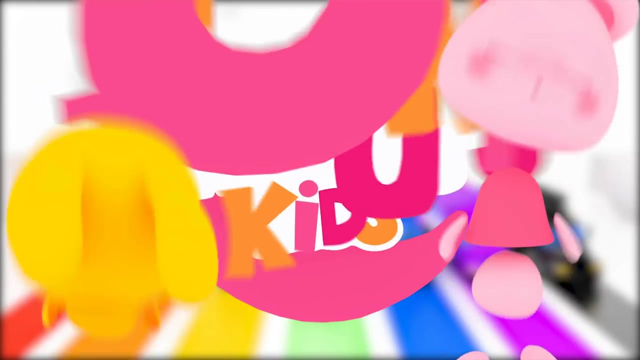 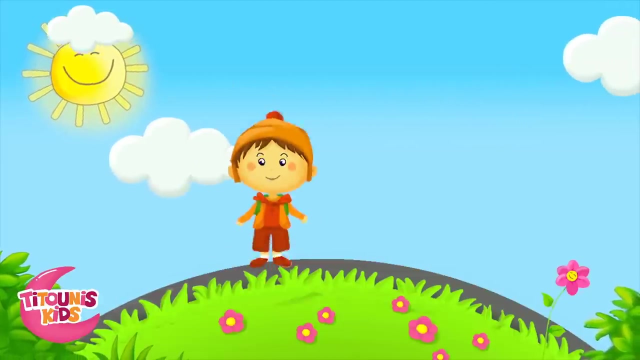 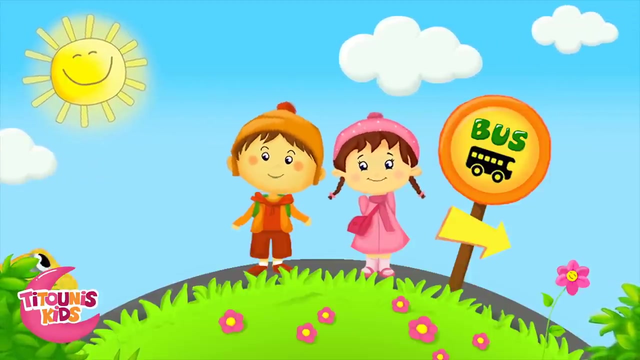 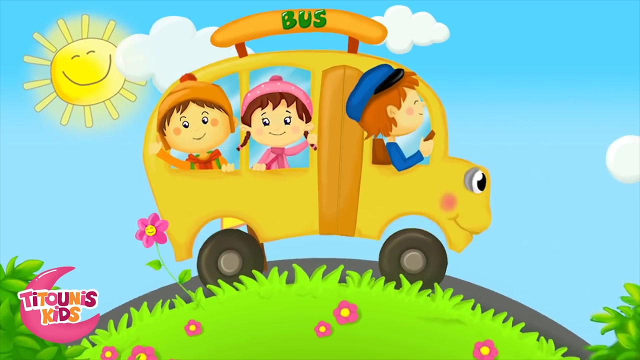 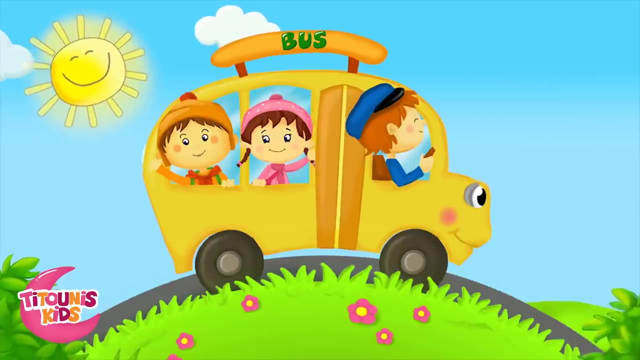 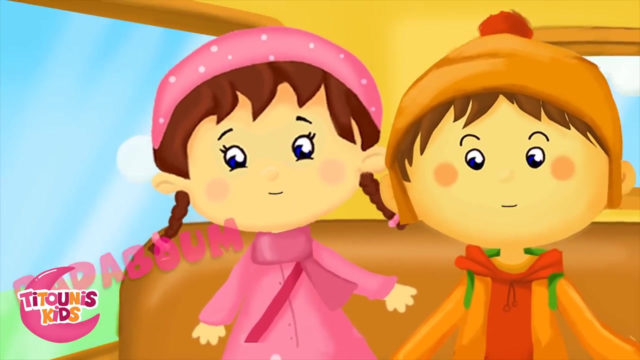 Black, black, black, black. I love the color black. With this little truck I never get sick. Black, black, black, black. I have a black truck. I love the color black. All through the town the passengers go bouncing ba-da-boom, ba-da-boom, ba-da-boom. 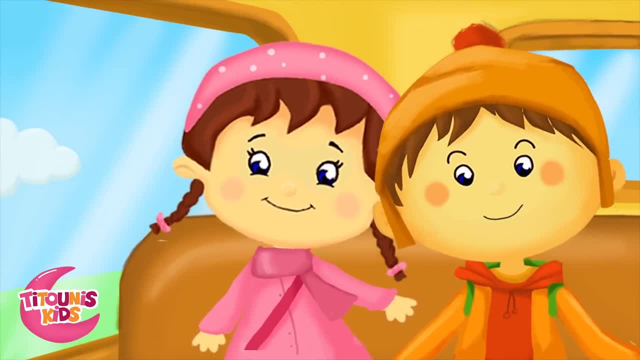 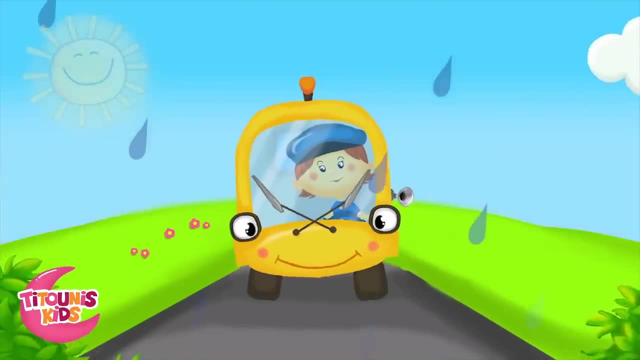 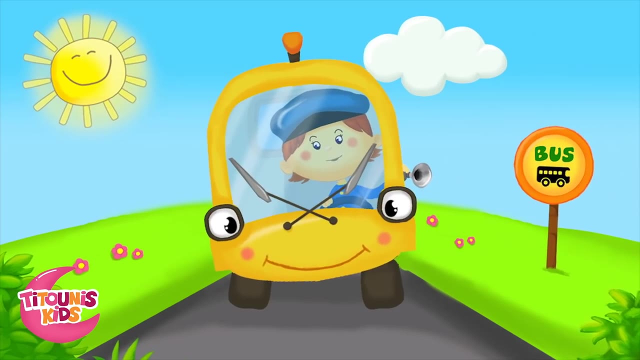 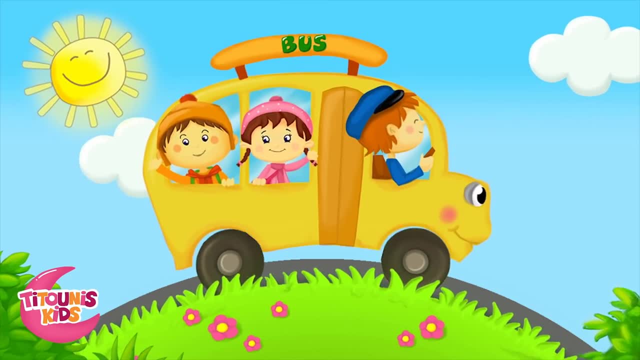 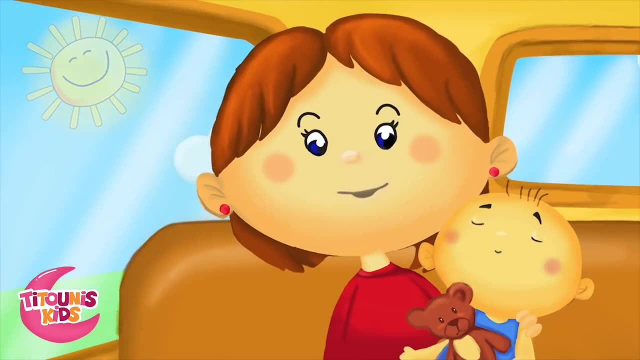 The wheels on the bus go round and round, round and round, round and round. The wheels on the bus go round and round all through the town. The motor cycles go vroom, vroom, vroom, vroom, vroom, vroom, vroom. 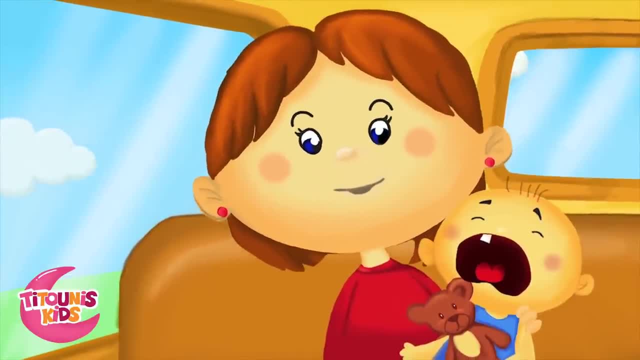 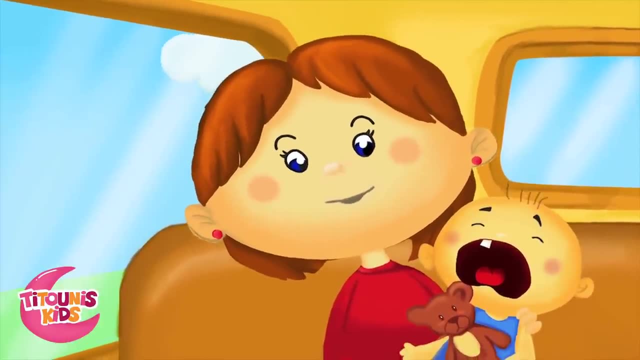 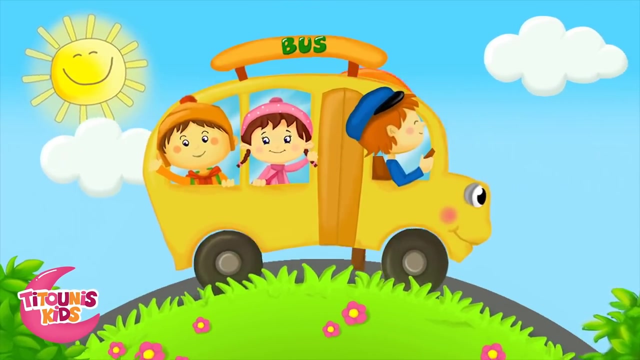 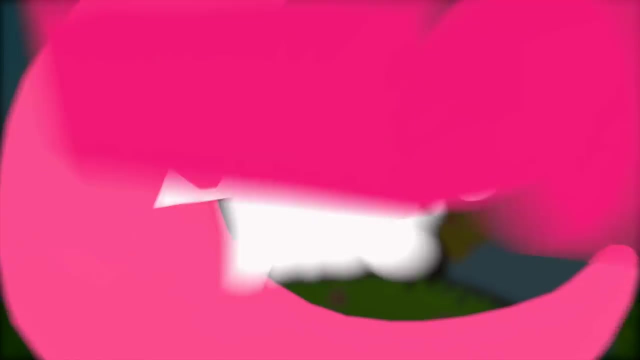 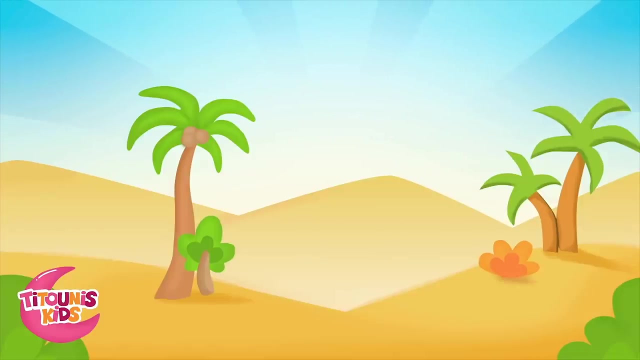 The motor cycles go vroom, vroom, vroom, all through the town. All the vehicles go round and round, round and round, round and round. All the vehicles go round and round all through the town. Once, a crocodile set off to fight a battle. 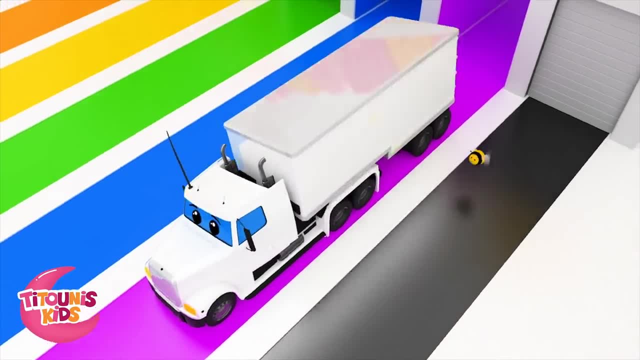 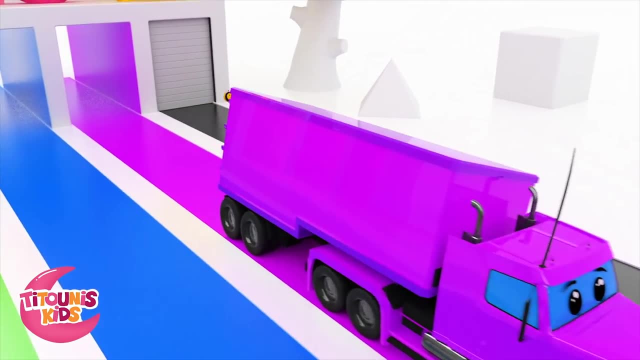 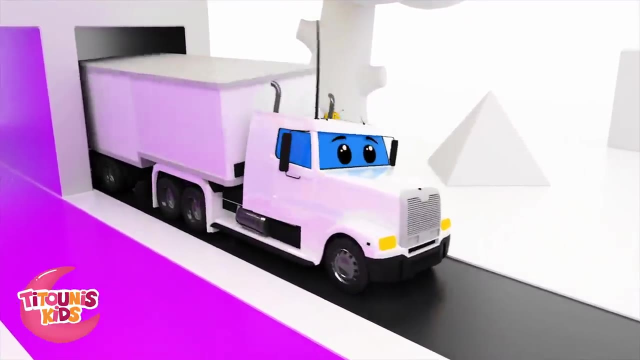 Purple, purple. I love the purple one. With this little truck I never get stuck. Purple, purple, I have a purple truck. Black, black, black, black. I have a black truck. Black, black, black, black. I love the color black. 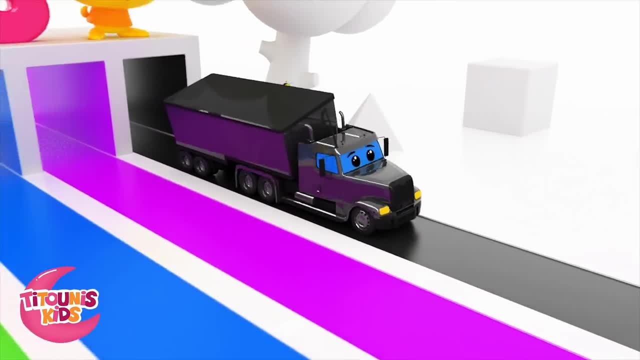 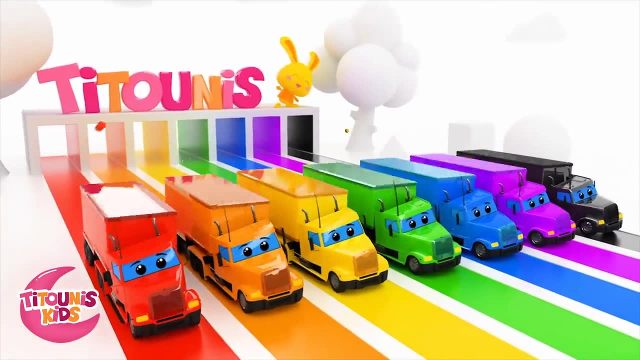 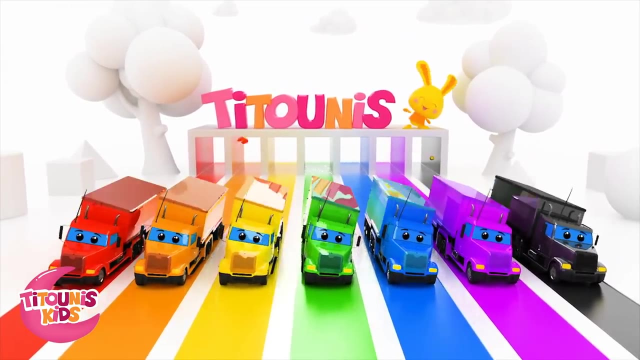 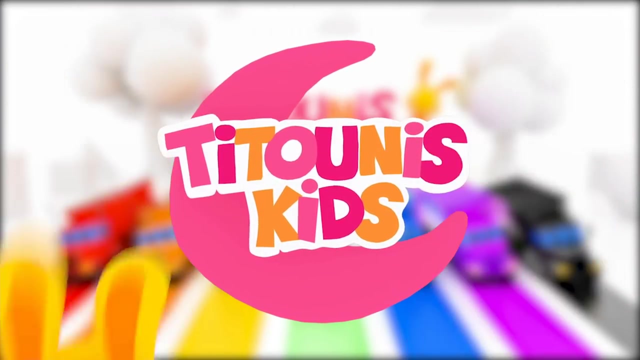 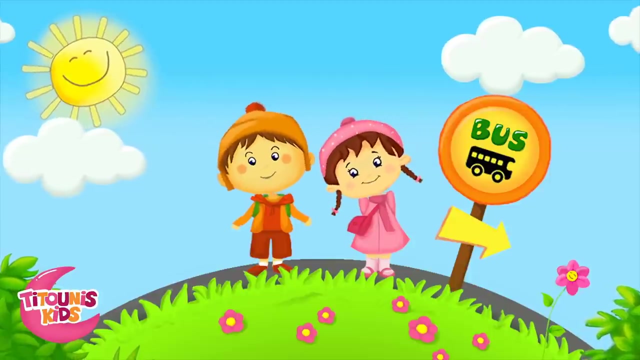 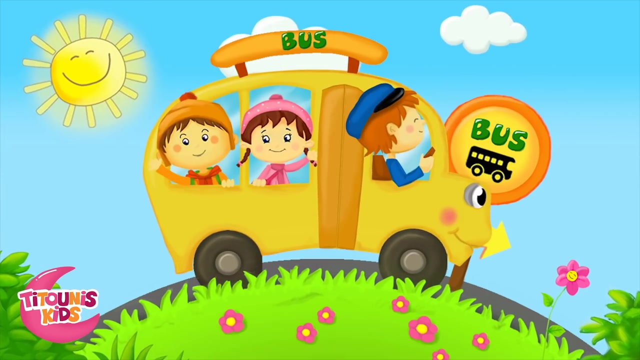 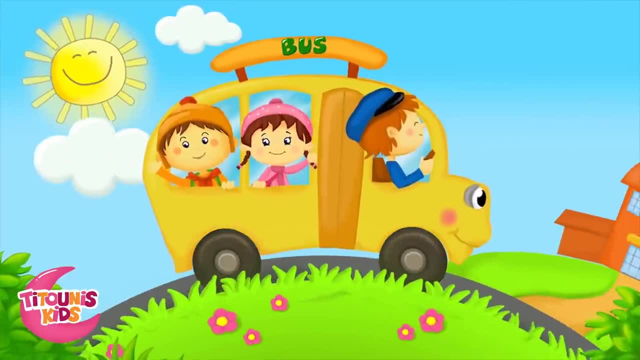 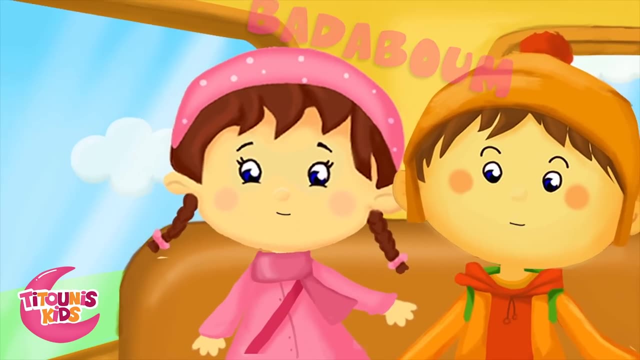 I bean them right out of the window. I bean them right out of the window. Open and shut, open and shut. the doors on the bus go open and shut All through the town. The passengers go bouncing, ba-da-boom, ba-da-boom, ba-da-boom. 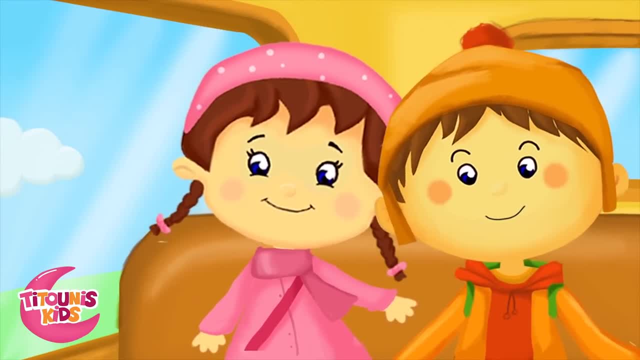 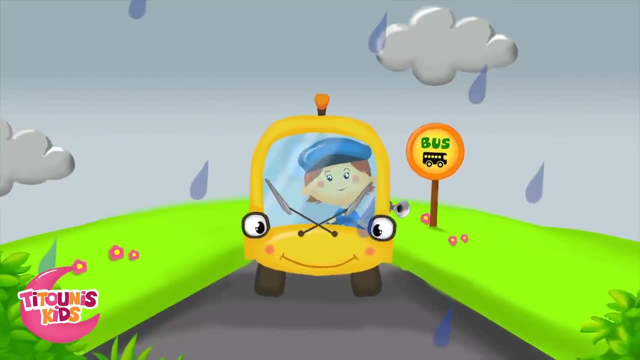 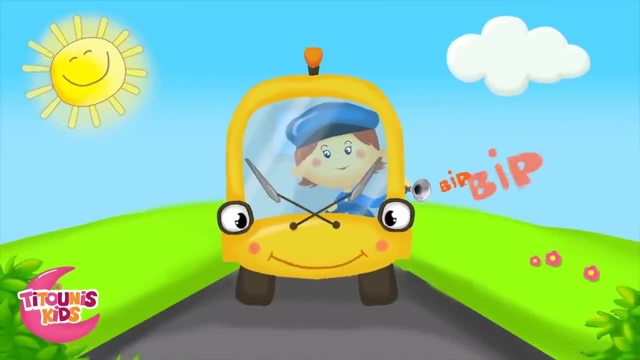 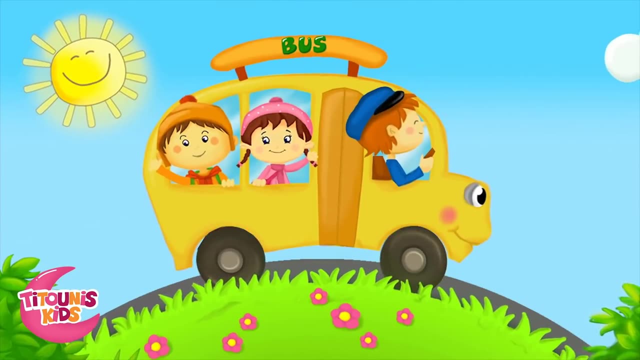 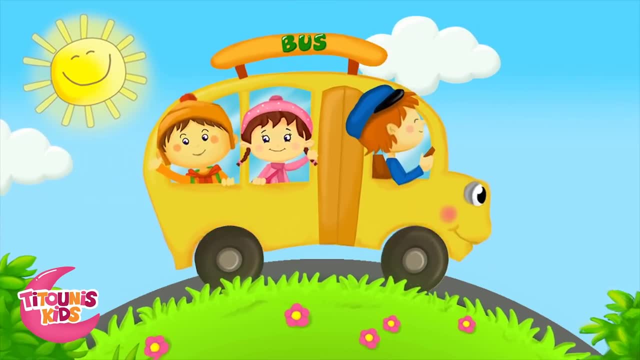 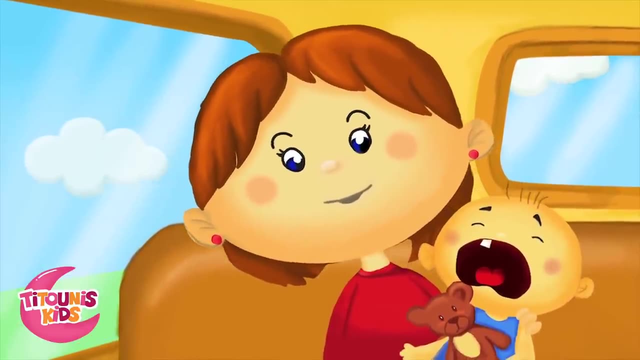 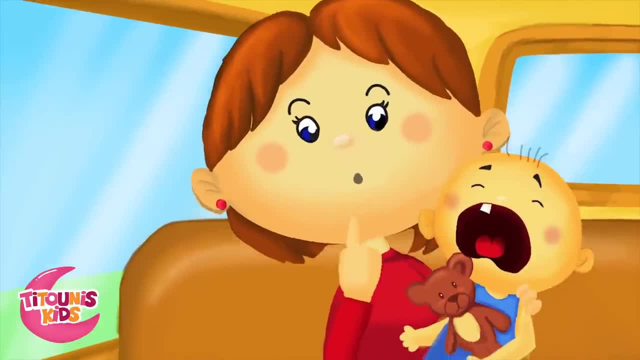 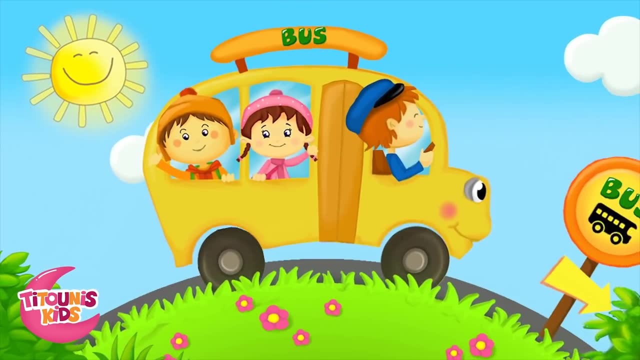 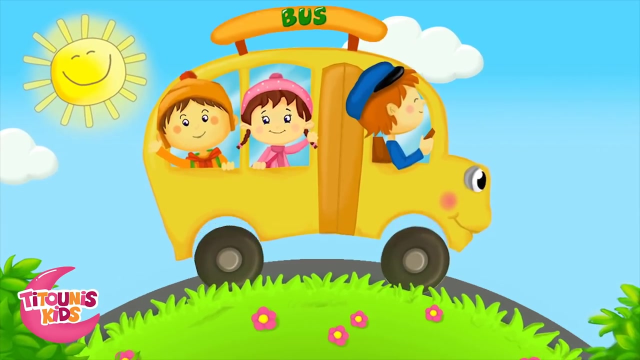 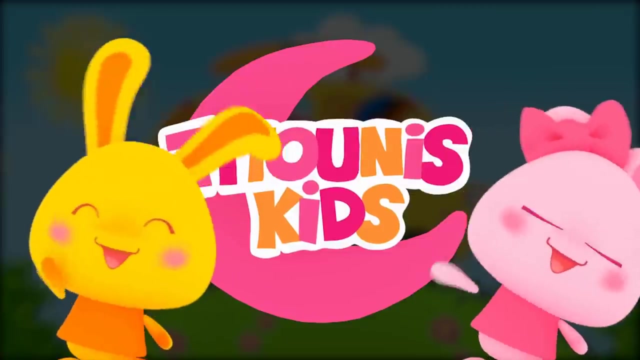 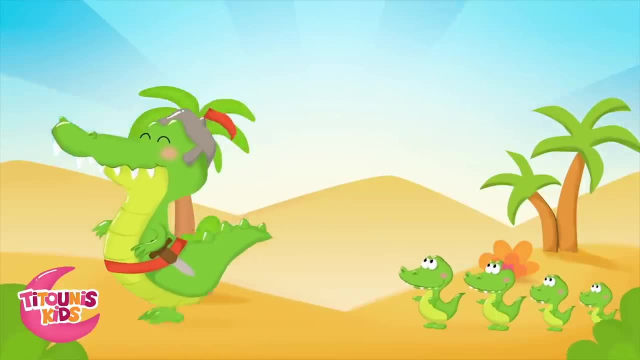 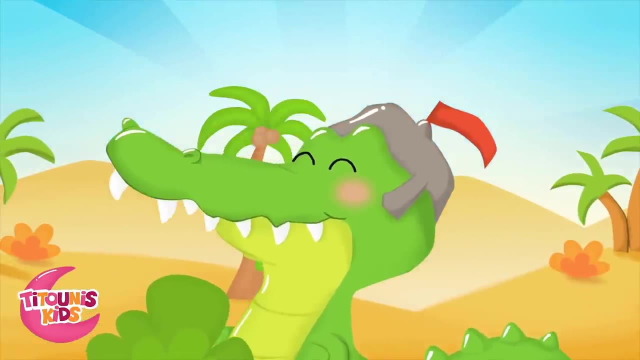 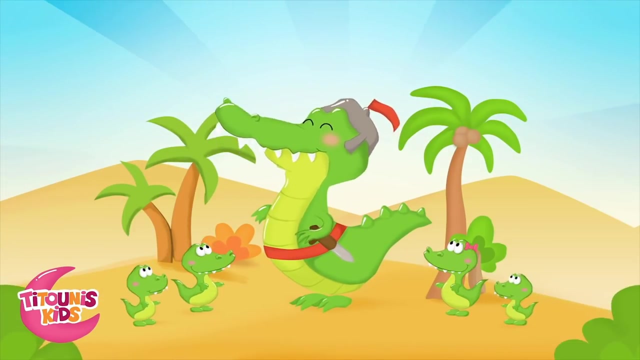 To fight a battle. He said goodbye to all his family. Off through the dust, he marches without fear, Wagging his tail in search of elephants. Oh, the crow, crow crow, the crow, crow crow, The crocodiles are marching to the Nile. 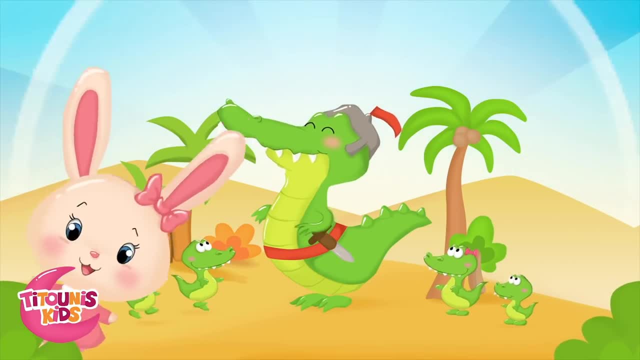 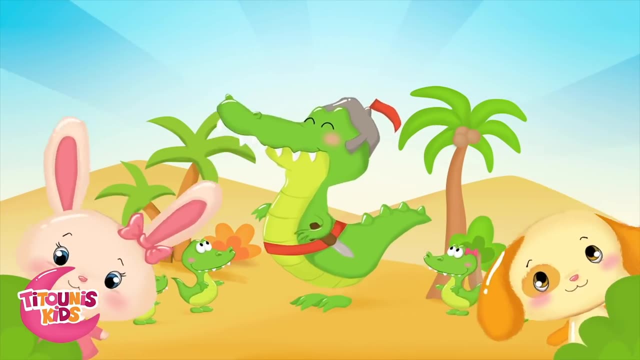 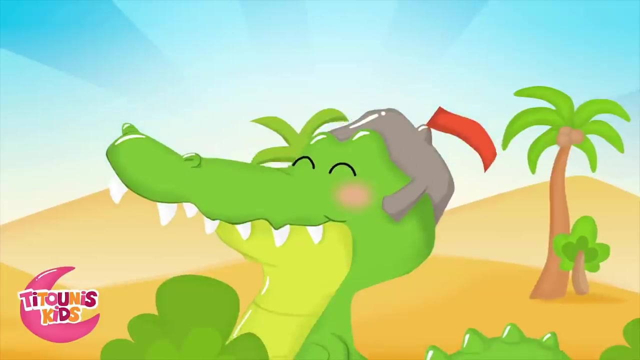 To find an elephant. Oh, the crow crow crow, the crow crow crow, The crocodiles are marching to the Nile To find an elephant, To find an elephant. Walking along, they sang their battle songs, Chomping the worms with lots of shiny teeth. 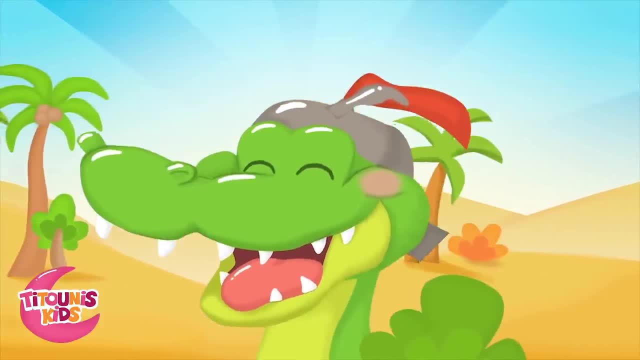 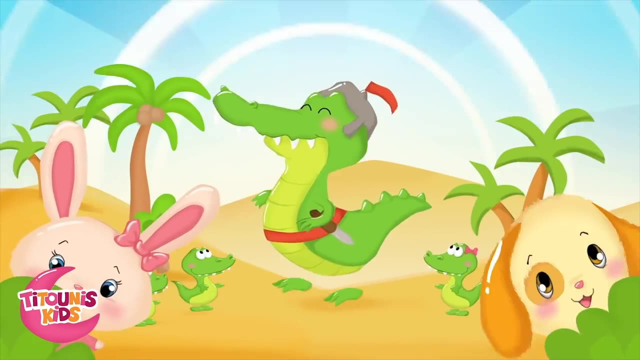 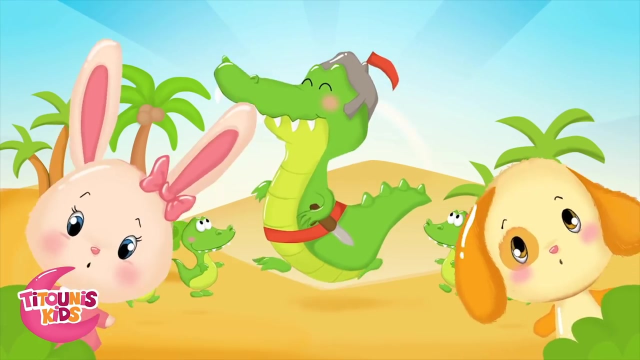 If you could see them walking there so proudly, You wouldn't want to be their enemy. Oh the crow crow crow, the crow crow crow. The crocodiles are marching to the Nile To find an elephant. Oh the crow crow crow, the crow crow crow. 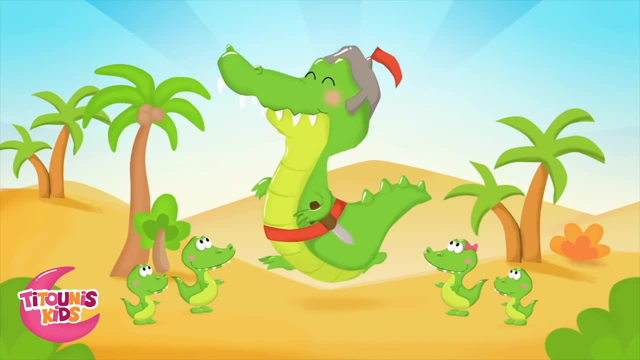 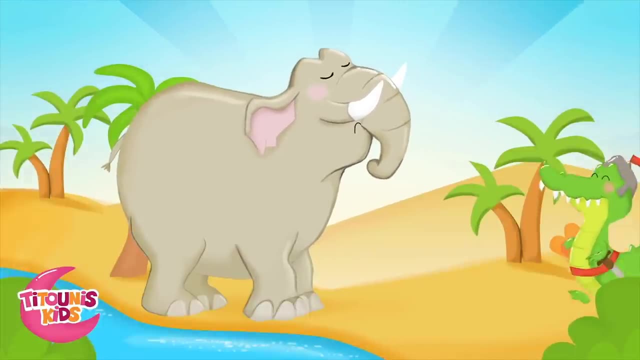 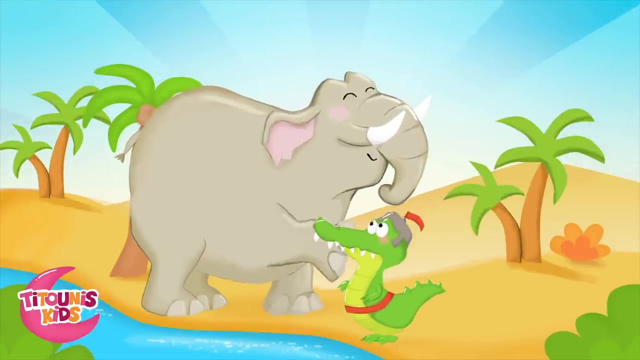 The crocodiles are marching to the Nile To find an elephant. When they arrived, the elephants were waiting. This great battle is about to begin. Oh, crocodile, it's better to start running, Jumping to the river. you have to swim away. Oh, the crocodile is marching to the Nile. 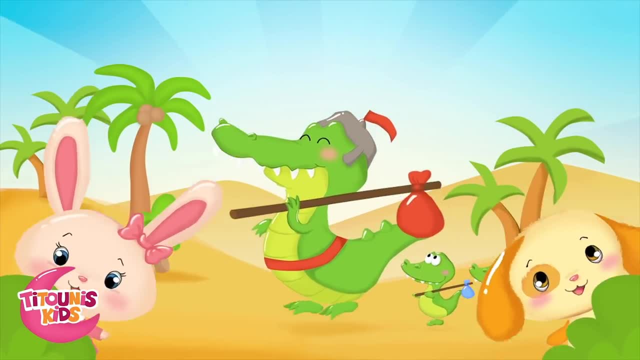 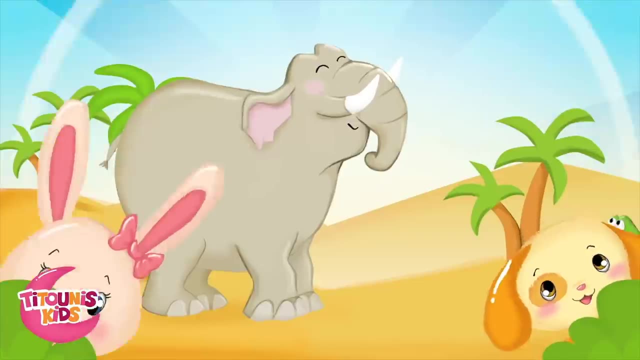 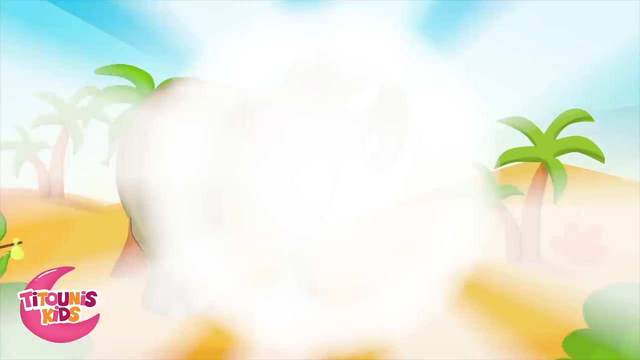 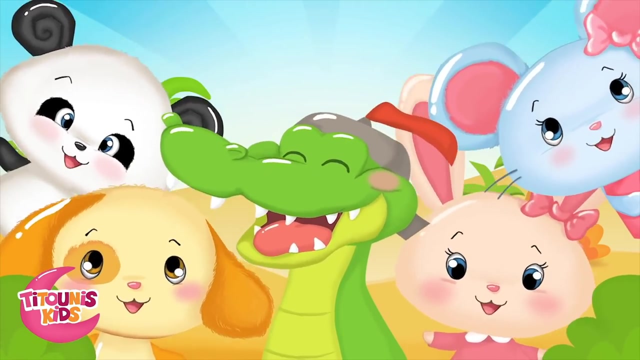 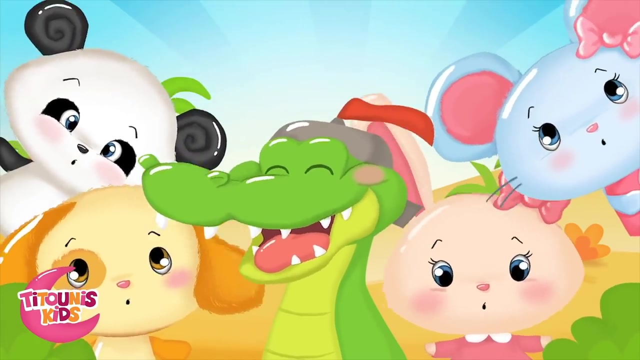 Oh, the crocodile is marching to the Nile Chugging its�ar To find the elephant. Oh, the crow crow, the cro, cro cro, the crocodile Chugging its own Crocodiles are marching to the Nile To find an elephant. 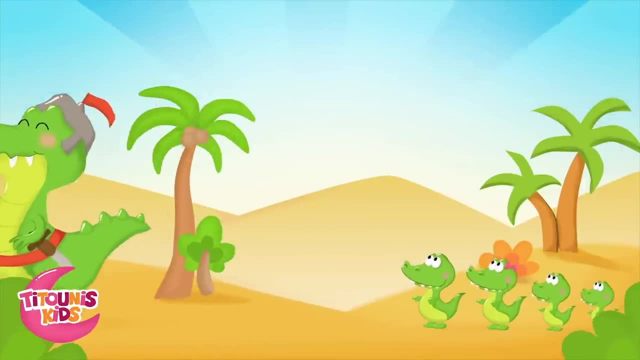 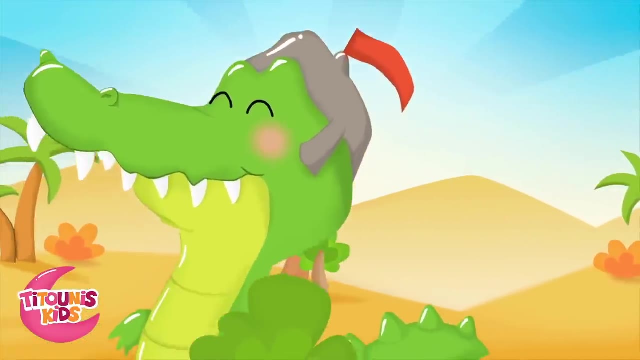 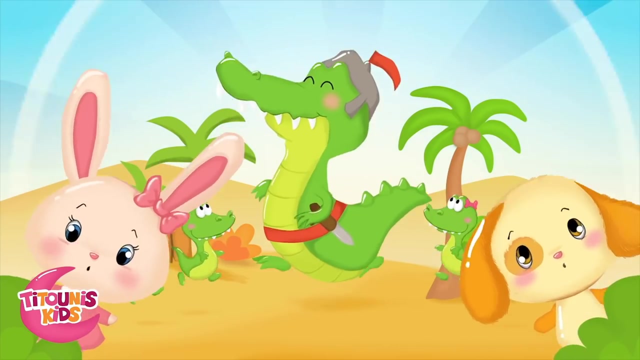 He said goodbye to all his family. Off through the dust, he marches with a fear Wagging his tail in search of elephants. Oh, the crow crow crow, the crow crow crow, The crocodiles are marching to the Nile To find an elephant. 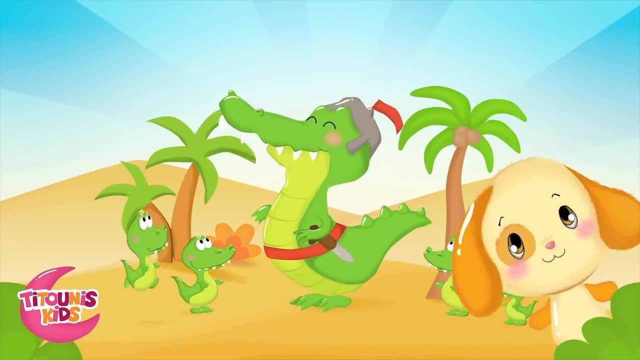 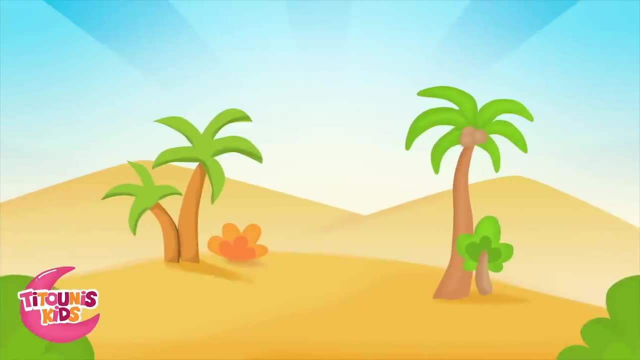 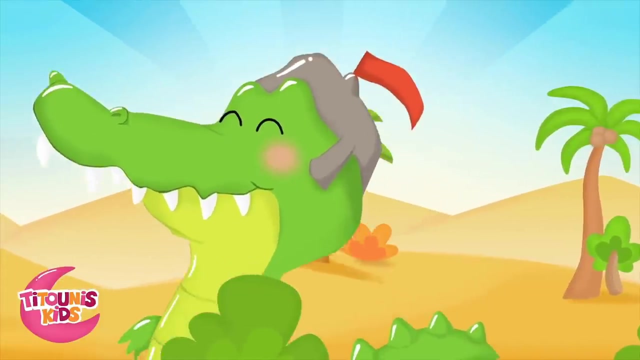 Oh, the crow crow crow, the crow crow crow. The crocodiles are marching to the Nile To find an elephant Whee. Walking Along, They sang their battle songs, Chomping the worms With lots of shiny teeth. If you could see. 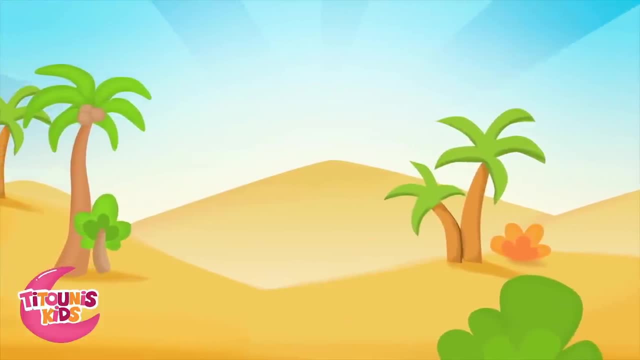 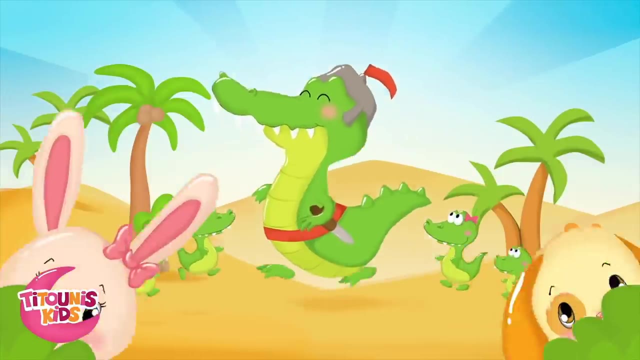 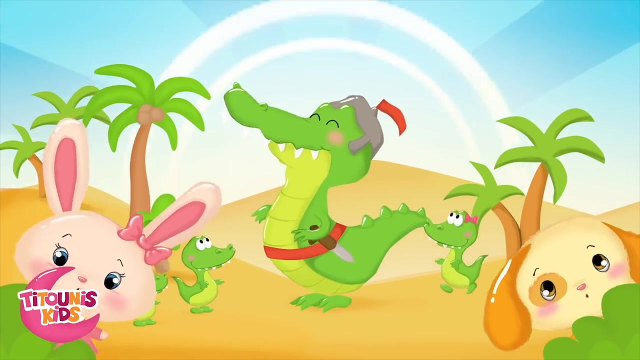 Them walking there so proudly, You wouldn't want To be their enemy. Oh, the crow crow crow, the crow crow crow. The crocodiles are marching to the Nile To find an elephant. Oh, the crow crow crow, the crow crow crow. 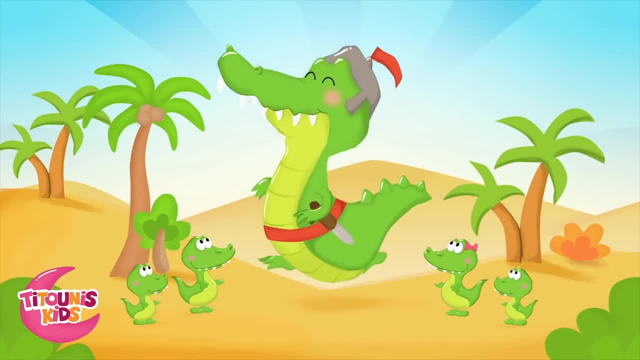 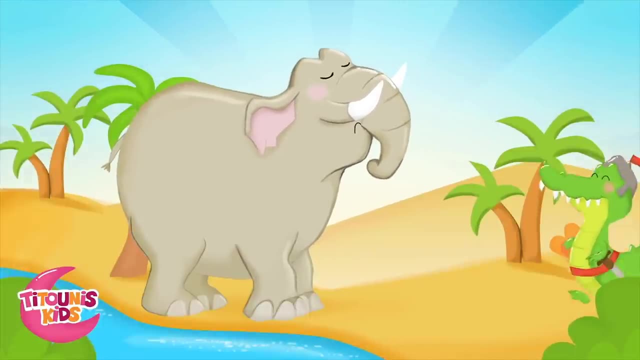 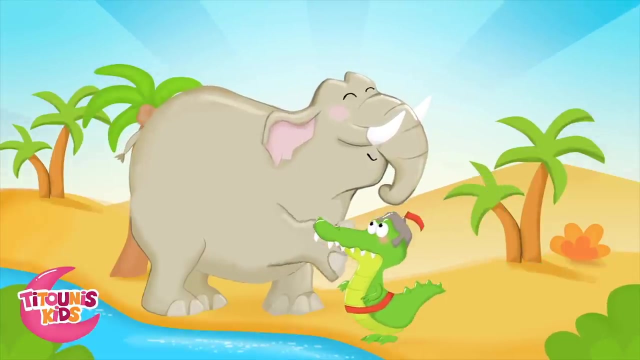 The crocodiles are marching to the Nile To find an elephant. Whoo, When they arrived, The elephants were waiting. This great battle is about to begin. Oh, crocodile, It's better to start running, Jumping to the river To have to swim away. Oh, the crow crow, crow, the crow, crow, crow, the crocodiles are. 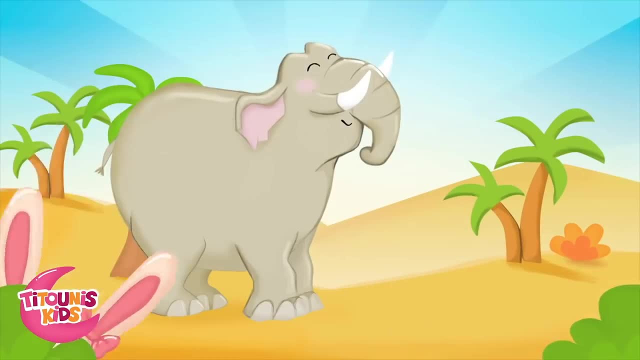 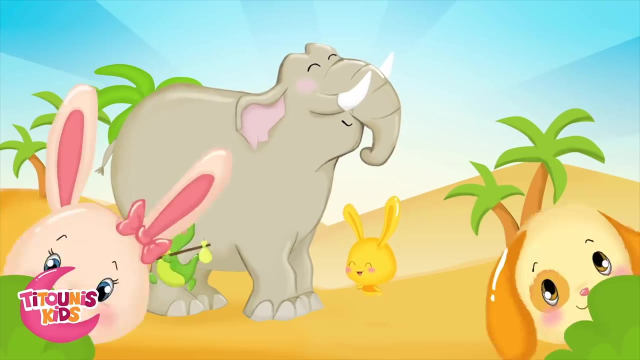 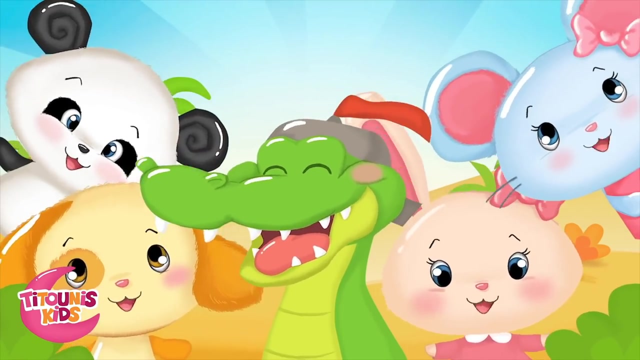 to find an elephant. Oh, the Cro Cro Cro, the Cro Cro Cro, the crocodiles are marching to the Nile to find an elephant. Oh, the Cro Cro Cro, the Cro Cro Cro, the crocodiles are marching to the Nile to find an elephant. 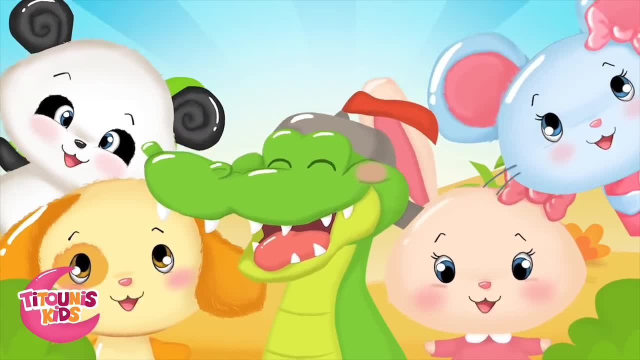 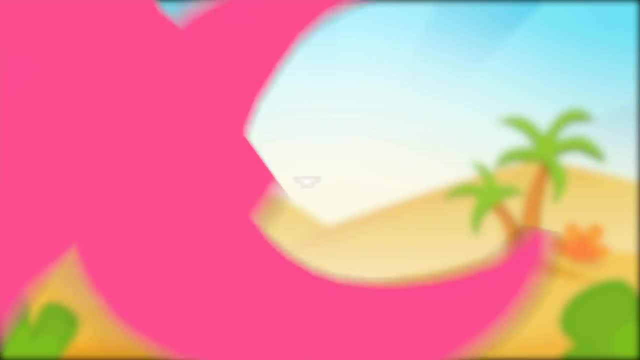 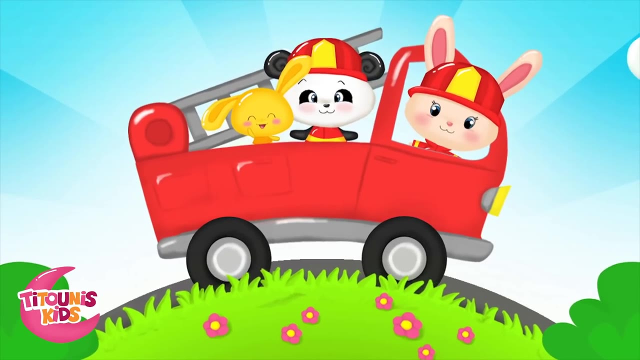 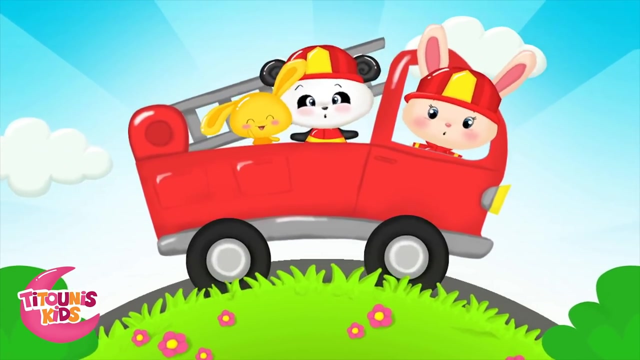 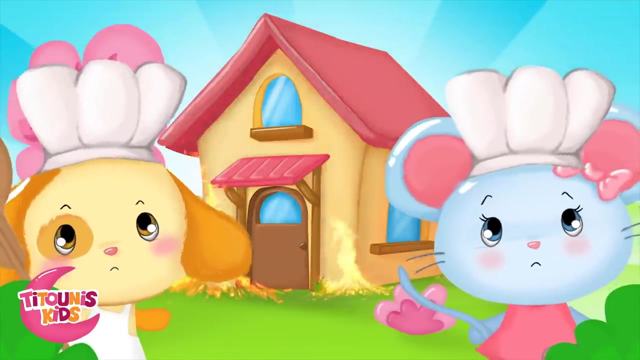 Oh, the Cro Cro Cro, the Cro Cro Cro, the crocodiles are Fire, fire, firemen, fire Quick, the house is burning. Fire, fire, firemen, fire. The house just burned down. It's not me who burnt it down, I'm sure it's Miss Chef. 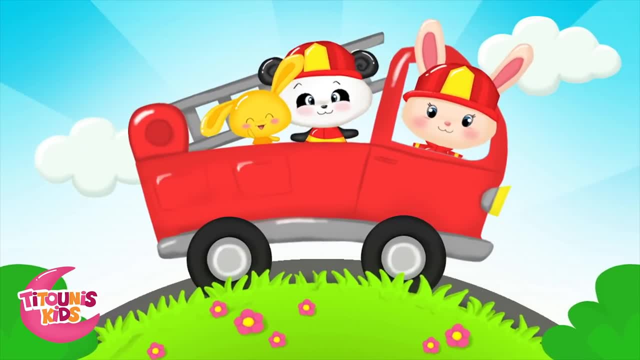 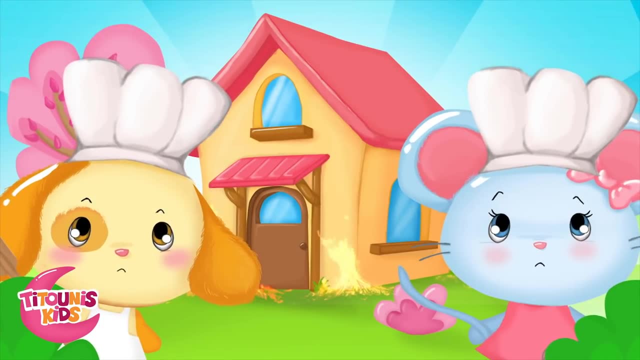 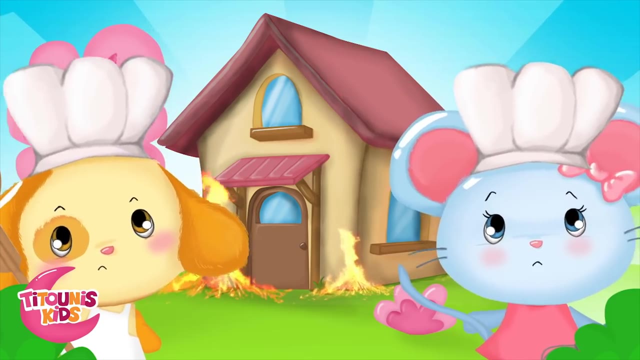 Fire, fire, fireman fire, Quick, the house is burning. Fire fire, fireman fire, The house just burned down. It's not me who burnt it down, I'm sure it's Mr Chef. Fire fire, fireman fire, Quick, the house is burning. 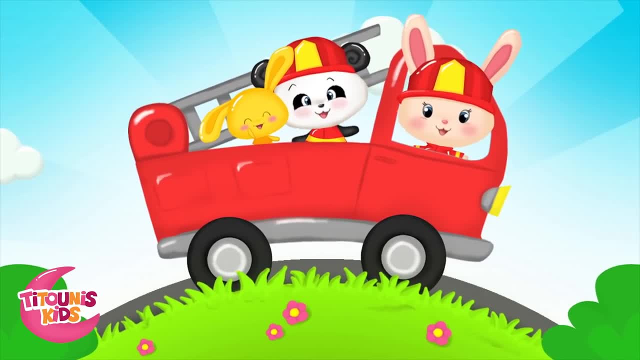 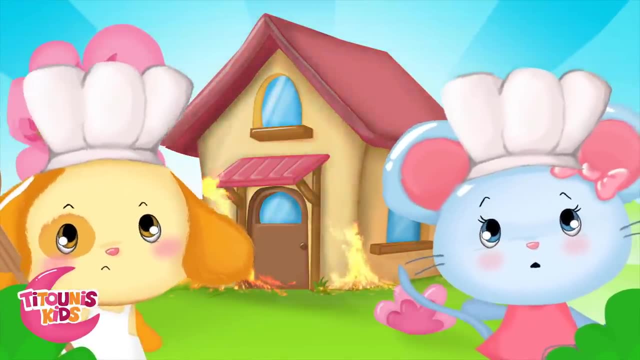 Fire, fire, fireman fire. The house just burned down. It's not me who burnt it down, I'm sure it's Mr Chef. It's not me who burnt it down, I'm sure it's Mr Chef. 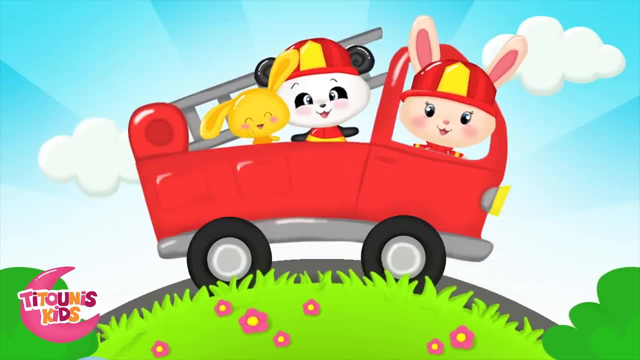 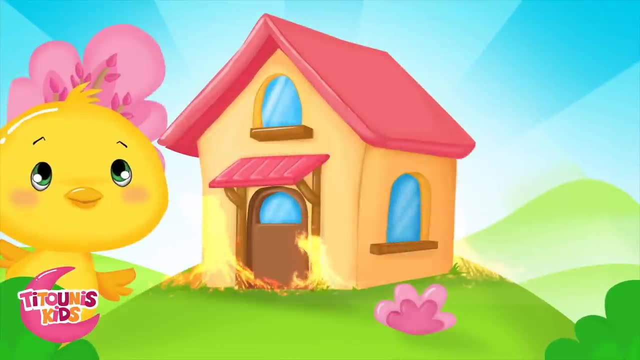 Fire, Fire, fire, fireman fire. Quick, the house is burning Fire, fire, fireman fire. The house just burned down. It's not me who burnt it down. I'm sure it's Little Teeny. 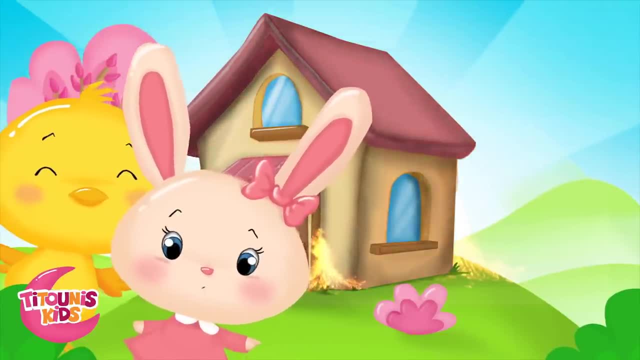 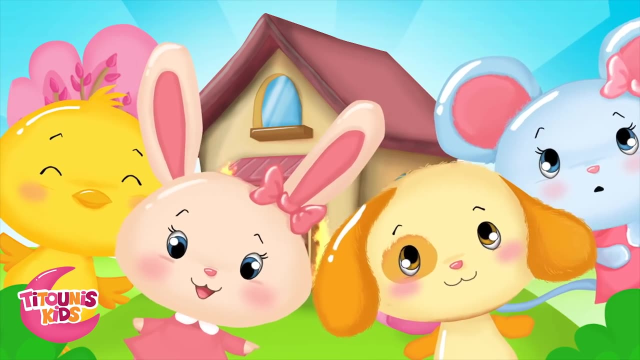 It's not me who burnt it down. I'm sure it's Little Boo. It's not me who burnt it down. I'm sure it's Little May. It's not me who burnt it down, I'm sure it's Little Toony. 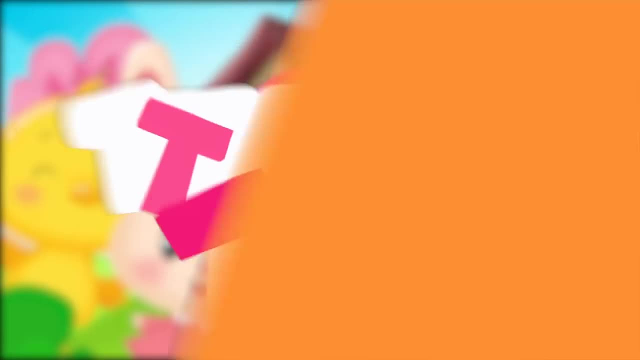 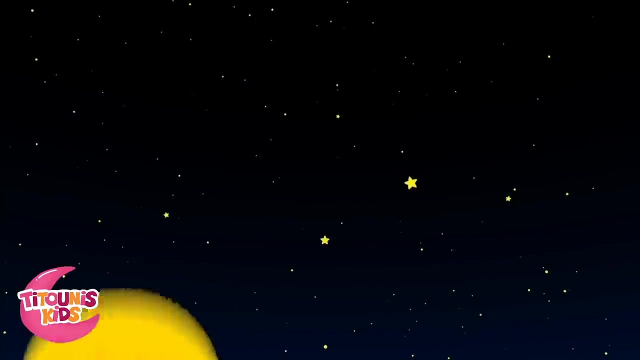 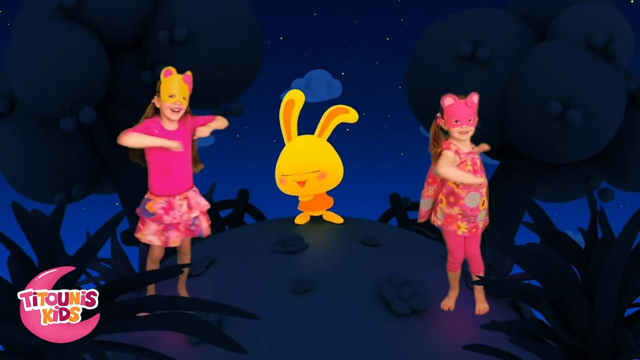 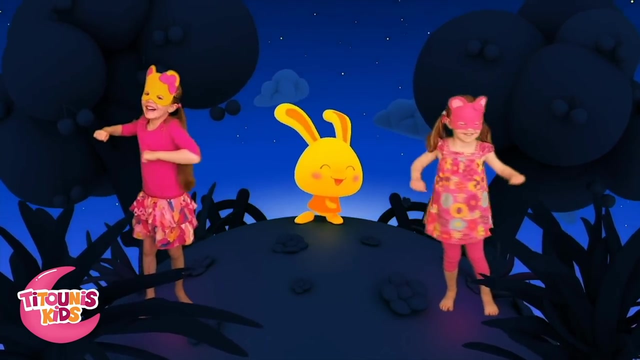 Oops, It's not me who burnt it down. It's not me who burnt it down. I'm sure it's Little Toony. Everybody up. it's that time. Everybody up. this is fine. Let's dance and jump all day long. 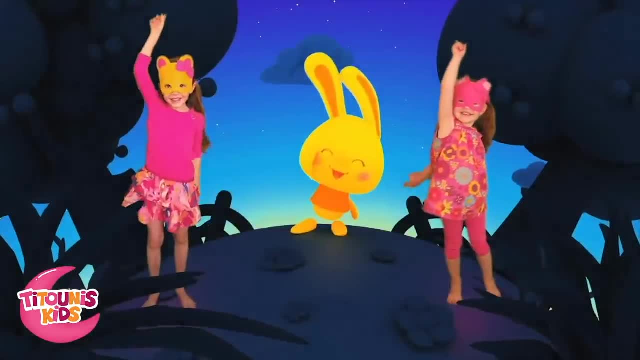 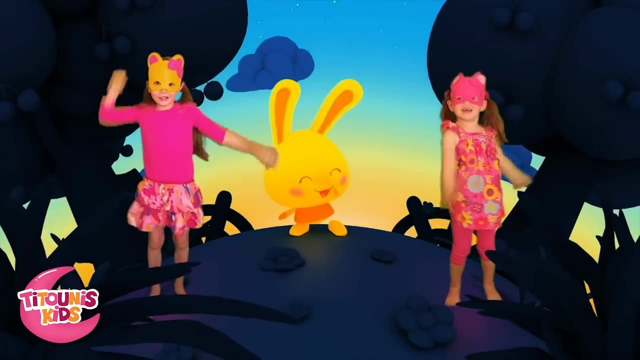 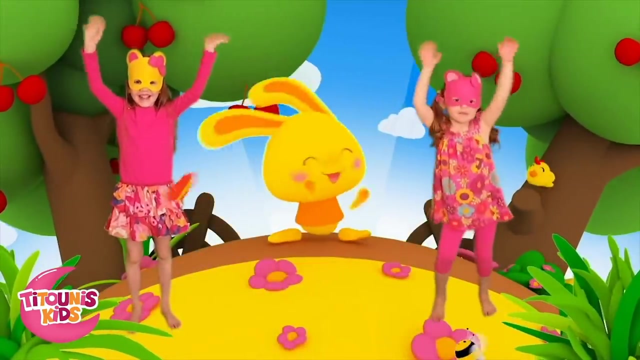 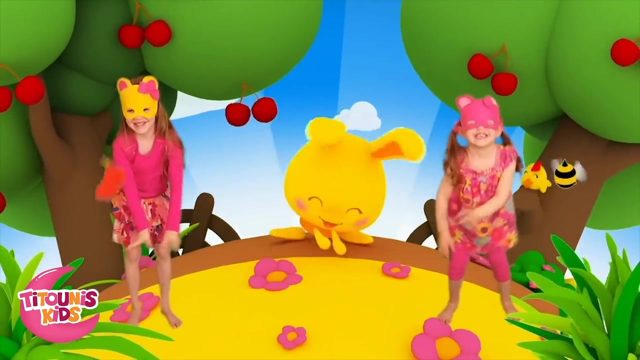 Ha, ha, ha ha. have some fun. This is a song. What is this song? What is this song? the kids, but parents also, like the peeps. We jump, swing, move and sing. Come, come, come, come, come with me, Join the party, come here, We dance with Melly and Toonie. Everybody dance like this. 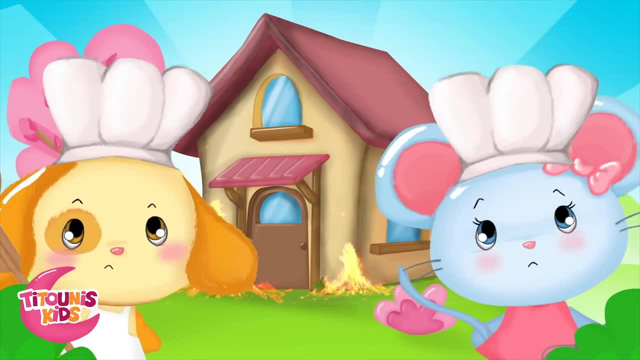 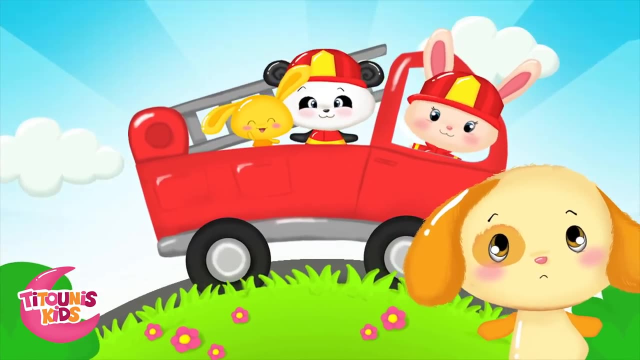 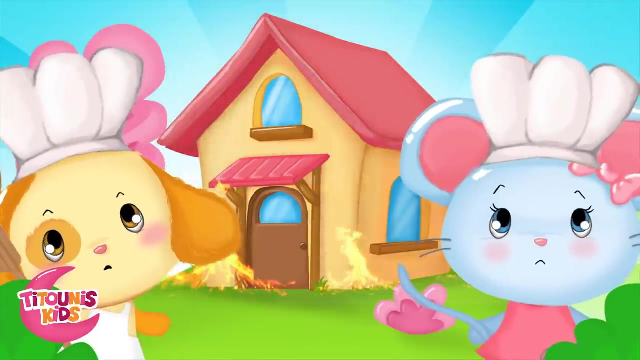 It's not me who burnt it down, Sure, it's Mr Chef, Fire, fire, firemen fire. Quick, the house is burning Fire, fire, firemen fire. The house just burned down. It's not me who burnt it down, I'm sure it's Miss Chef. 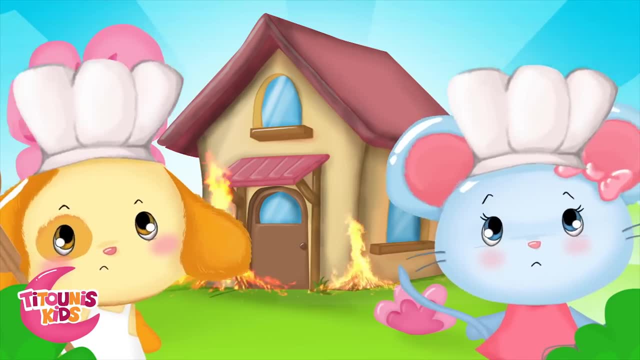 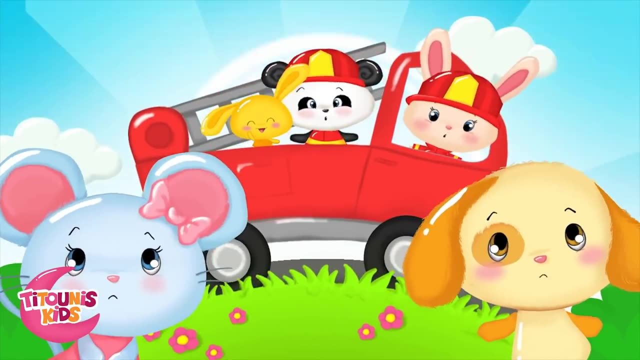 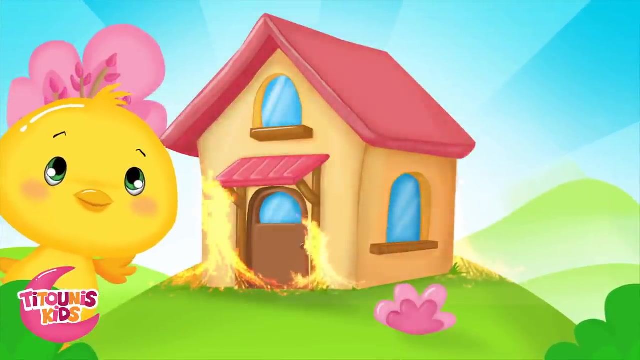 It's not me who burnt it down, Sure, it's Mr Chef, Fire fire, firemen fire. Quick, the house is burning Fire, fire, fireman fire. The house just burned down. It's not me who burnt it down, Sure, it's Little Teenie. 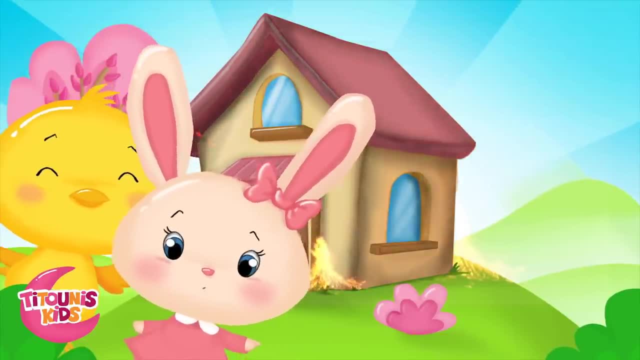 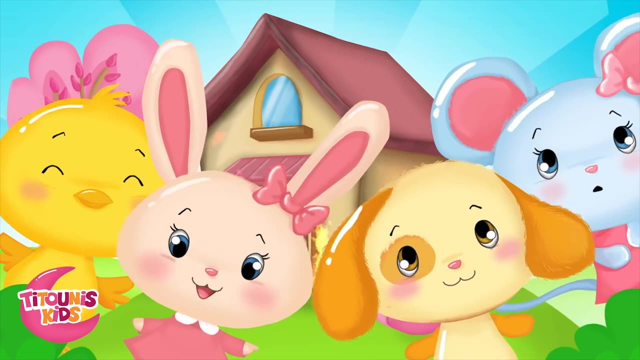 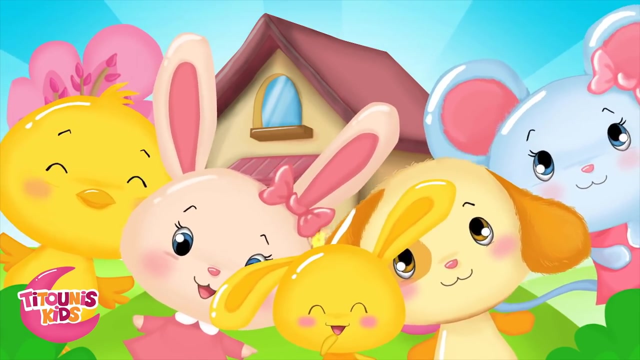 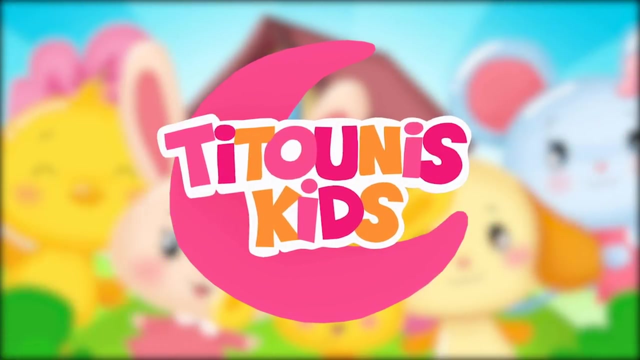 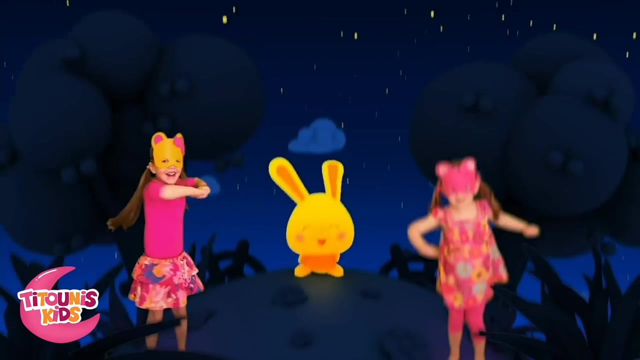 It's not me who burnt it down, Sure, it's Little Boo. It's not me who burnt it down, Sure, it's Little May. It's not me who burnt it down, Sure, it's Little Toonie. Oops, Everybody up. it's the time, Everybody up. this is fine. 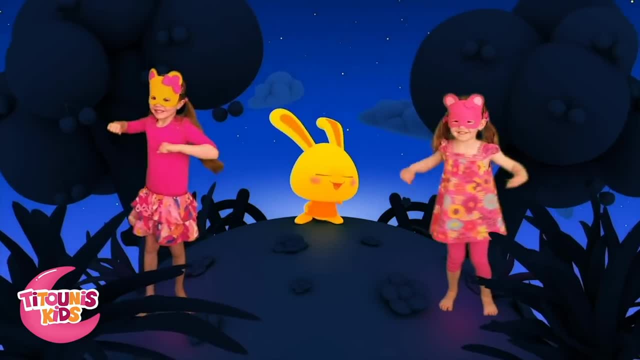 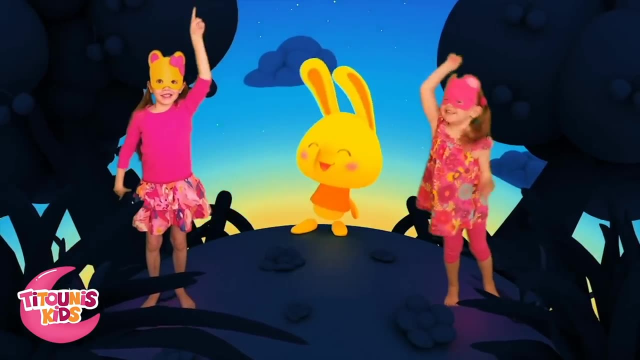 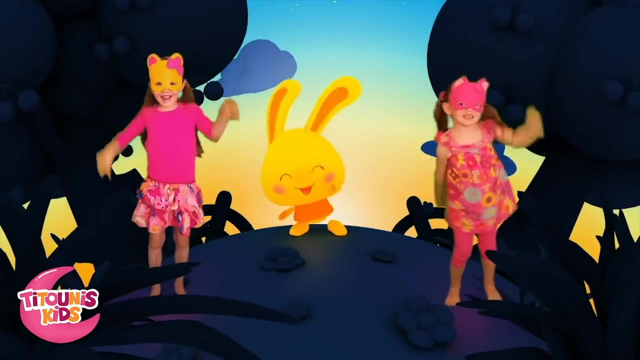 Let's dance and jump all day long. Ha ha, ha ha. have some fun. This is a song by the kids, But parents also like the beeps. We jump, swing, move and sing Ka-ka-ka-ka-ka, come with me. 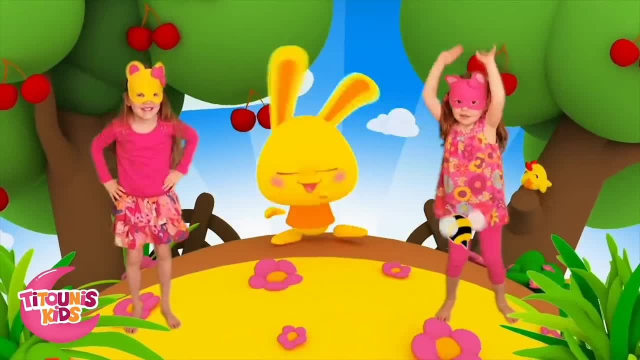 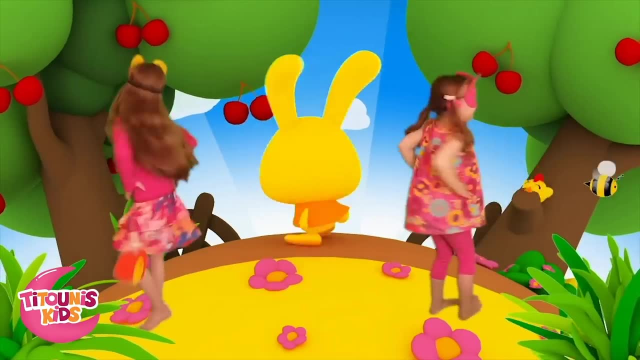 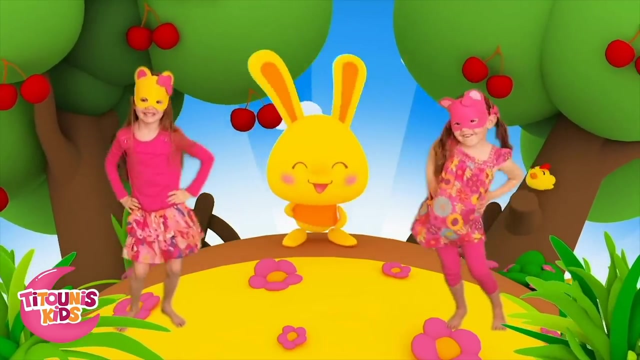 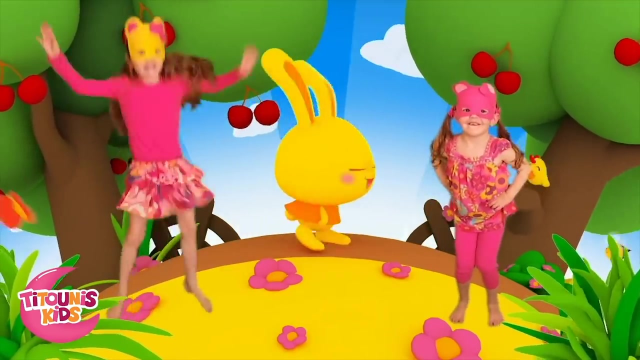 Join the party. come here, We dance with Manny and Toonie. Everybody dance like this. The Dance, Dance, Dance from Toonie. Join the party. come here, We dance with Manny and Toonie. Everybody dance like this. The Dance, Dance, Dance from Toonie. 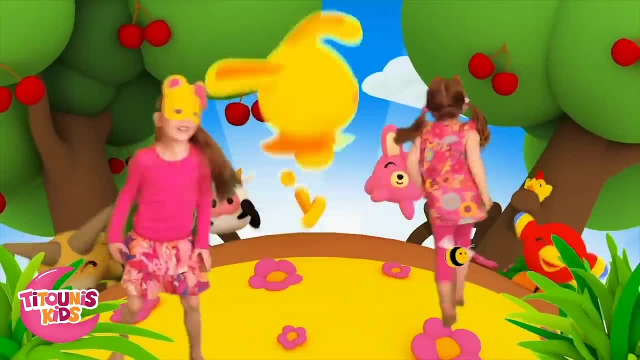 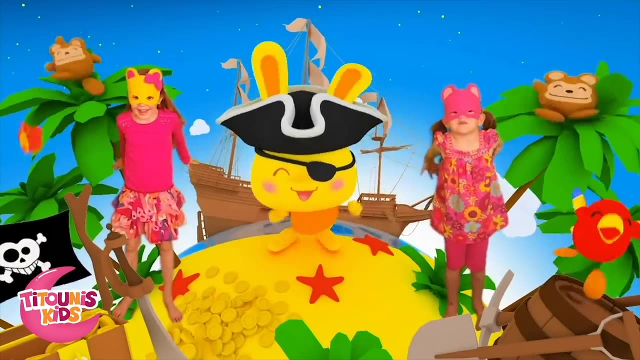 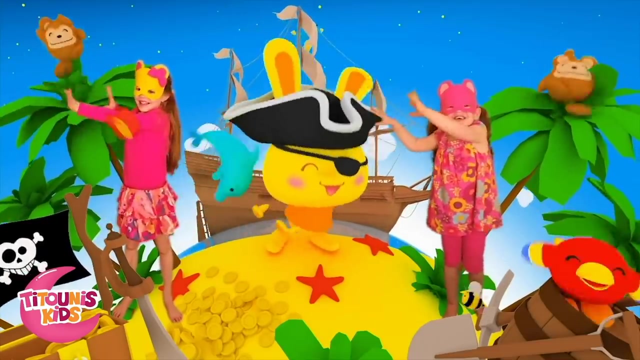 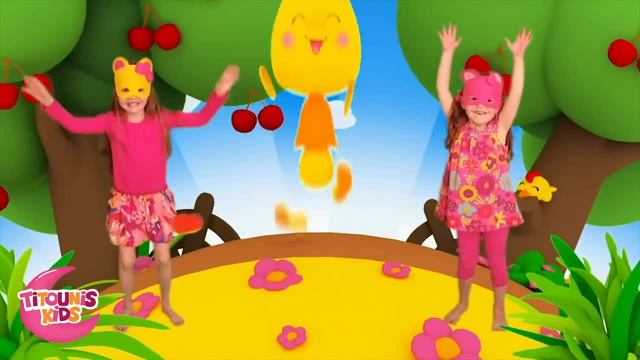 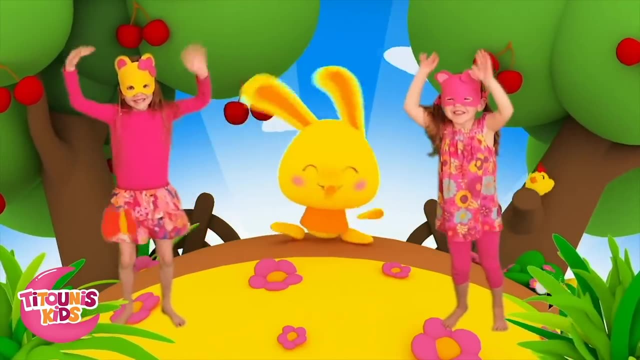 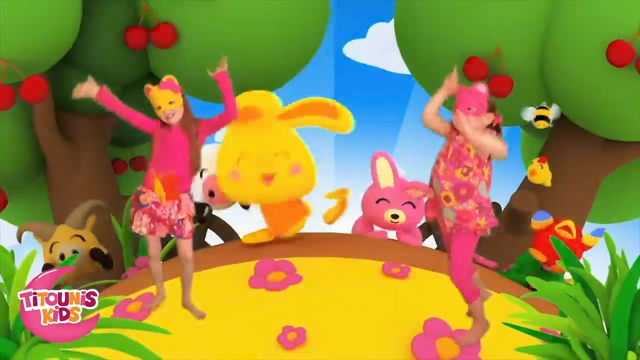 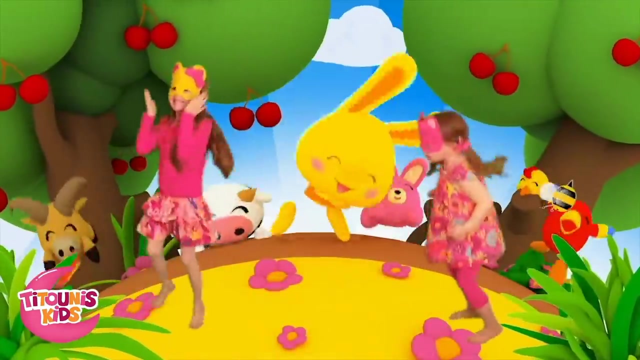 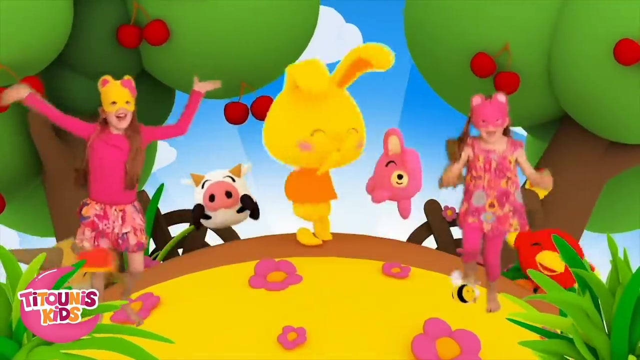 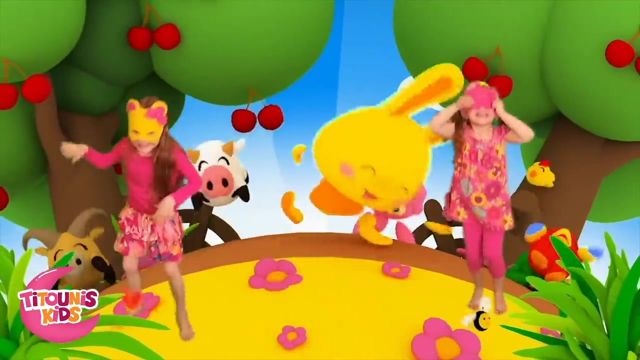 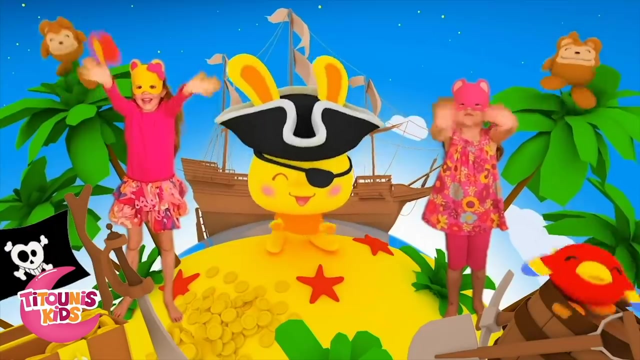 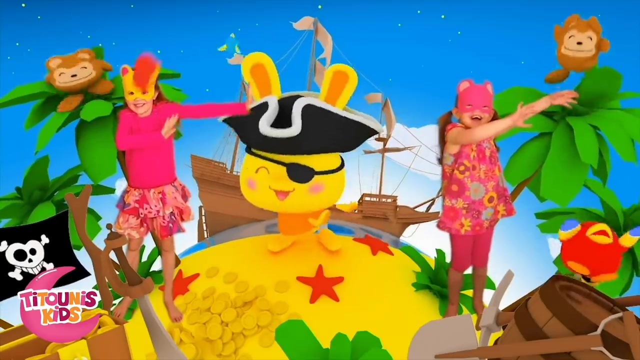 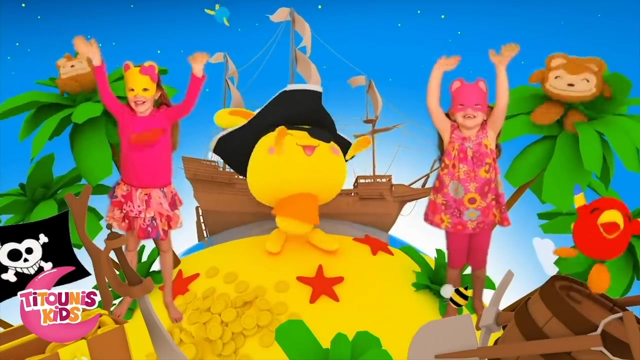 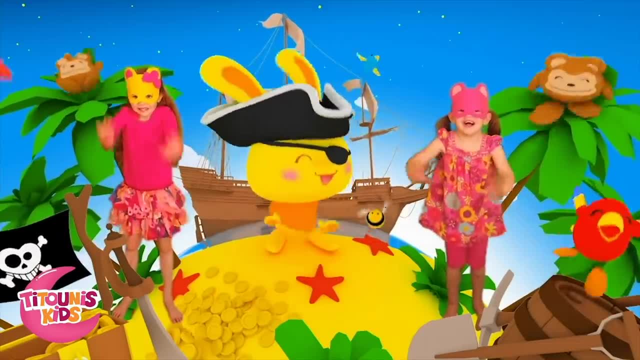 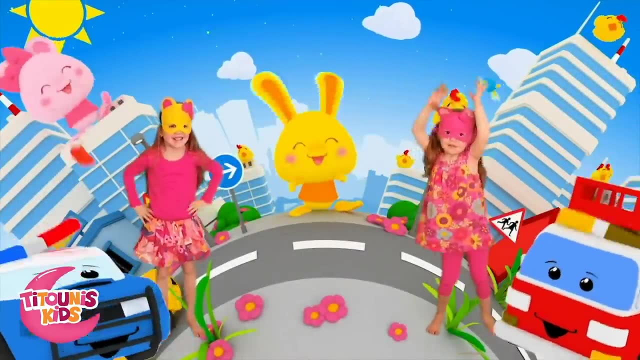 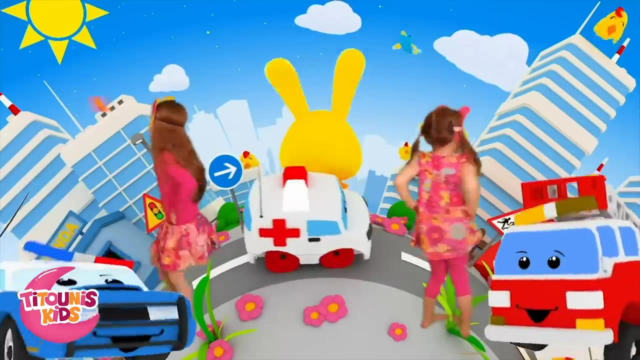 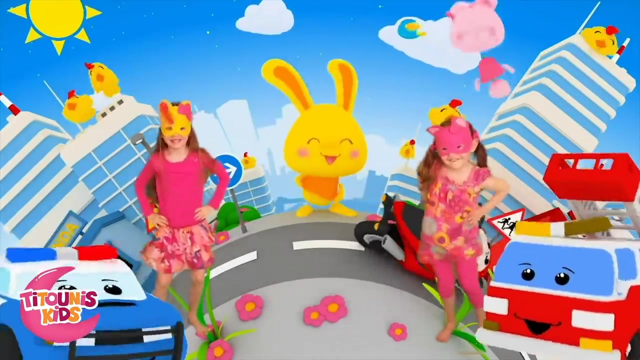 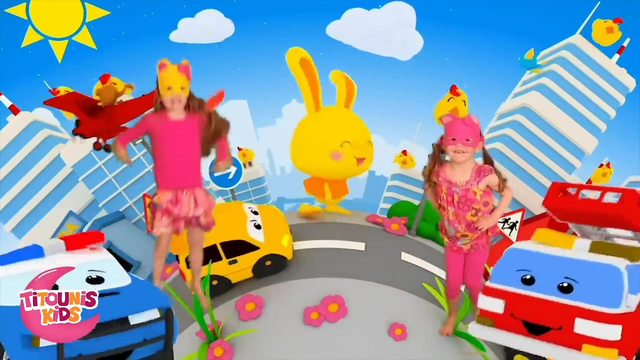 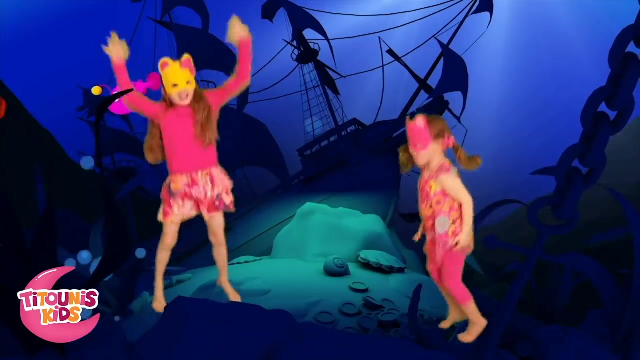 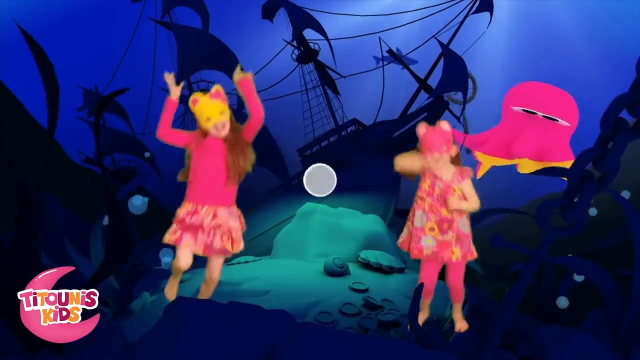 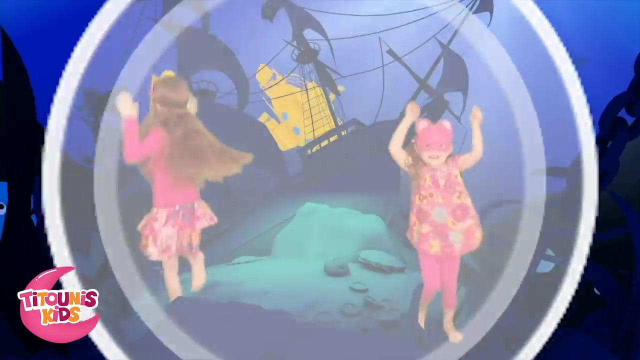 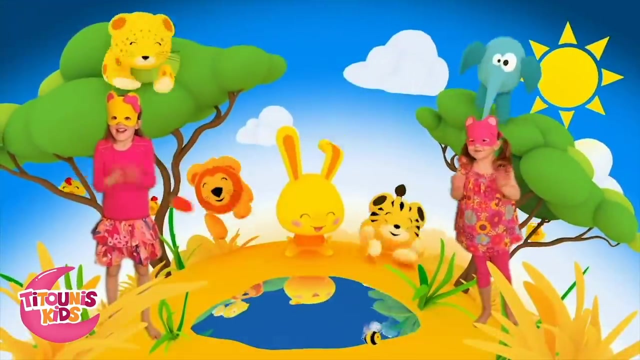 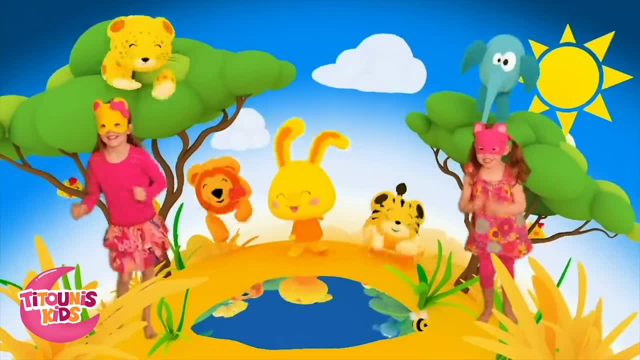 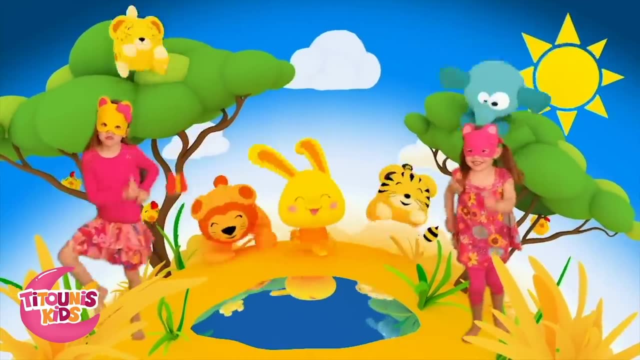 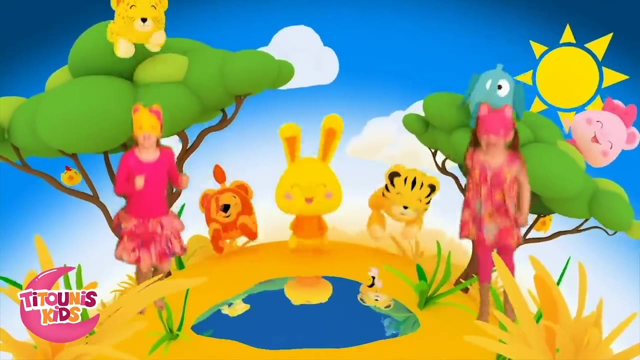 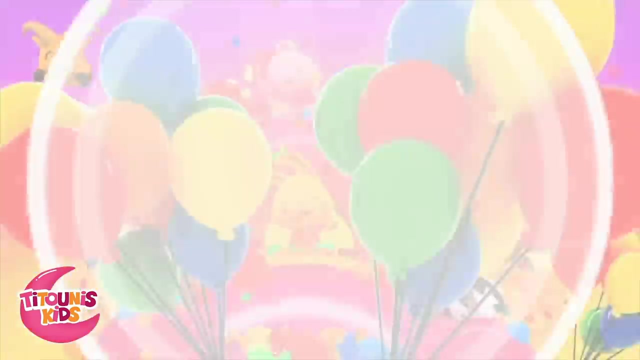 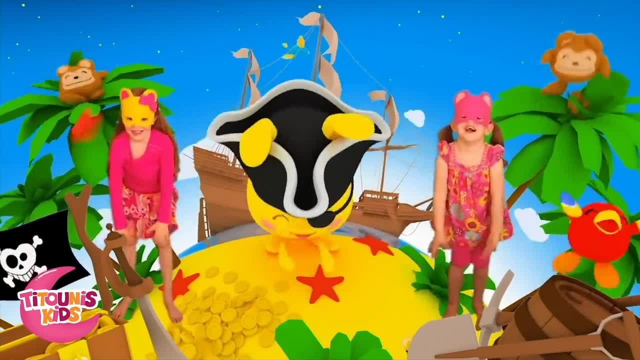 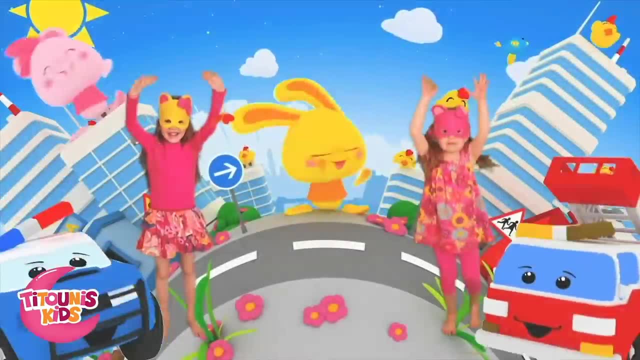 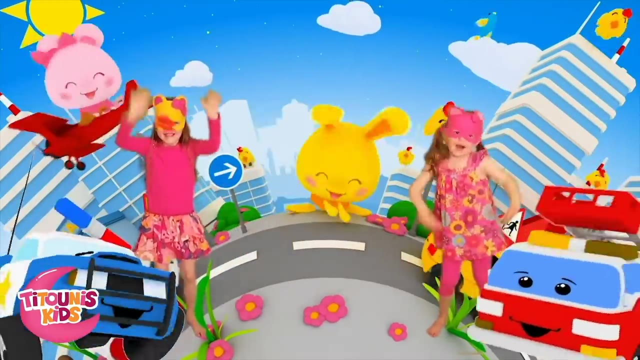 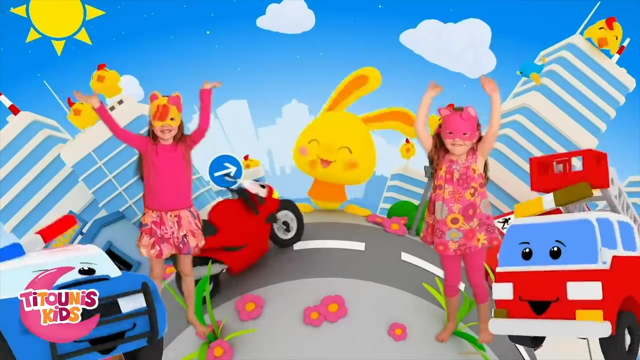 Move the hands where To the floor, Move the hands where To the middle. Dance, dance, dance and never stop. Join the party, come here. We dance with Manny and Toonie. Everybody dance like this. The Dance, Dance, Dance from Toonie. Join the party, come here. 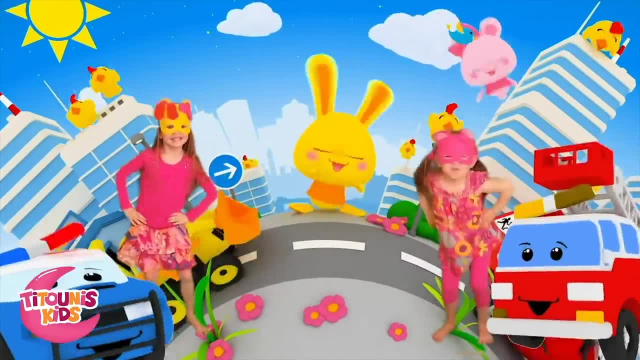 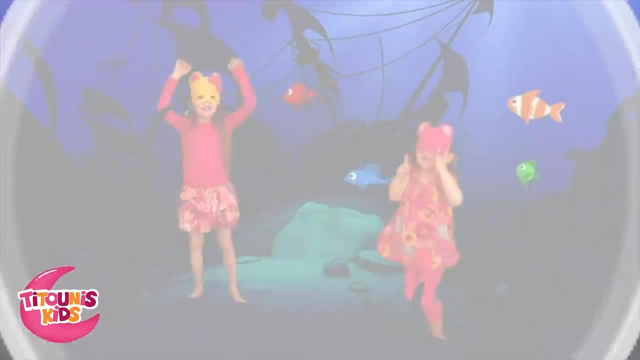 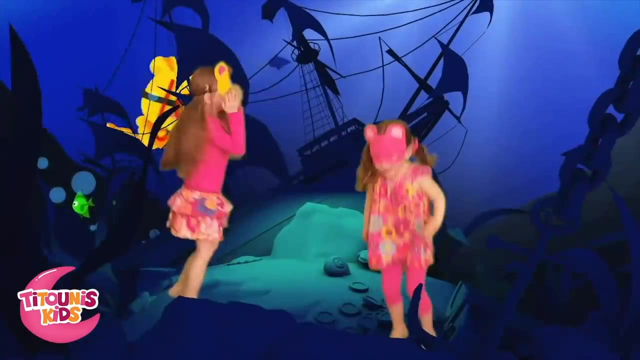 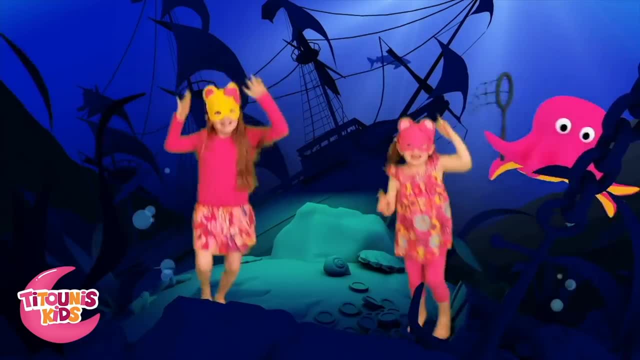 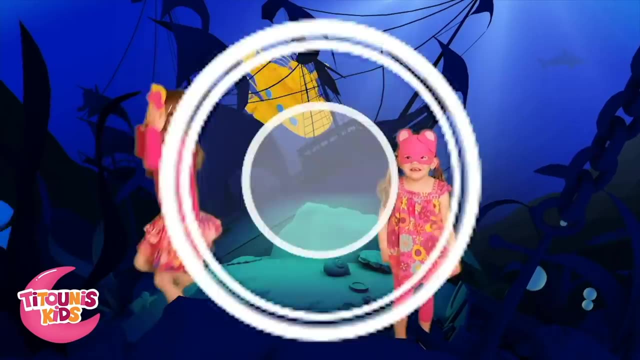 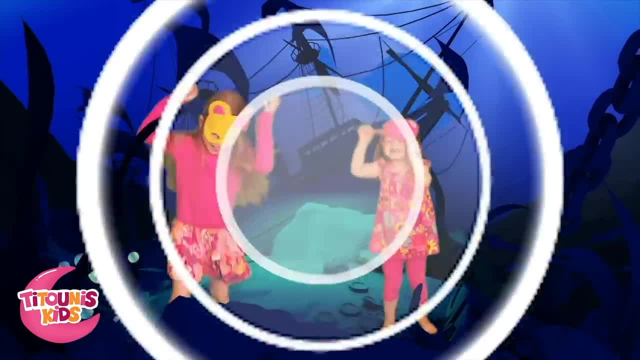 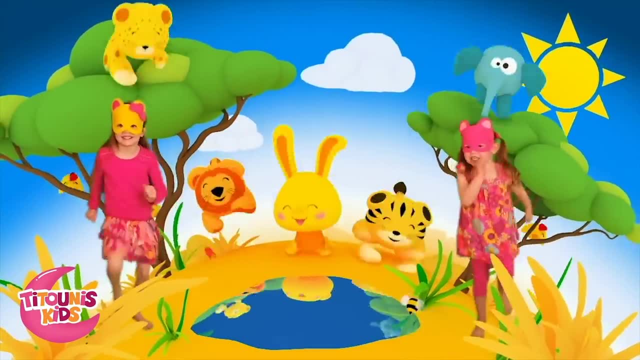 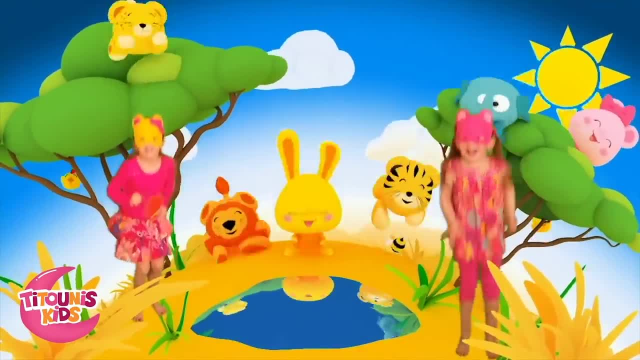 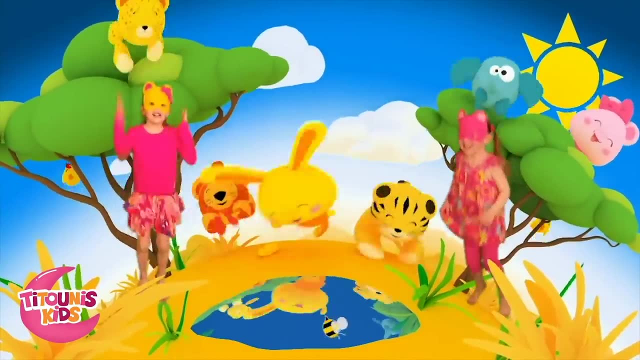 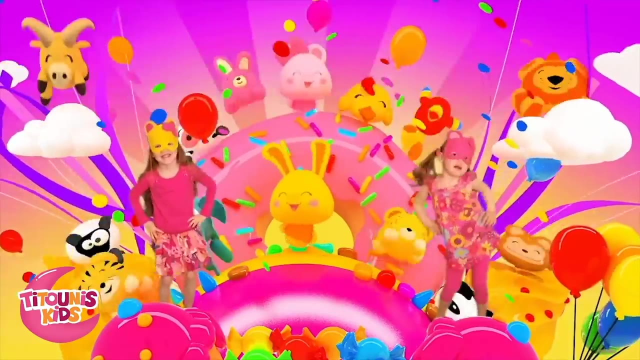 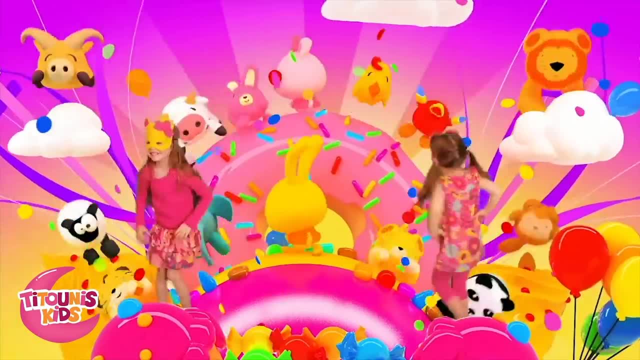 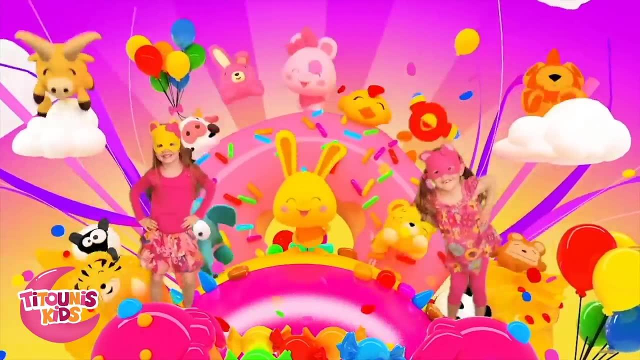 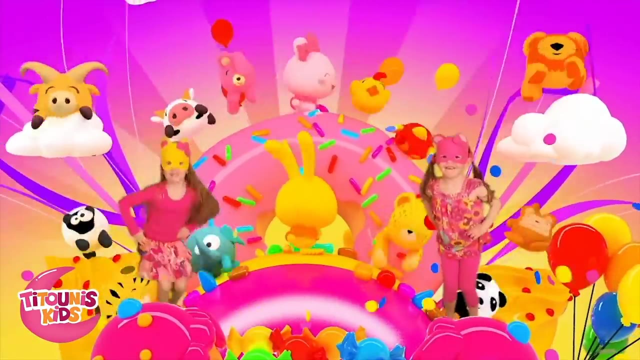 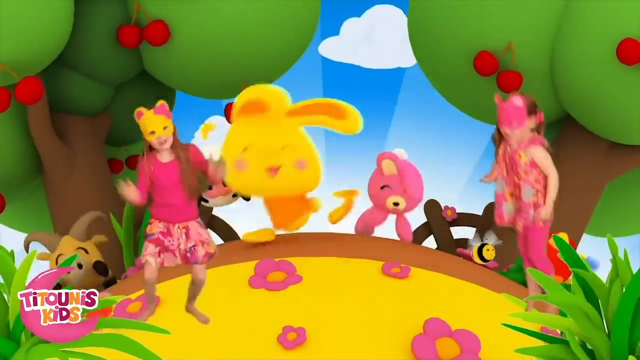 Everybody dance like this. The dance, dance, dance Something to me. Join the party. come here, We dance with Ellie and Jimmy. Everybody dance like this. The dance, dance, dance Something to me. La-la-la-la, la-la-la-la, La-la-la-la, la-la-la-la. 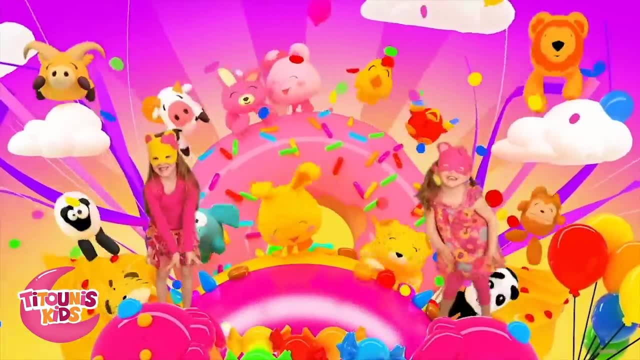 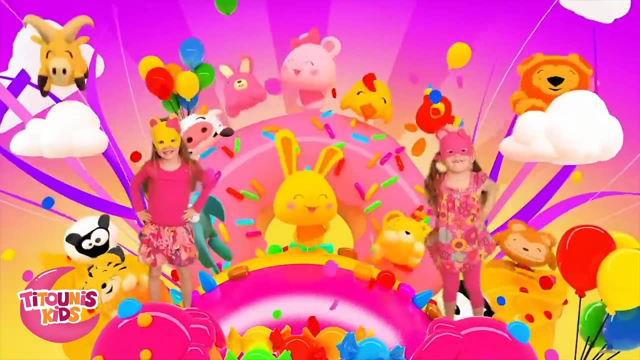 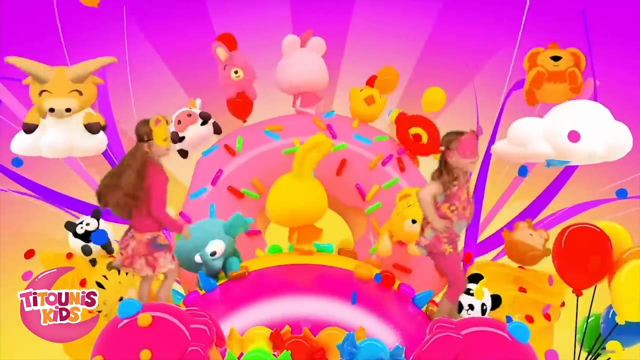 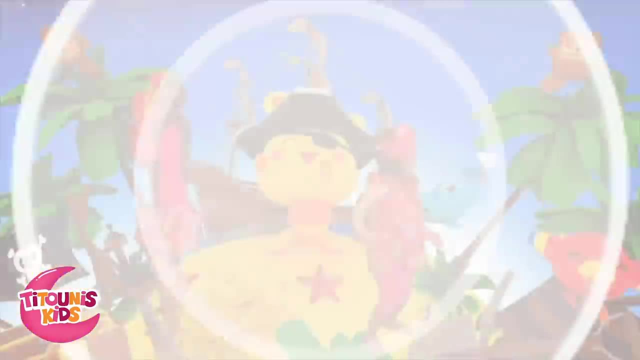 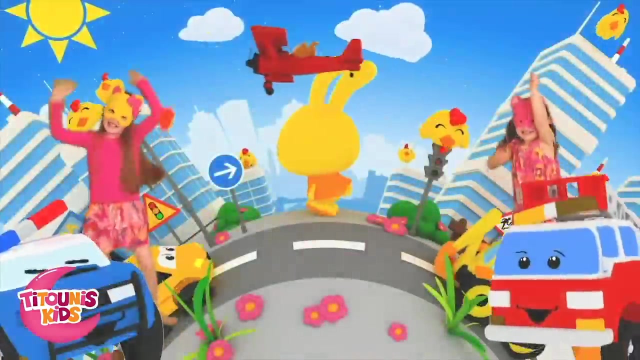 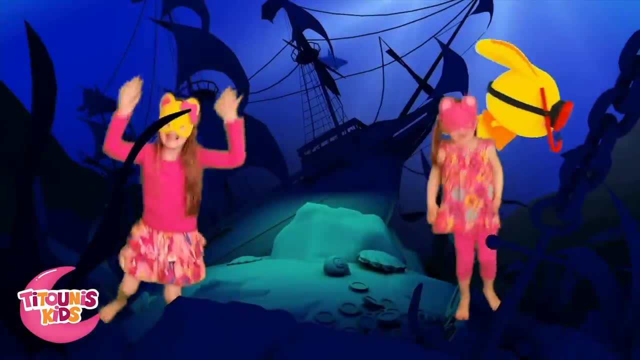 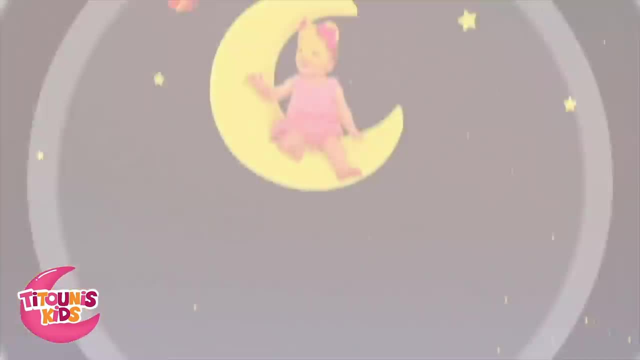 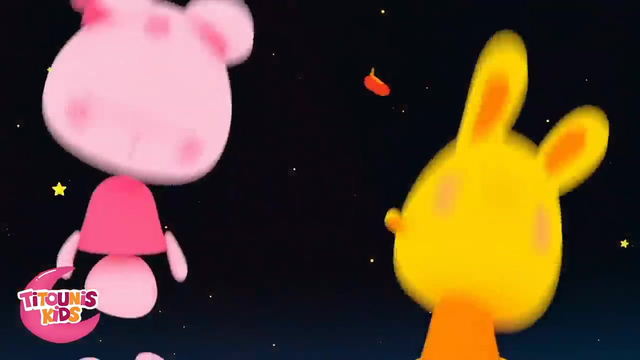 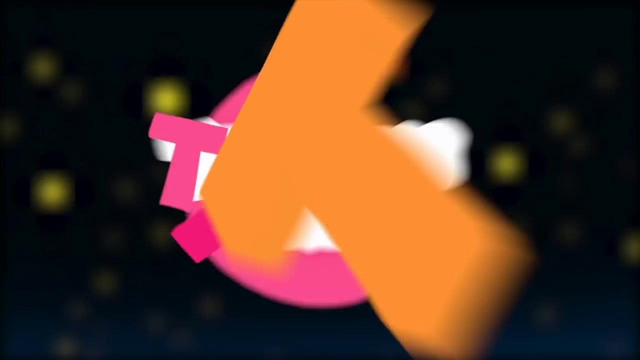 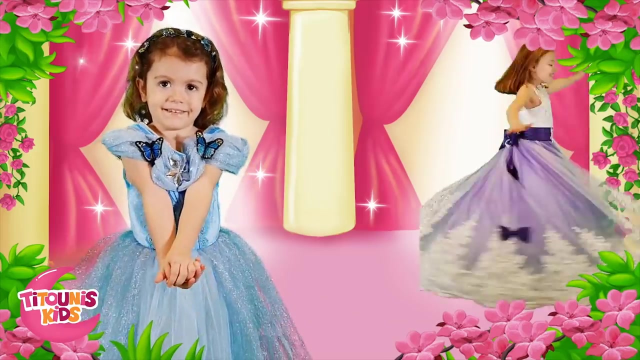 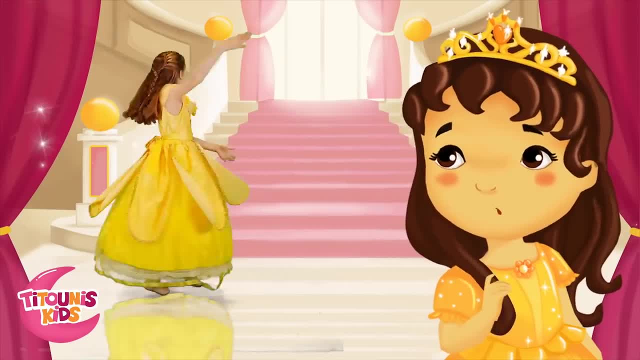 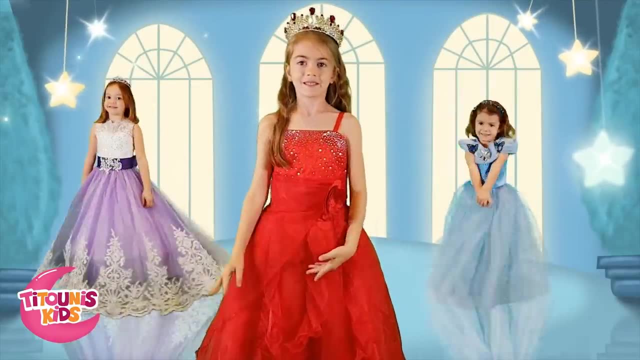 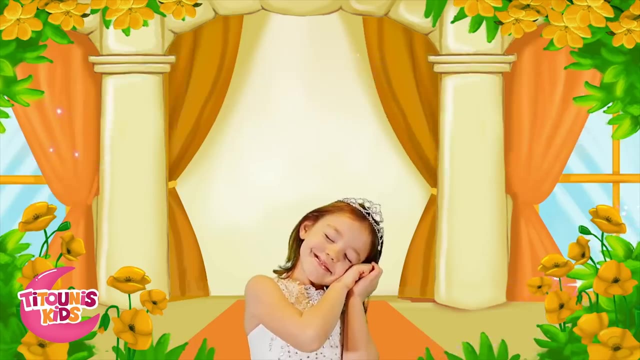 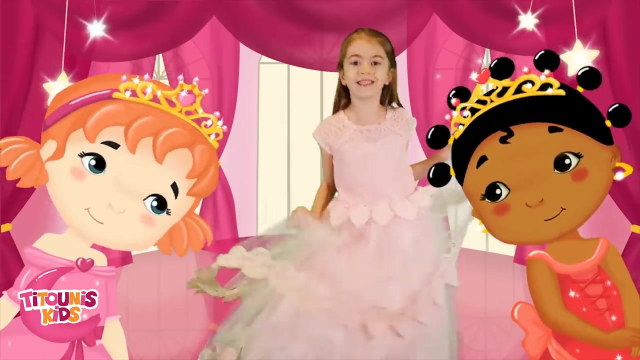 In the magical world, everything is beautiful. Oh princesses, dance, dance, dance. Oh princesses, come on, take a bow. With your imagination And a little magic, of course, A princess, you can be The best princess of them all. Oh princesses, dance, dance, dance. 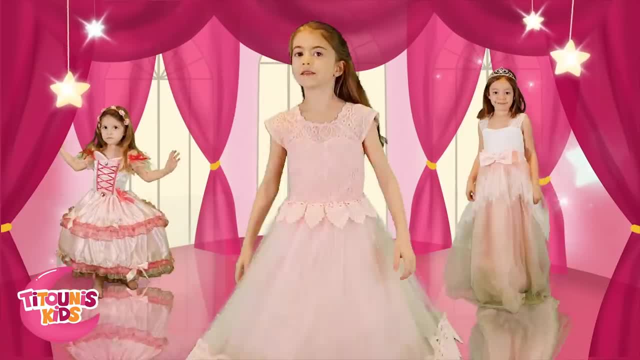 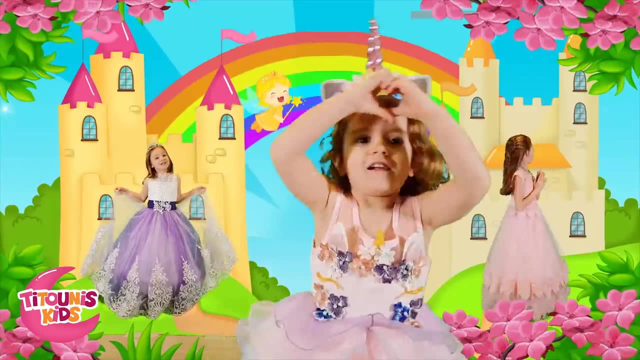 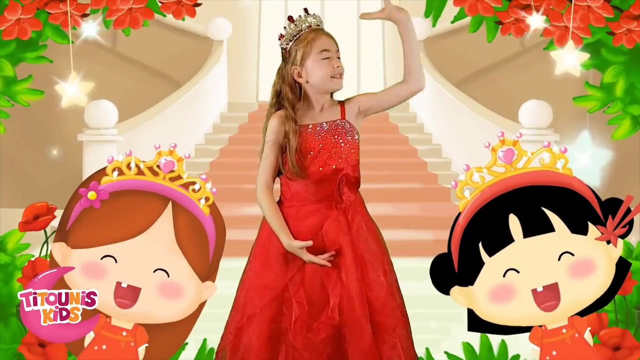 Oh princesses, come on, take a bow. Picture a giant castle. You can live there all the time With your friends. you will be, And you'll have so much fun. Oh princesses, dance, dance, dance. Oh princesses, come on, take a bow. 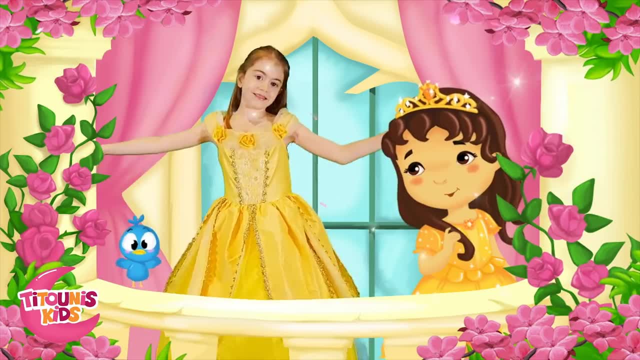 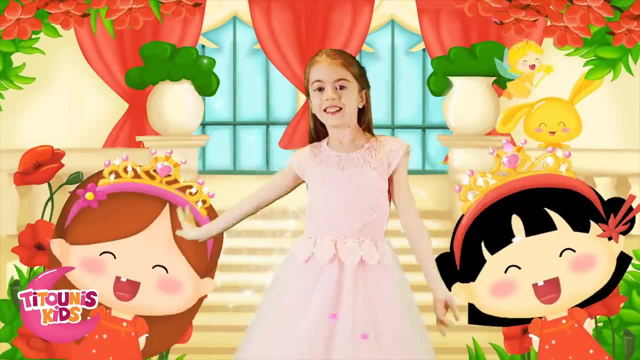 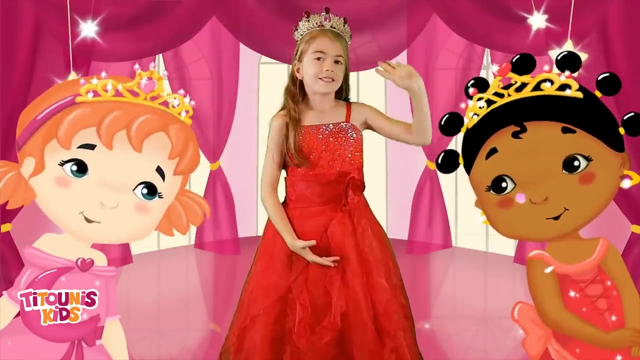 In the princesses' world, Everything is fine and cool. If you want to come along, What are you waiting for? What are you waiting for? Take my hand and come with me. Oh princesses, dance, dance, dance. Oh princesses, come on, take a bow. 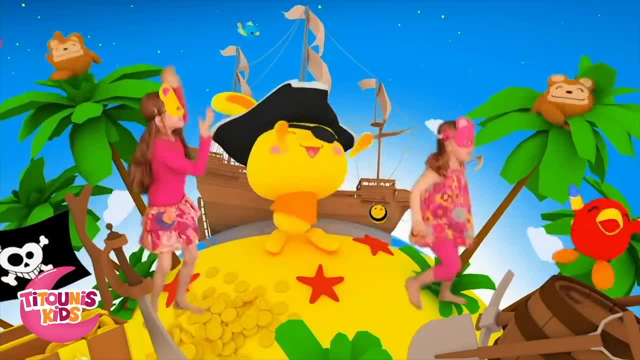 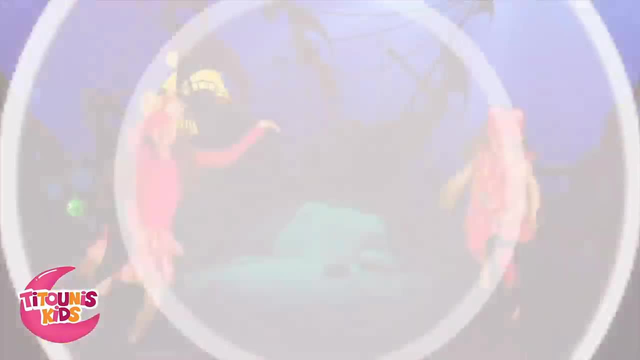 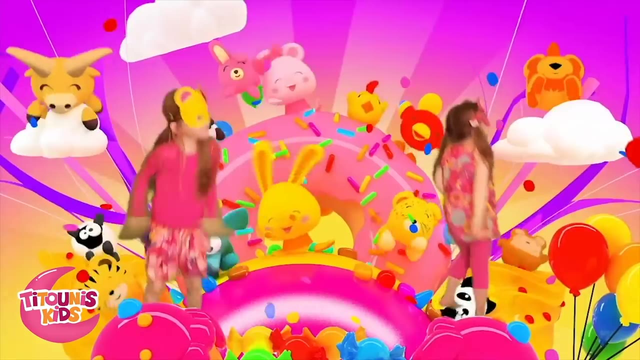 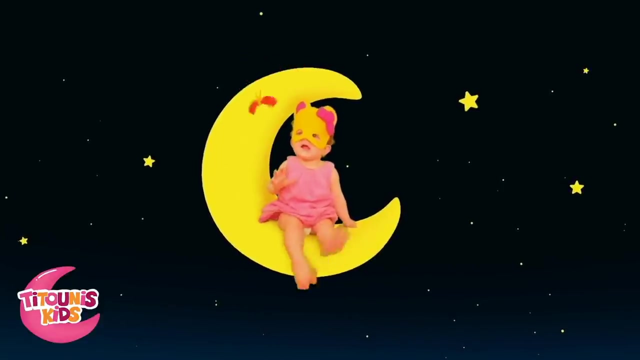 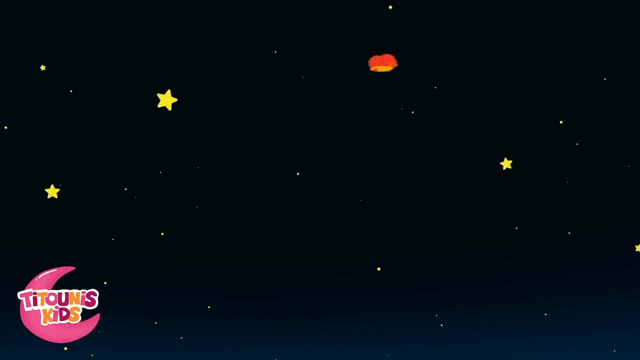 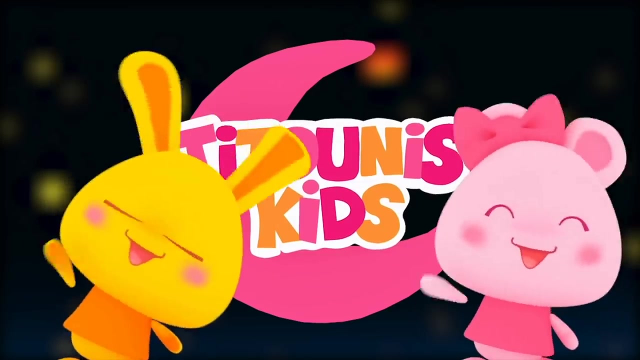 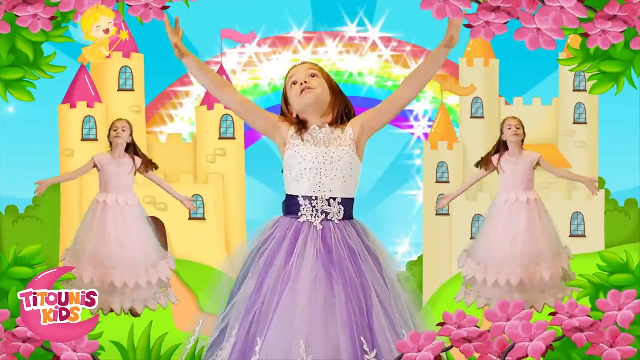 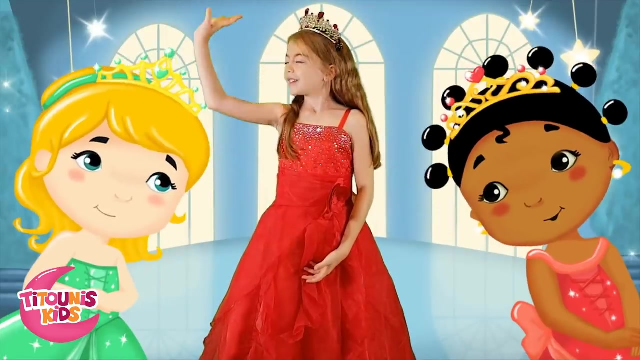 La-la-la-la, la-la-la-la, La-la-la-la, la-la-la-la, La, la, la, la, la. Stop. It's the magical world of the princesses, of course, In the magical world, everything is beautiful. Oh, princesses, dance, dance, dance. 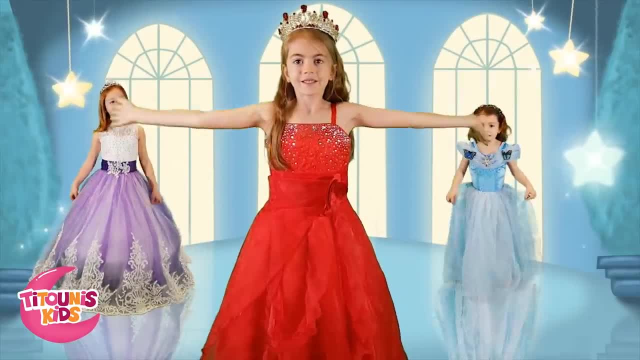 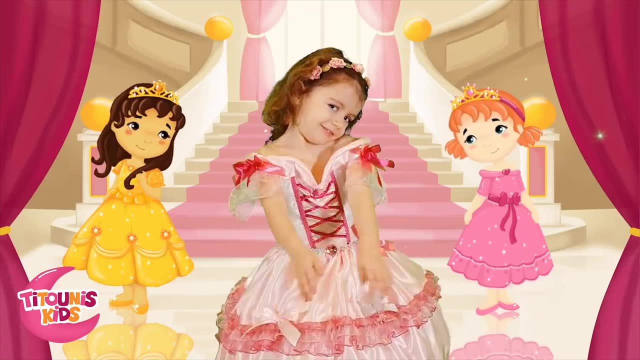 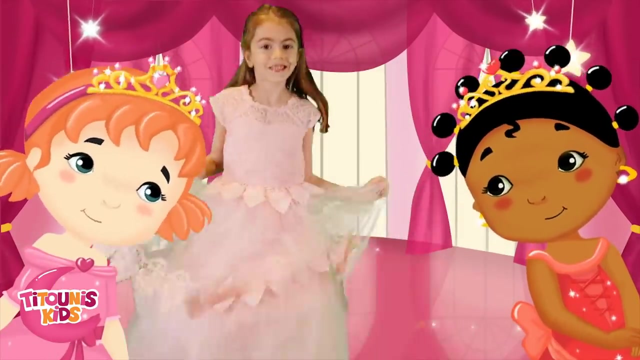 Oh, princesses, come on, take a bow With your imagination and a little magic. of course, It's the magical world of the princesses. of course, A princess, you can be the best princess of them all. Oh, princesses, dance, dance, dance. 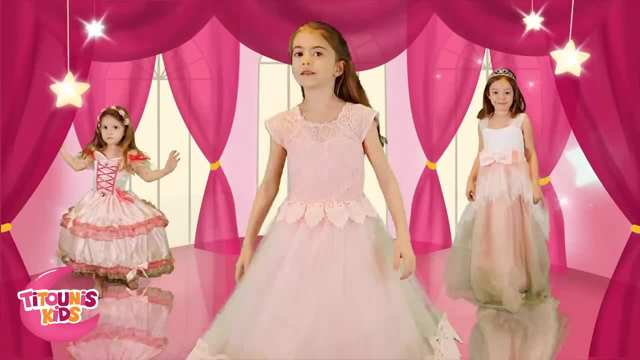 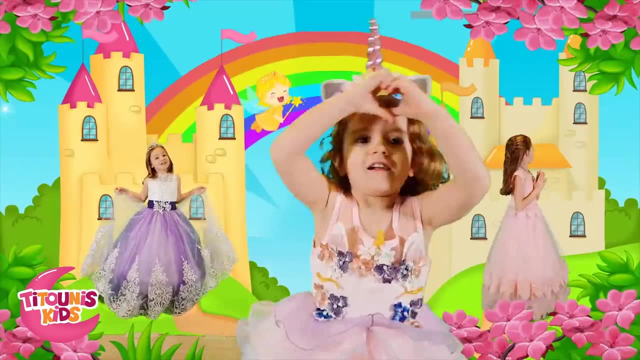 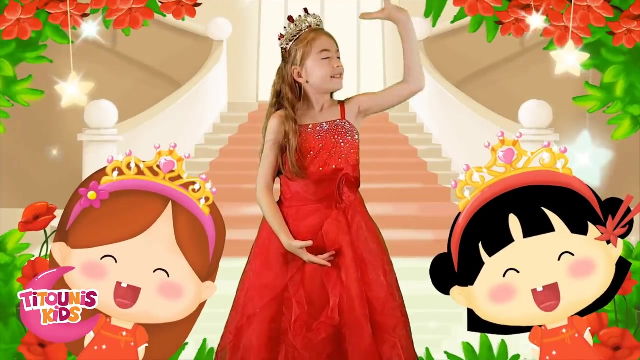 Oh princesses, come on, take a bow. Picture a giant castle. you can live there all the time With your friends. you will be and you'll have so much fun. Oh princesses, dance, dance, dance. Oh princesses, come on, take a bow. 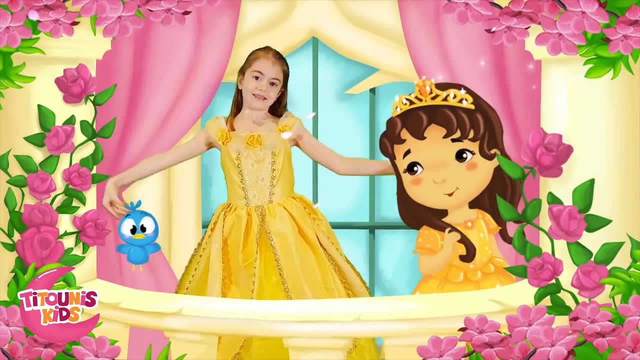 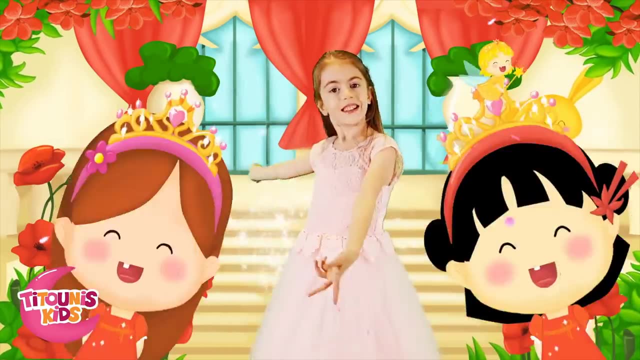 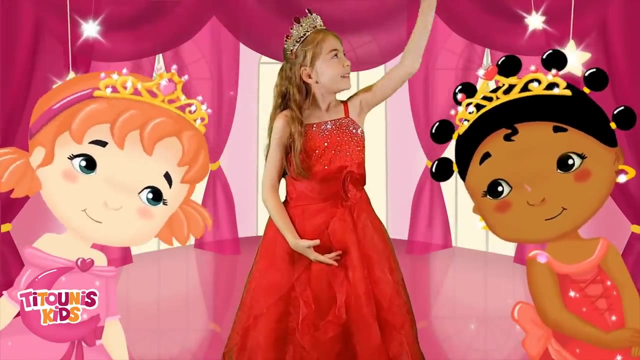 In the princesses' world, everything is fine and cool. If you want to come along, what are you waiting for? What are you waiting for? Take my hand and come with me. Oh princesses, dance, dance, dance. Oh princesses, come on, take a bow. 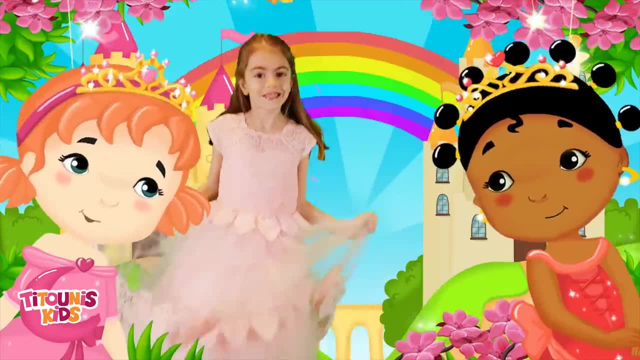 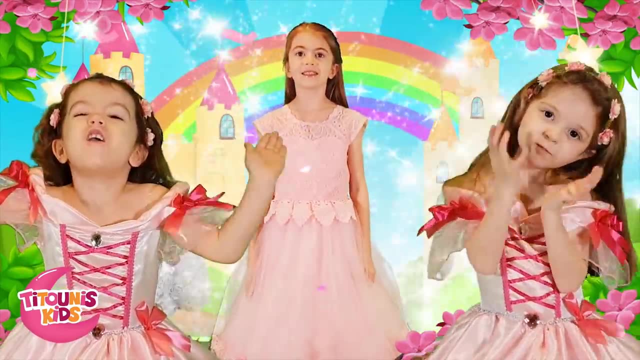 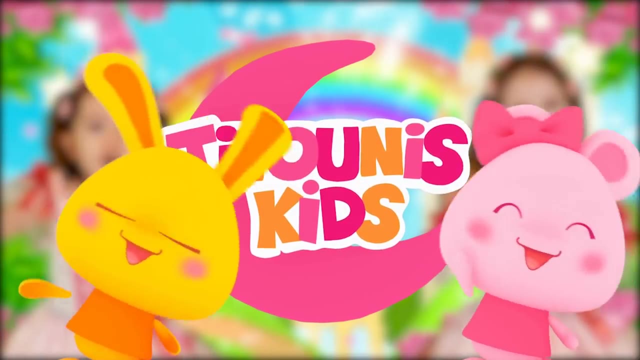 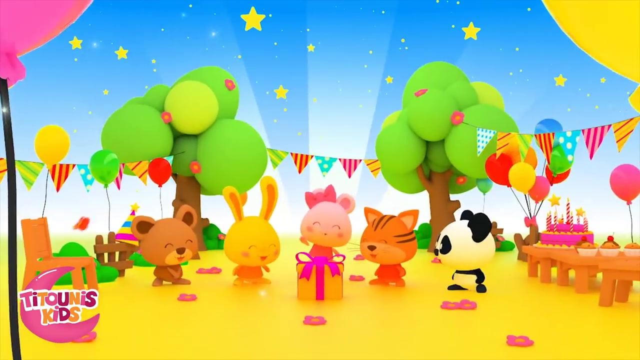 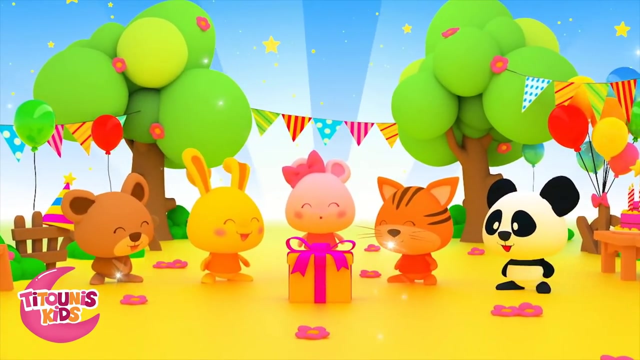 Oh princesses, dance, dance, dance. Oh princesses, come on, take a bow. Come on, take a bow. Hi friends of Say Tonight, Today is my birthday. Do you want to open the presents? Come on, let's discover the surprises. 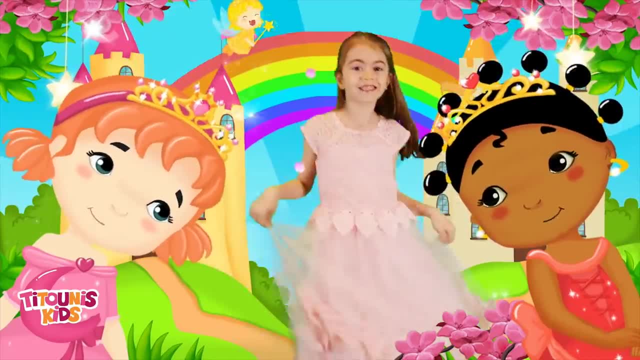 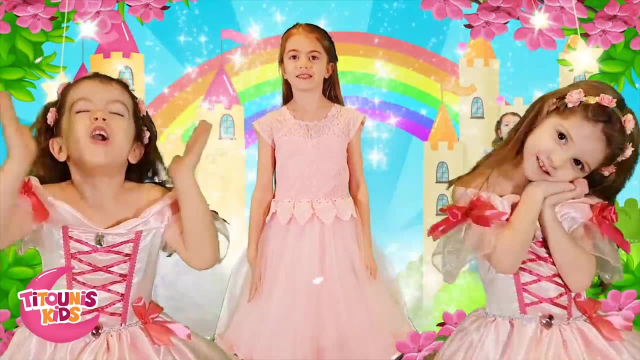 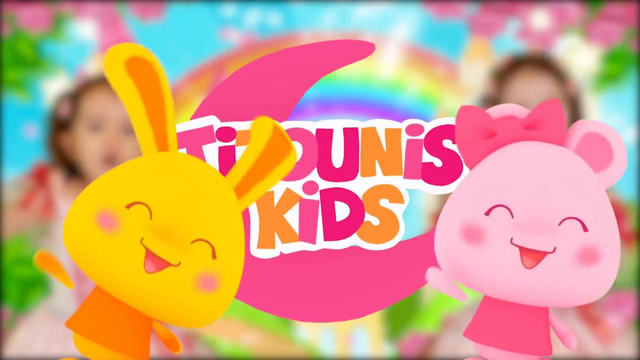 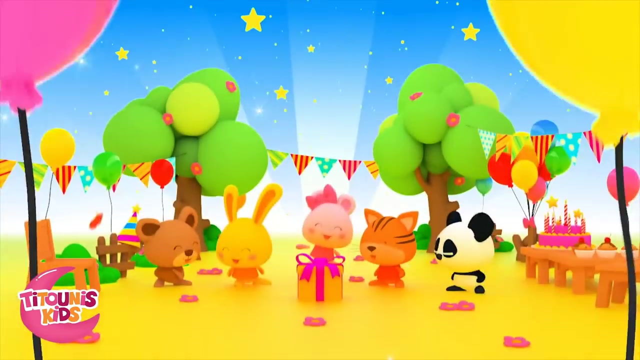 Oh princesses, dance, dance, dance. Oh princesses, come on, take a bow. Take my hand and come with me. Oh princesses, dance, dance, dance. Oh princesses, come on, take a bow. Hi, friends of Satanese, Today is my birthday. 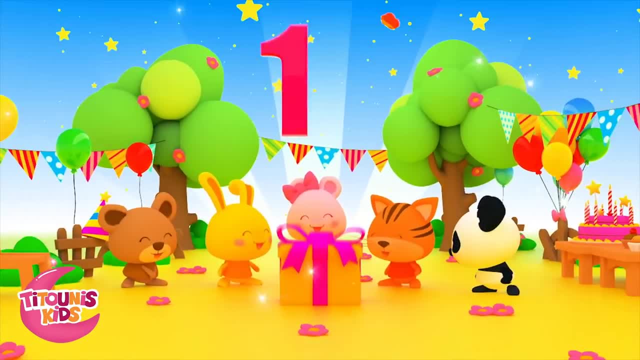 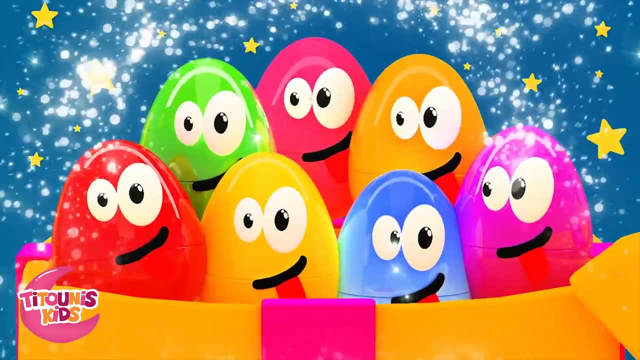 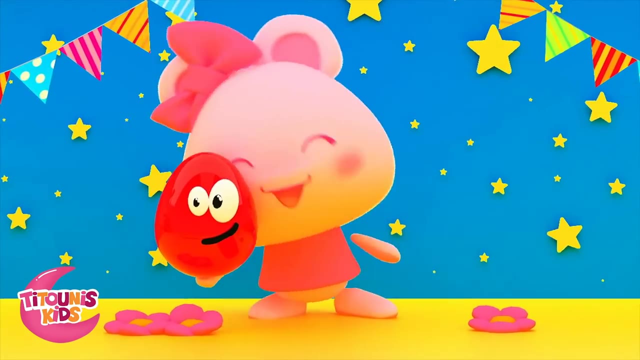 Do you want to open the presents? Let's discover the surprises. One, two, three. Oh look, These are colored surprise eggs. Let's open the red one. Mech mech mech- what's hiding in the egg? Mech mech mech- what's hiding in the egg? 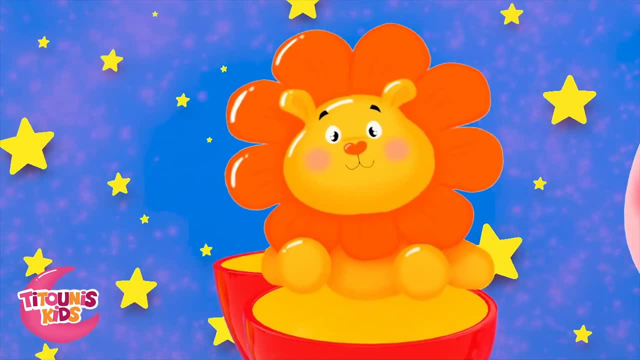 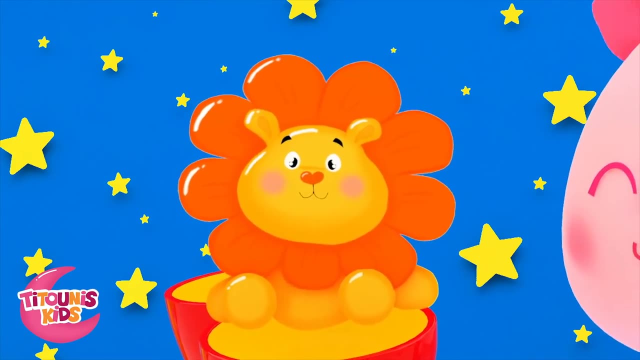 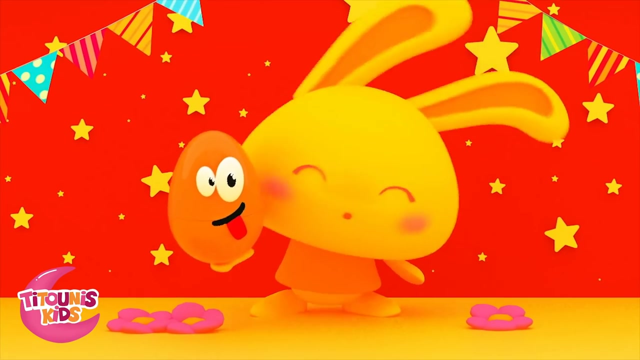 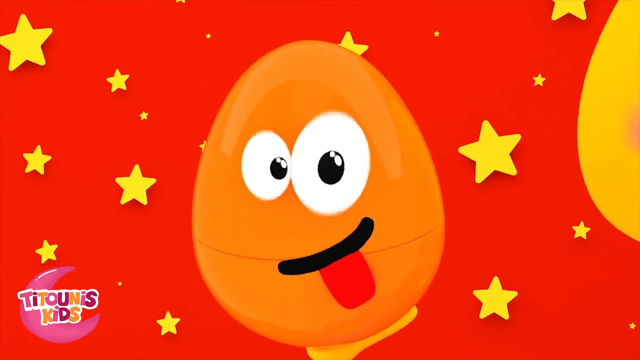 One, two, three. Oh, it's a magnificent lion. Let's open another surprise egg, The orange one. Mech mech mech. what's hiding in the egg? Mech mech mech. what's hiding in the egg? One, two, three. 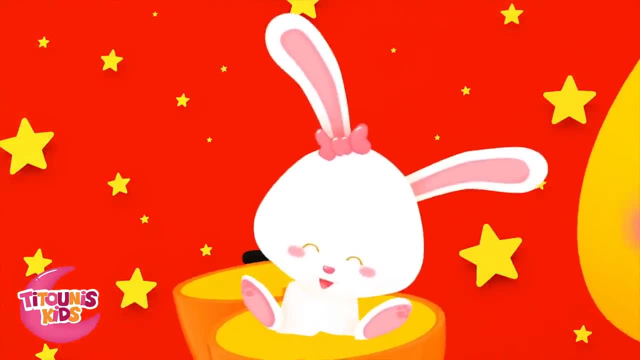 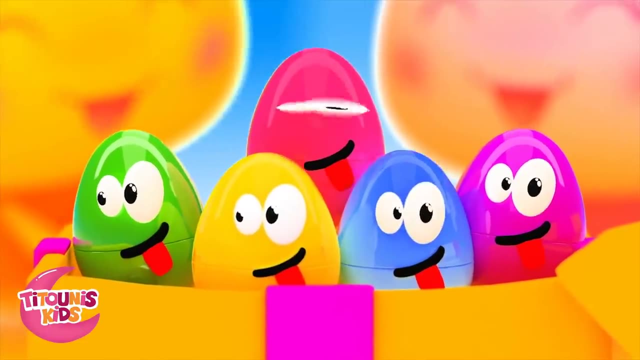 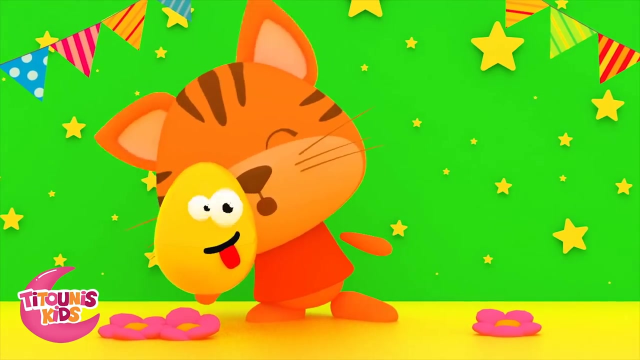 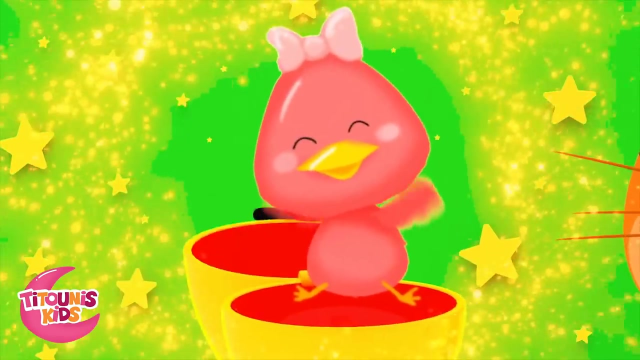 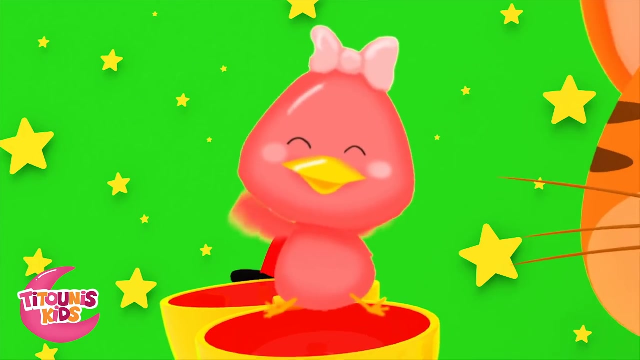 Oh, a cute bunny. Let's open another one, The yellow egg. Mech mech mech. what's hiding in the egg? Mech mech mech. what's hiding in the egg? One, two, three, A little bird- How cool. Let's open another surprise egg. 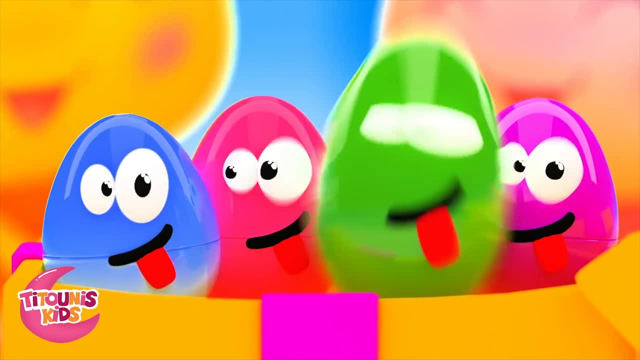 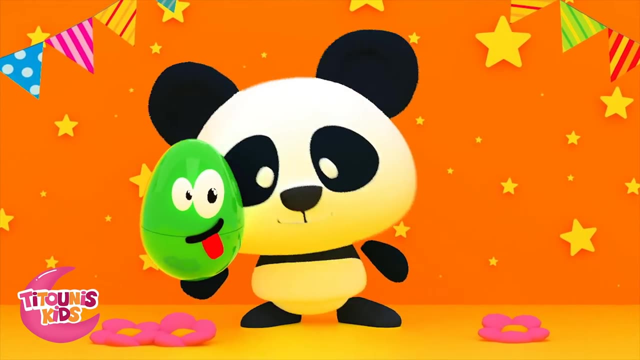 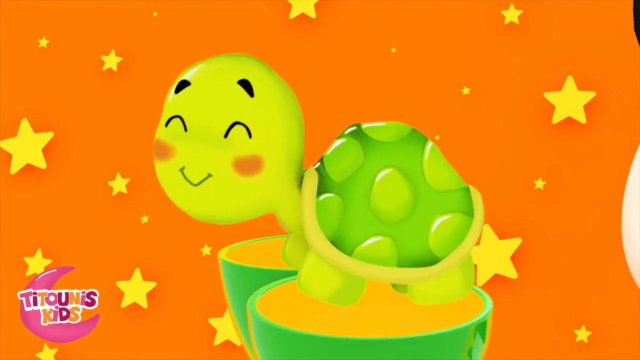 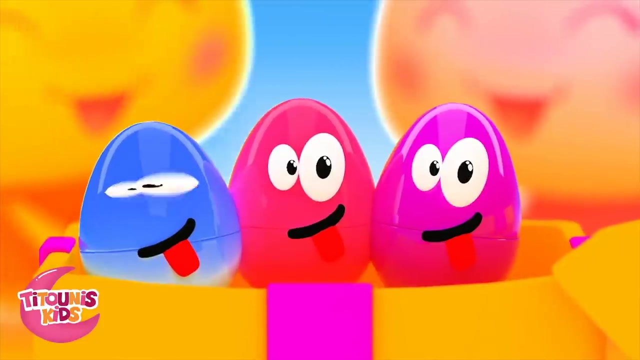 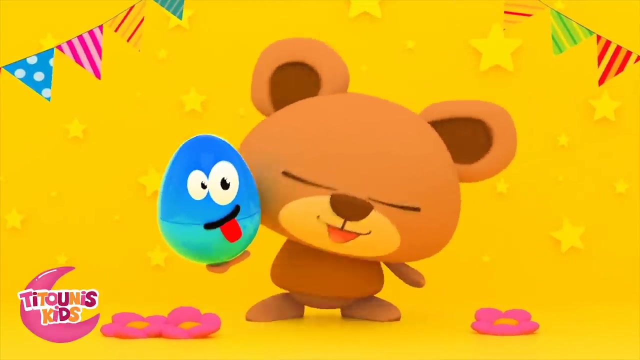 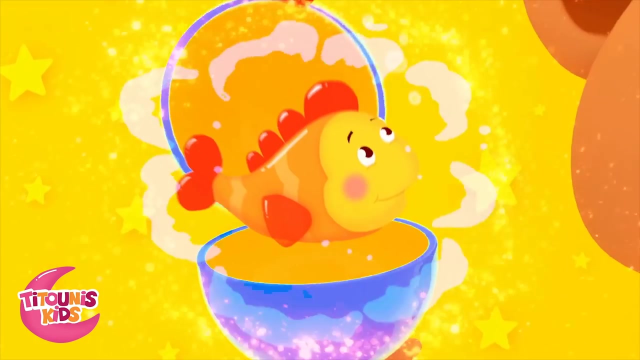 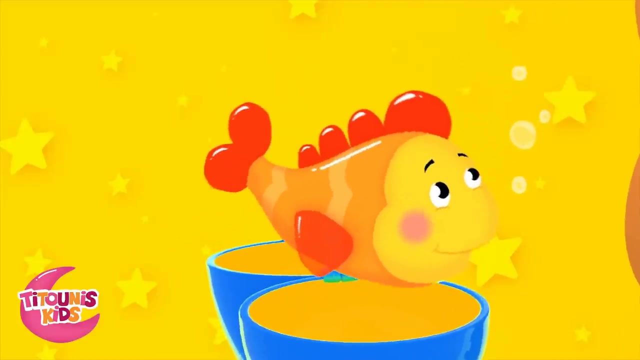 The green one: Mech mech mech. what's hiding in the egg? Mech mech mech. what's hiding in the egg? Mech mech mech. what's hiding in the egg? Wow, A beautiful little fish. Let's open another surprise egg. 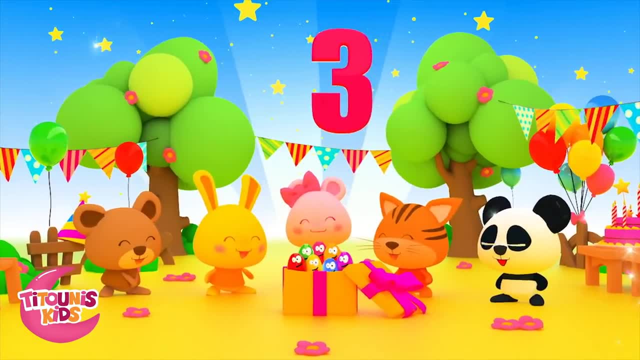 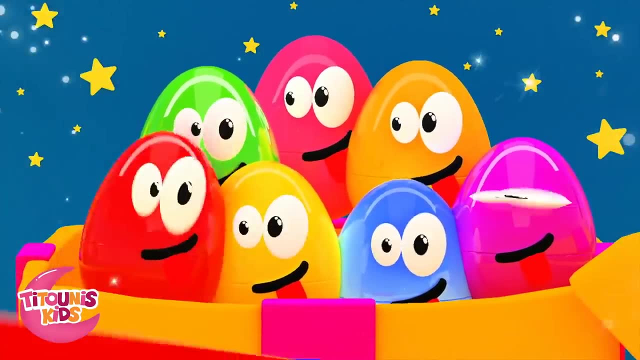 One, two, three. Oh, we're going to the fair. Oh, we're going to the fair. Oh look, These are colored surprise eggs. Let's open the red one. Mech, mech, mech. what's hiding in the egg? 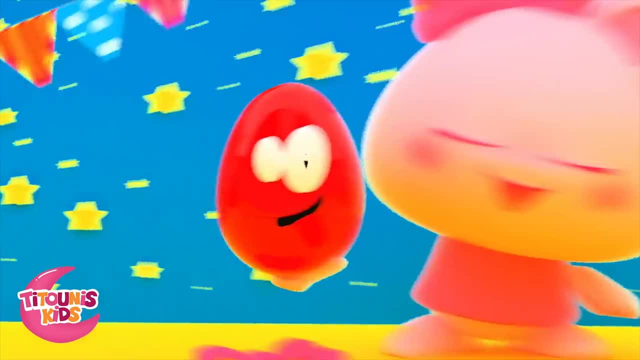 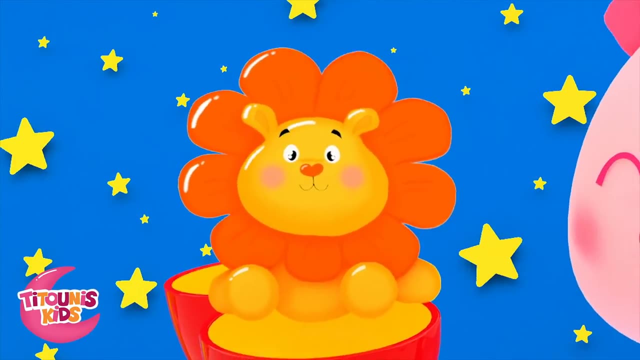 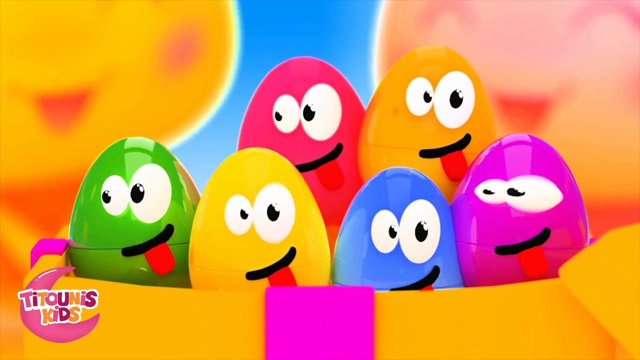 Mech mech mech, what's hiding in the egg? One, two, three. Oh, it's a magnificent lion. Let's open another surprise egg, The orange one. Mech mech mech, what's hiding in the egg? 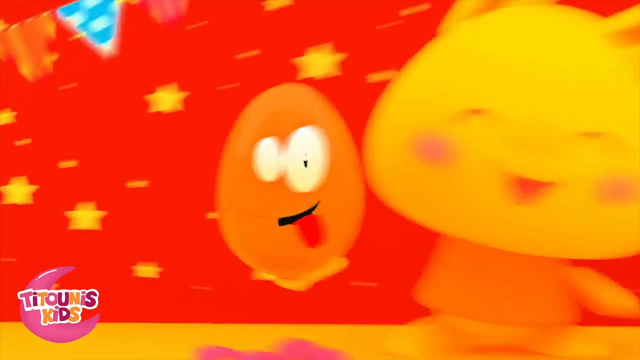 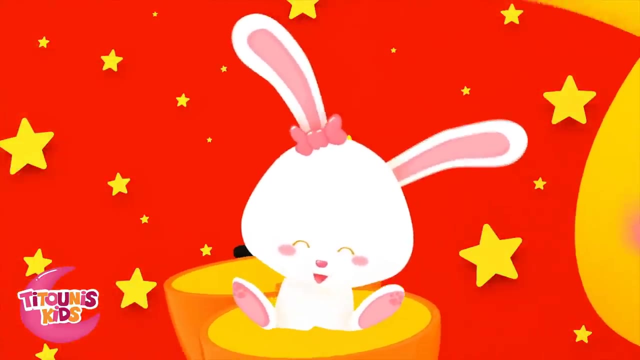 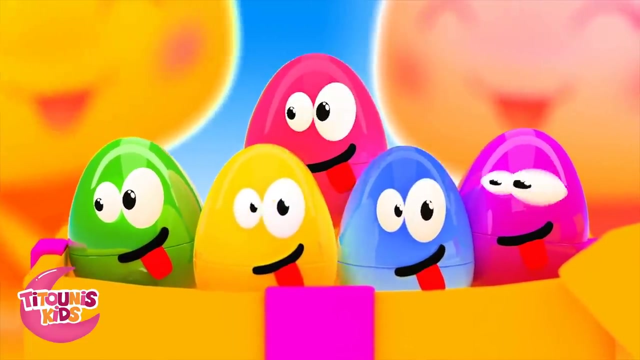 Mech mech mech, what's hiding in the egg? One, two, three. Oh a cute bunny, Let's open another one, The yellow egg. Mech mech mech, what's hiding in the egg? Mech mech mech, what's hiding in the egg? 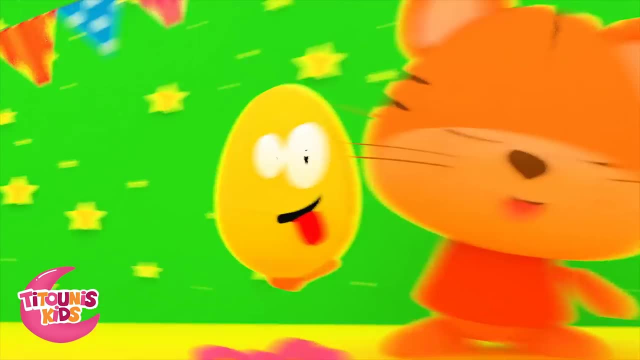 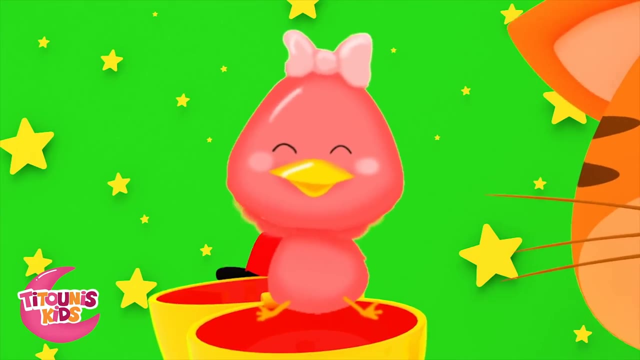 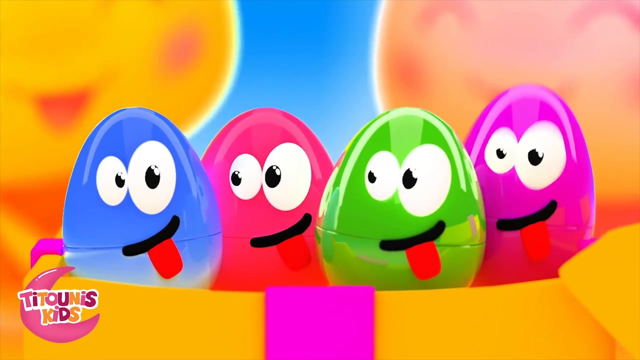 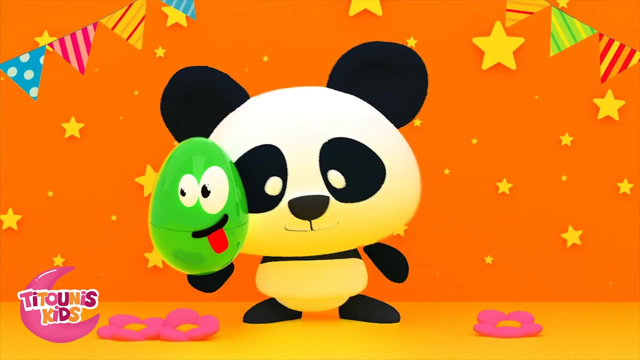 Mech mech mech. what's hiding in the egg? One, two, three. A little bird- How cool. Let's open another surprise egg, The green one. Mech mech mech, what's hiding in the egg? Mech mech mech. what's hiding in the egg? 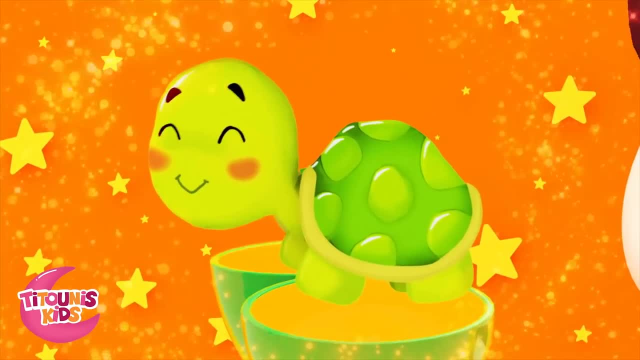 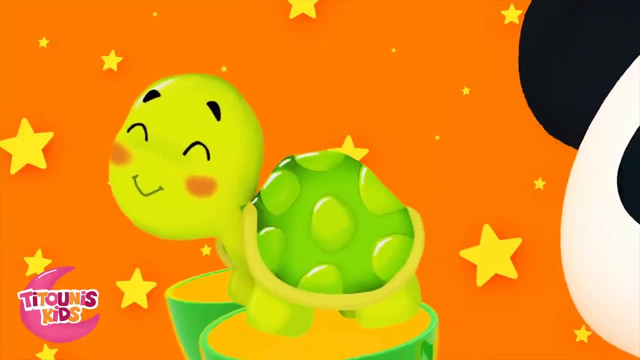 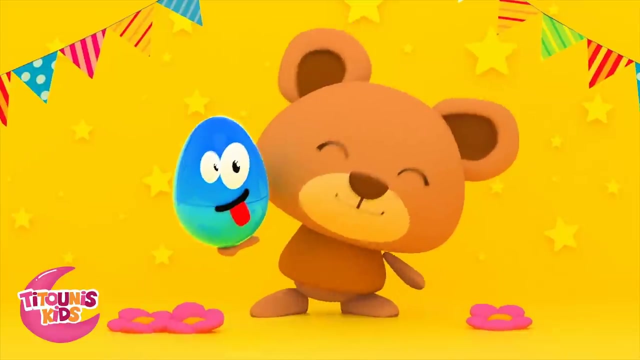 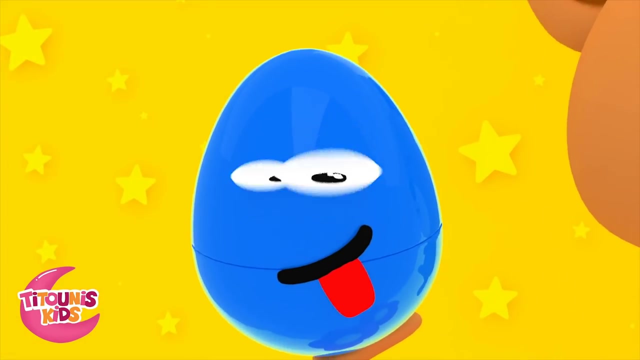 The blue one. Oh, it's a little turtle. Let's open another egg, The blue one. Mech, mech, mech. what's hiding in the egg? Mech, mech, mech. what's hiding in the egg? Wow, Wow. 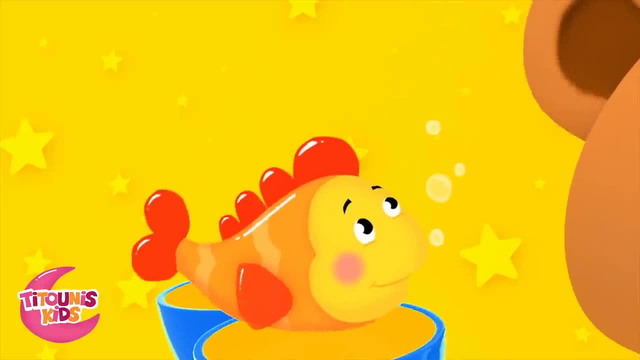 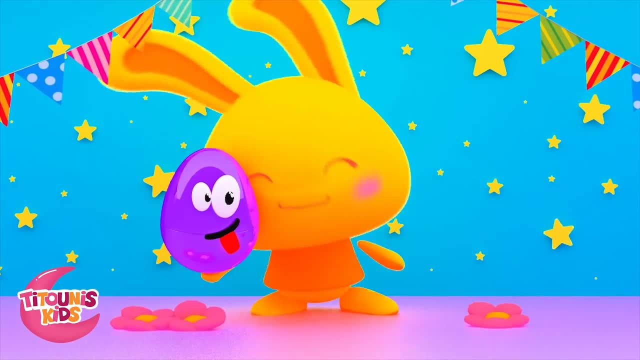 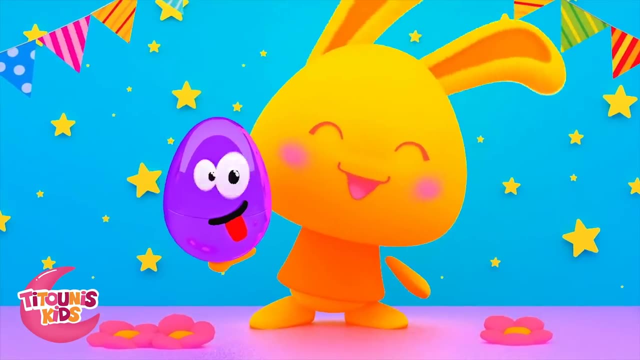 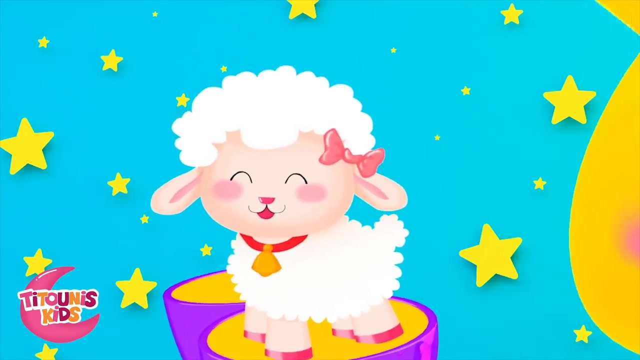 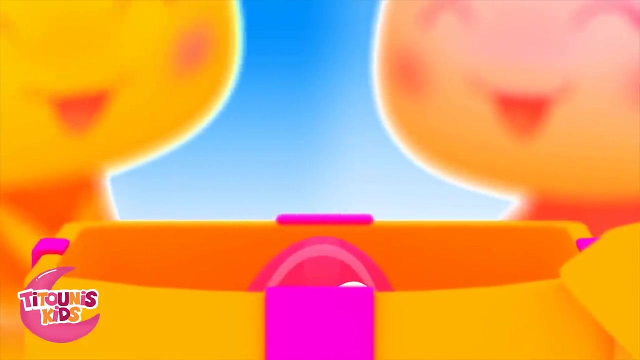 The purple egg. Mech mech mech. what's hiding in the egg? Mech mech mech. what's hiding in the egg? Oh, a little sheep, Let's open another one, The pink one. Meck meck meck was hiding in the egg. 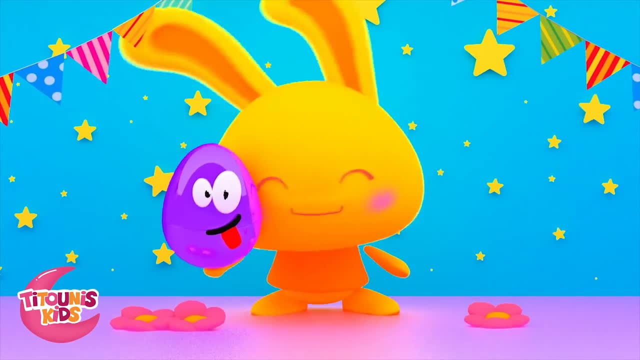 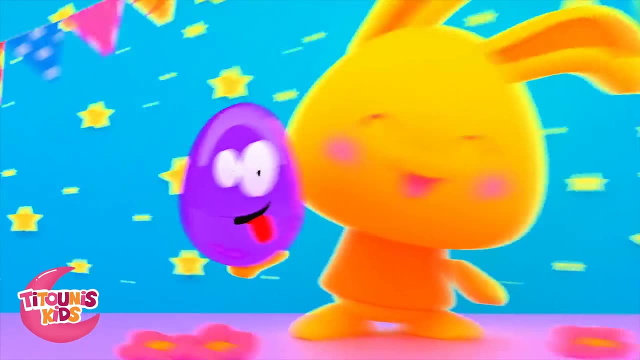 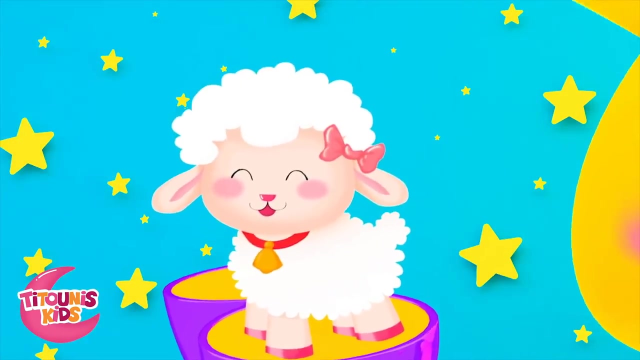 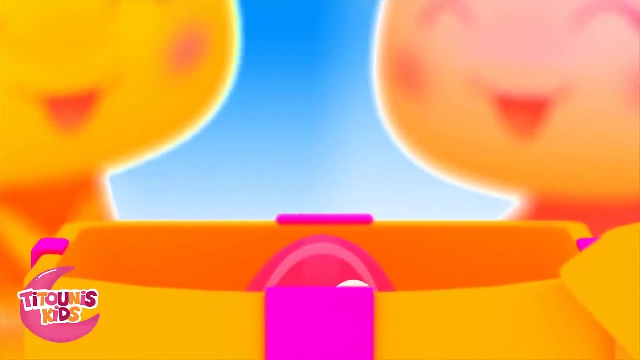 The purple egg: Meck meck meck was hiding in the egg. Meck meck meck was hiding in the egg. Oh, a little sheep, Let's open another one, The pink one: Meck meck meck was hiding in the egg. 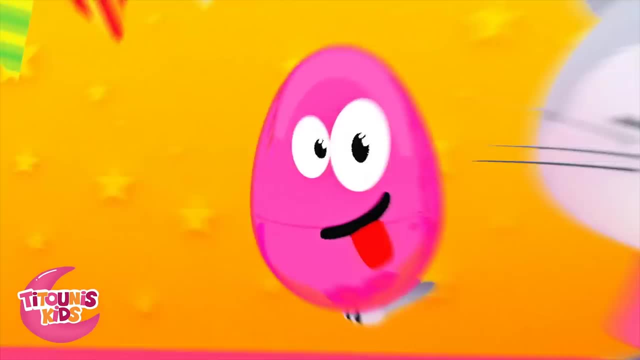 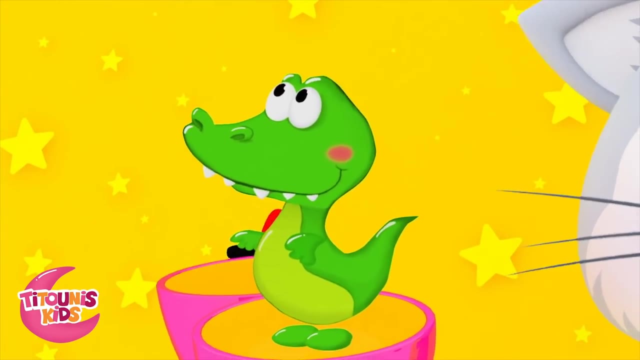 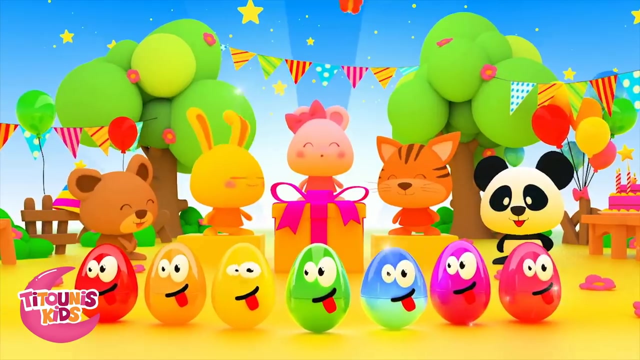 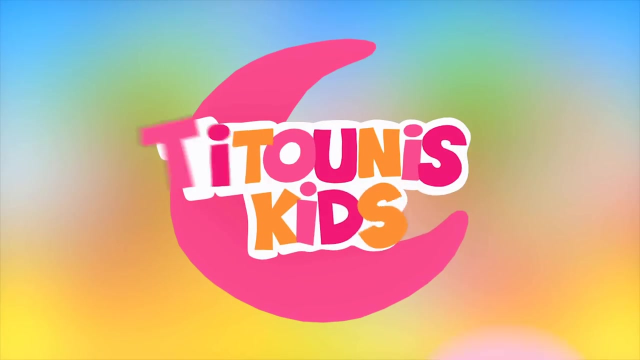 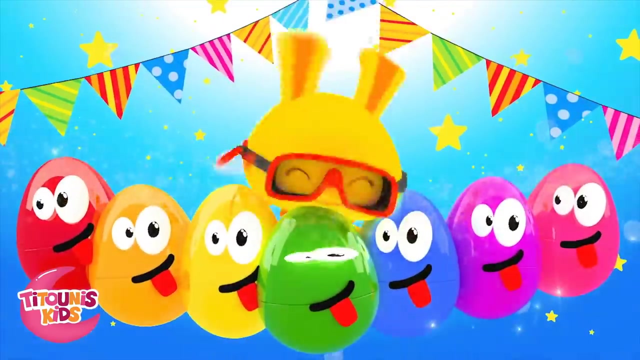 Meck meck meck was hiding in the egg, A little crocodile. Oh, the egg. The eggs have been opened. Thank you for these great birthday gifts And see you soon. girls and boys, Hi, friends of the Tunis. 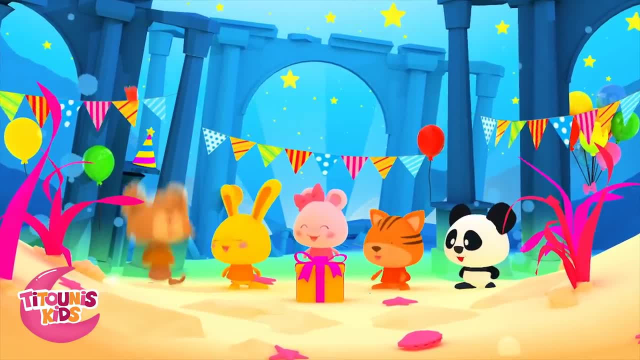 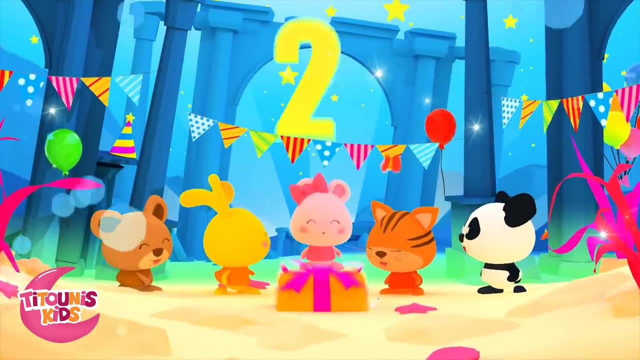 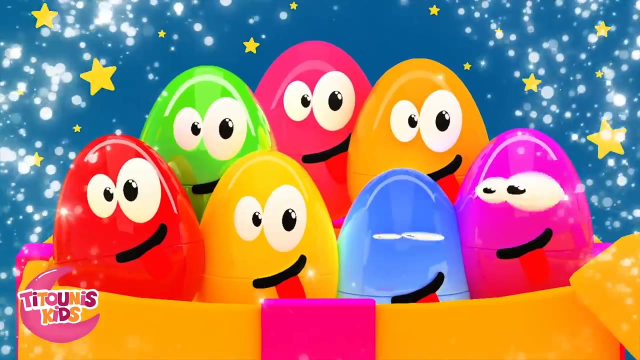 Let's open the eggs to find sea animals. Come on, let's discover the surprises. One, Two, Three, Oh look, These are colored surprise eggs. Let's open the red one. Meck meck meck was hiding in the egg. 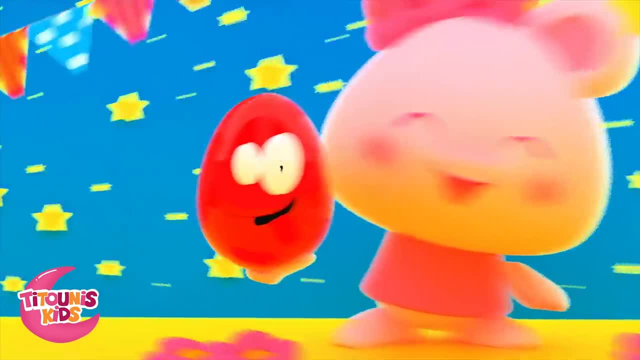 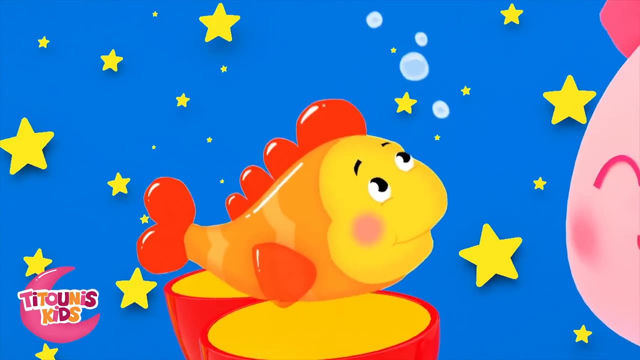 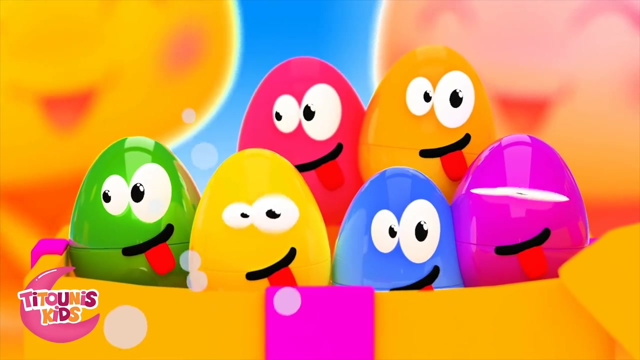 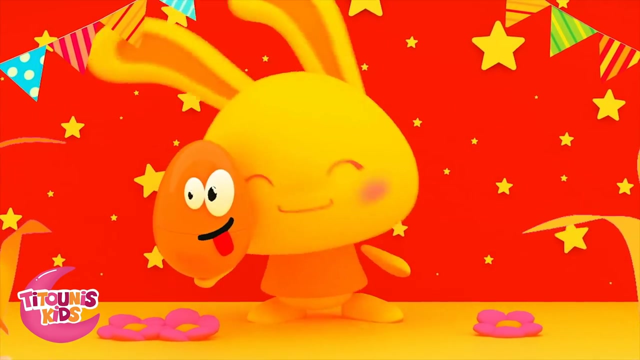 Meck meck meck was hiding in the egg. One, Two, Three. A cute little fish, Ha-ha. Let's open another surprise, The orange one. Meck meck meck was hiding in the egg. 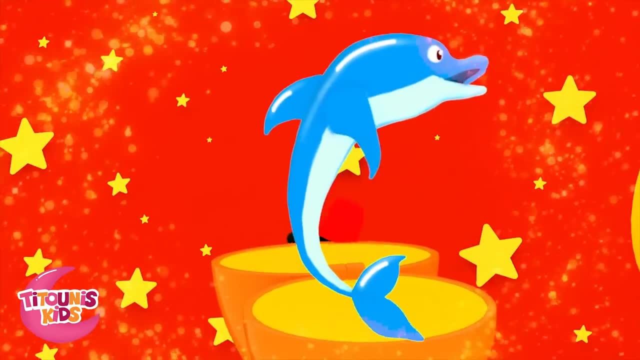 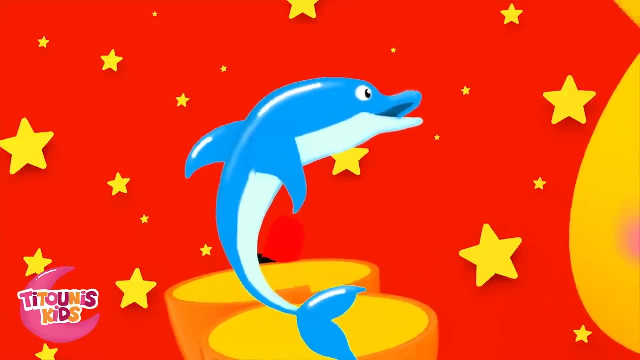 One, Two, Three. Cool, a magnificent dolphin. Let's open another one, The yellow egg. Meck, meck meck was hiding in the egg. Let's open another one: The yellow egg, The yellow egg, The yellow egg. 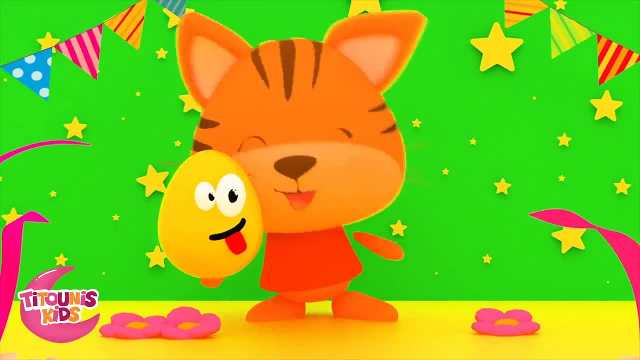 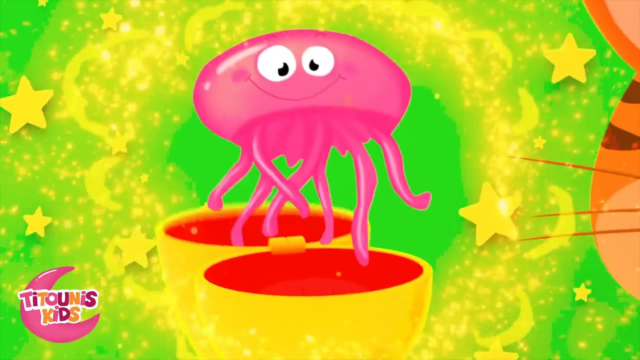 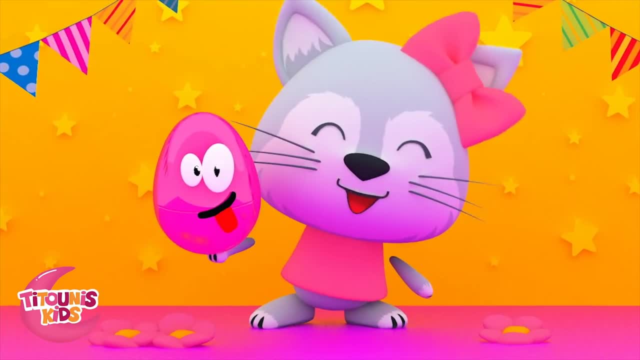 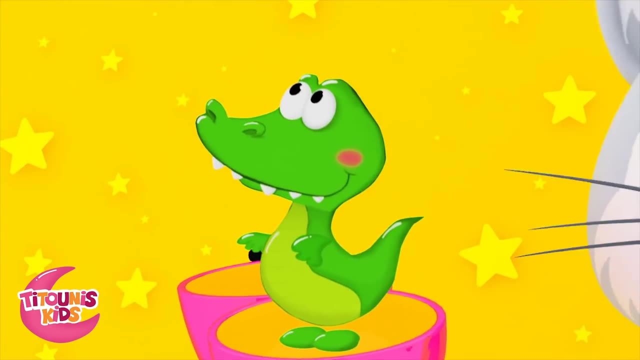 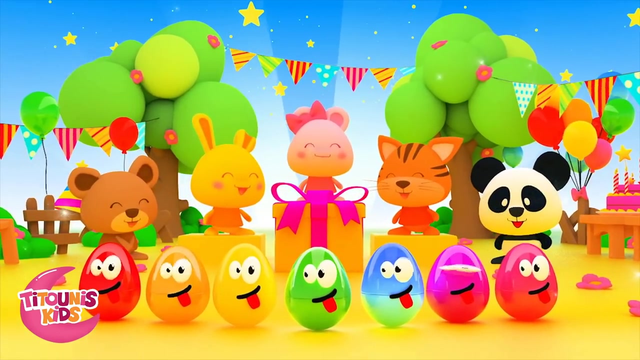 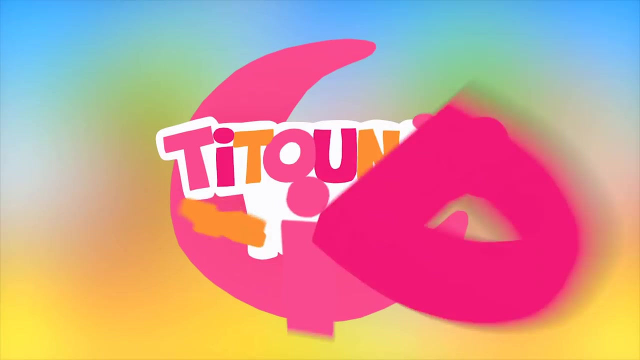 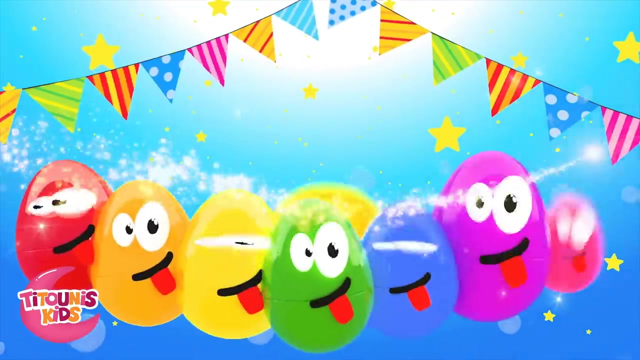 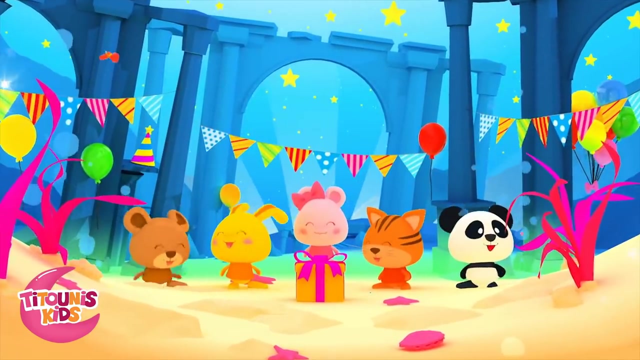 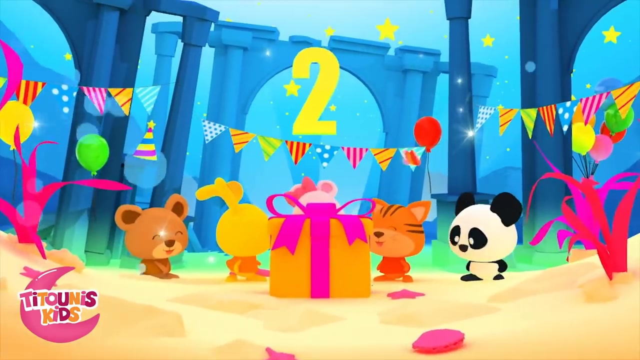 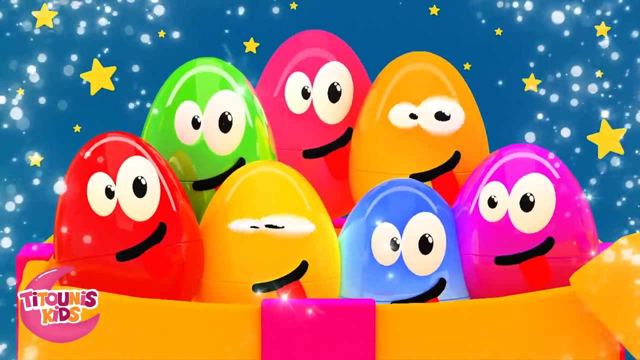 Meck meck meck was hiding in the egg- A little crocodile. All the eggs have been opened. Thank you for these great birthday gifts And see you soon. girls and boys, To be continued, Let's open the red one. 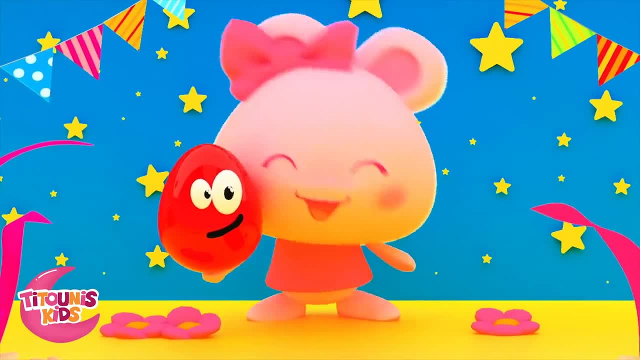 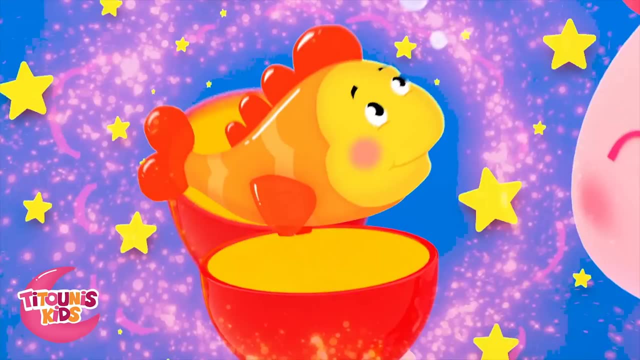 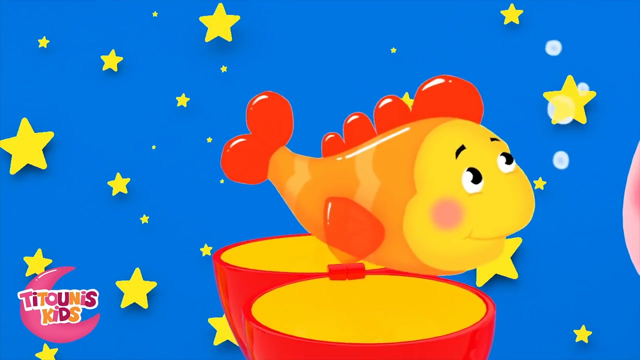 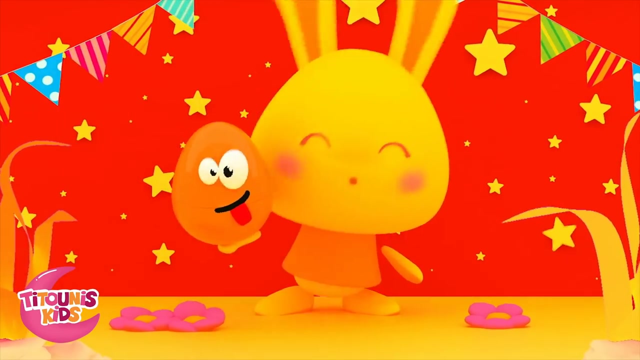 Meck meck meck was hiding in the egg. Meck meck meck was hiding in the egg. One, two, three. A cute little fish. Let's open another surprise egg, The orange one. Meck meck meck was hiding in the egg. 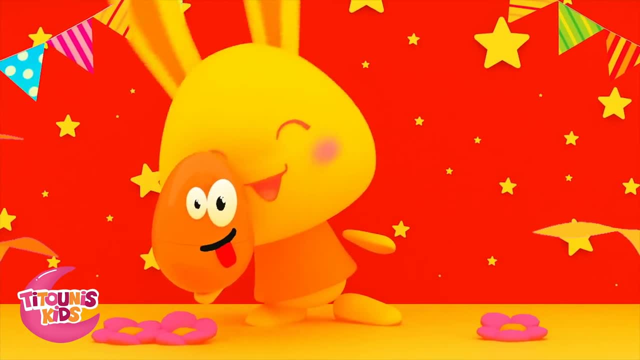 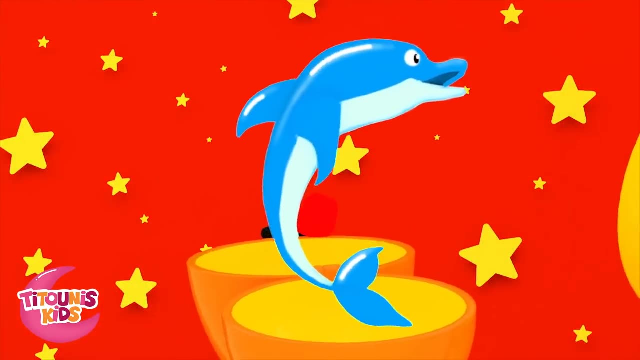 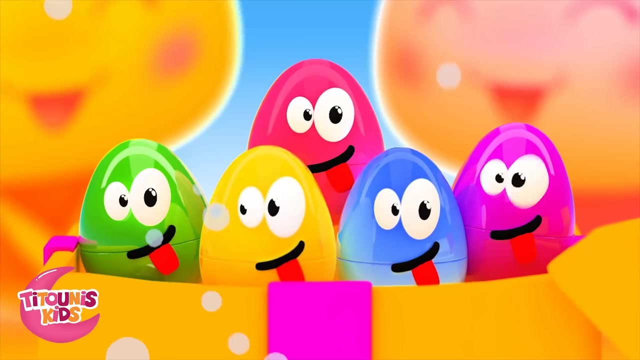 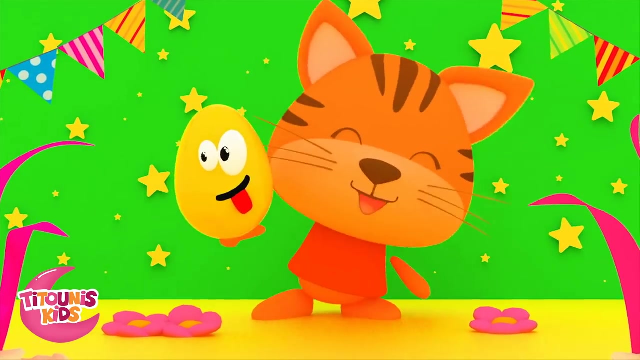 Meck meck meck was hiding in the egg. Meck meck meck was hiding in the egg. One, two, three, Cool, A magnificent dolphin. Let's open another one, The yellow egg. Meck meck meck was hiding in the egg. 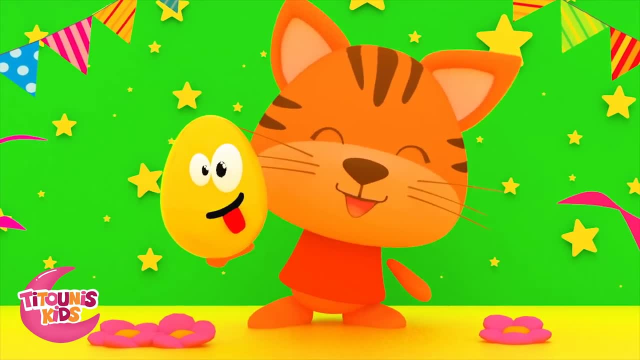 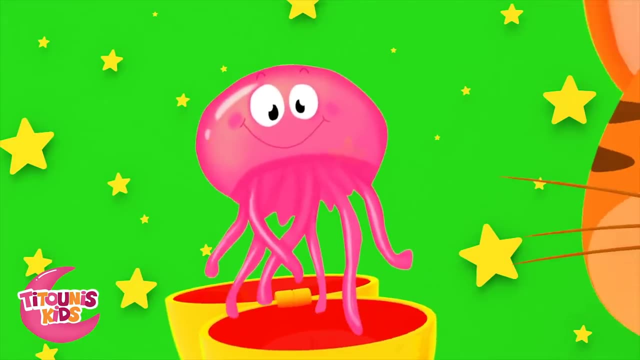 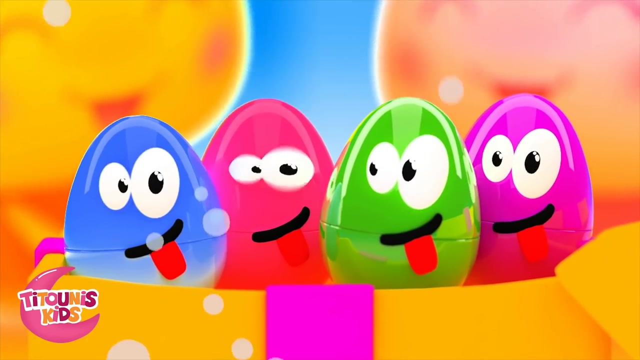 Meck meck meck was hiding in the egg. One, two, three, One, two, three A jellyfish. Be careful, Let's open another surprise egg, The green one. Meck meck meck was hiding in the egg. 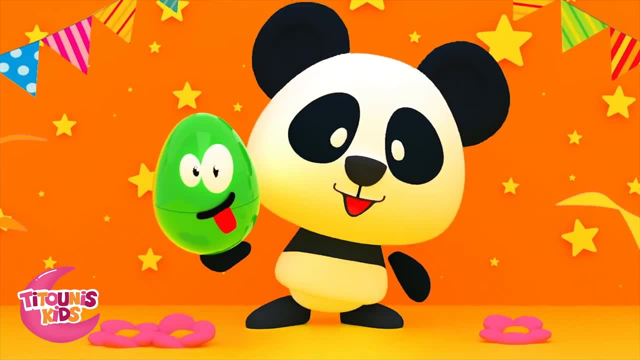 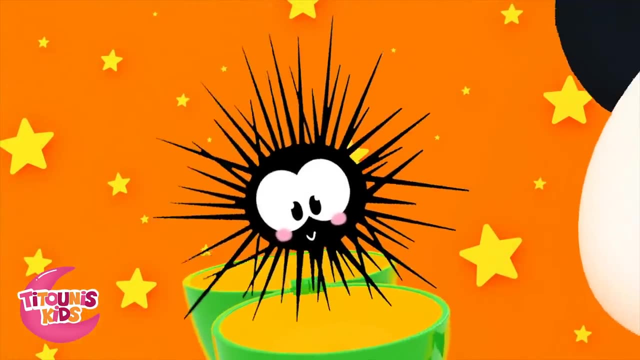 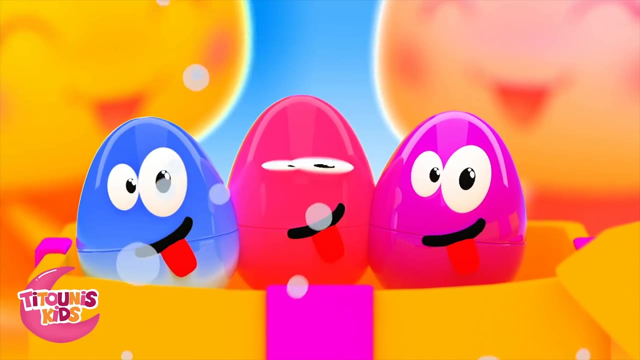 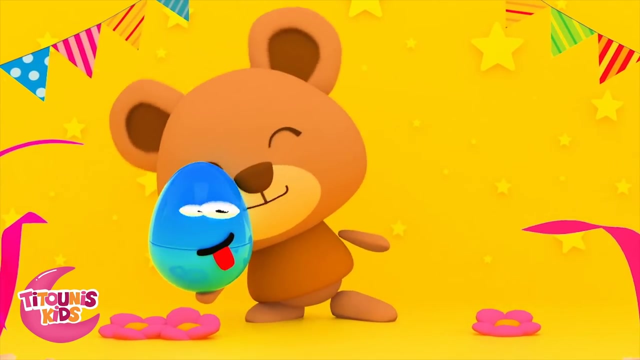 Meck meck meck was hiding in the egg. One, two, three. Oh A sea urchin, Let's open another egg, The blue one. Mech mech mech was hiding in the egg. Mech mech mech was hiding in the egg. 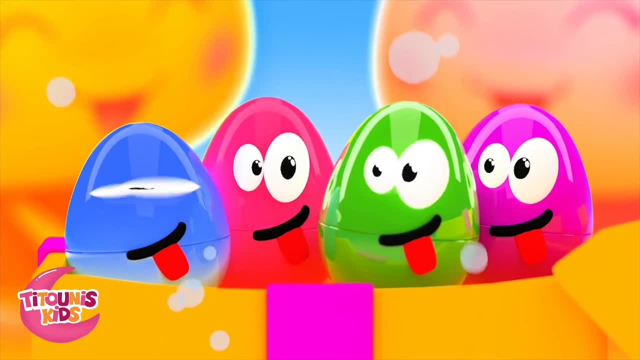 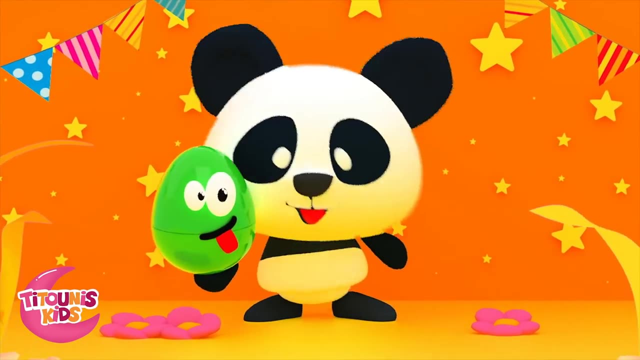 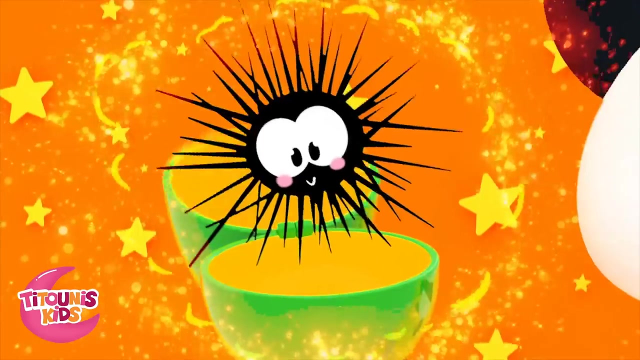 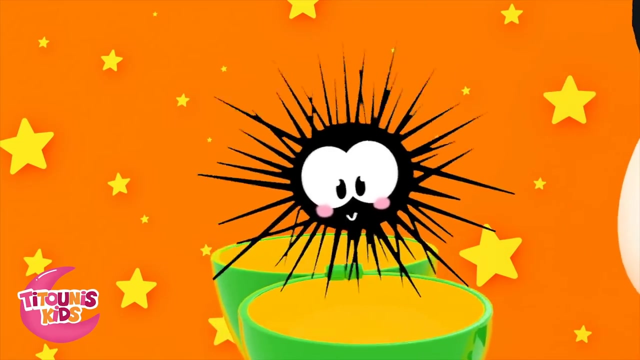 Let's open another surprise egg, The green one. Mac Mac Mac was hiding in the egg. Mac Mac Mac was hiding in the egg. One, two, three, Oh, a sea urchin. Let's open another egg, The blue one. 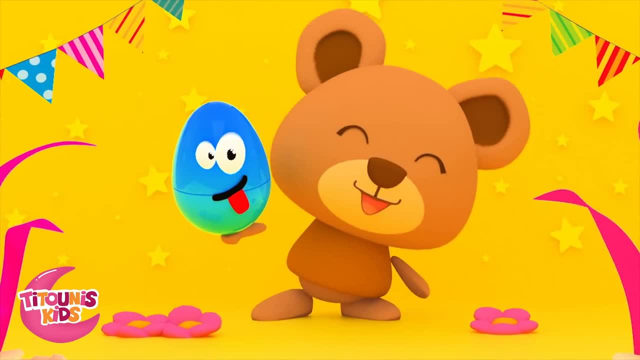 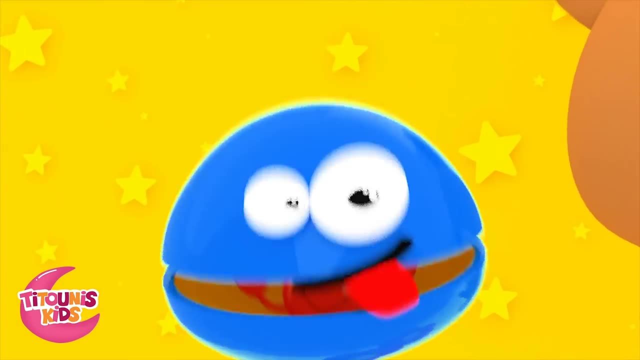 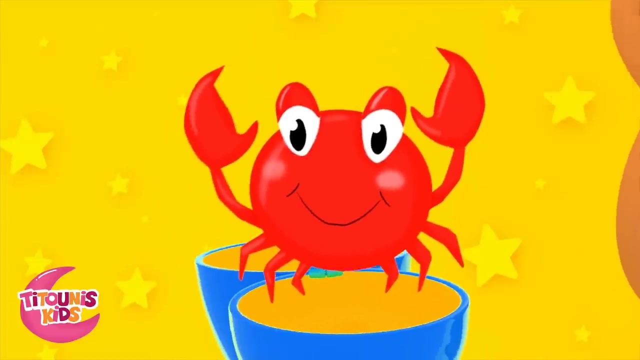 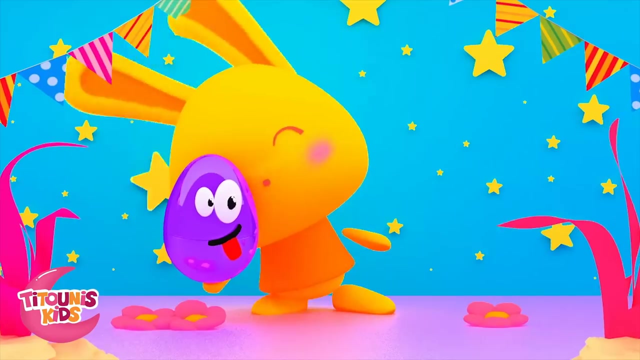 Mac Mac Mac was hiding in the egg. Mac Mac Mac was hiding in the egg. One, two, three, A big red crab. Wow, Let's open another surprise egg, The purple egg. Mac Mac Mac was hiding in the egg. 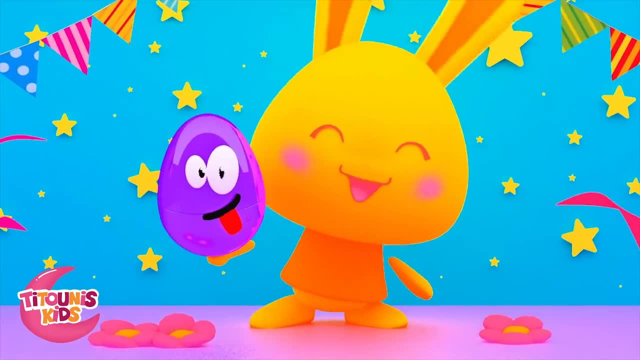 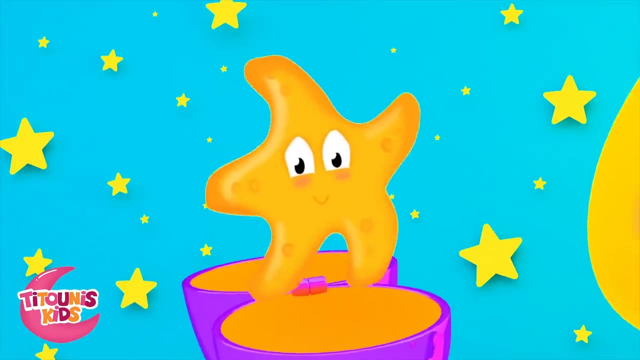 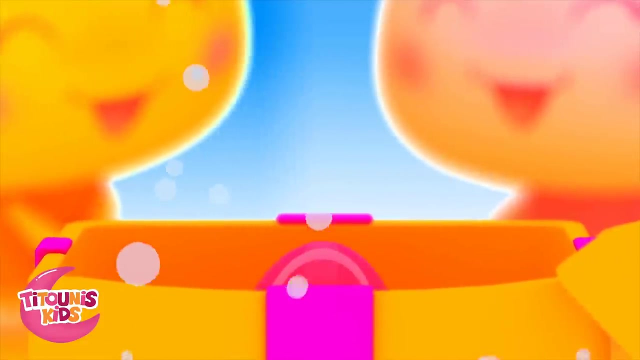 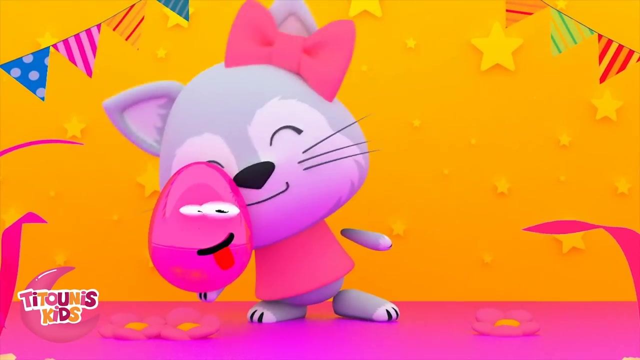 Mac Mac Mac was hiding in the egg. One, two, three, A little starfish, Let's open another one, The pink one. Mac Mac Mac was hiding in the egg. Mac Mac Mac was hiding in the egg. 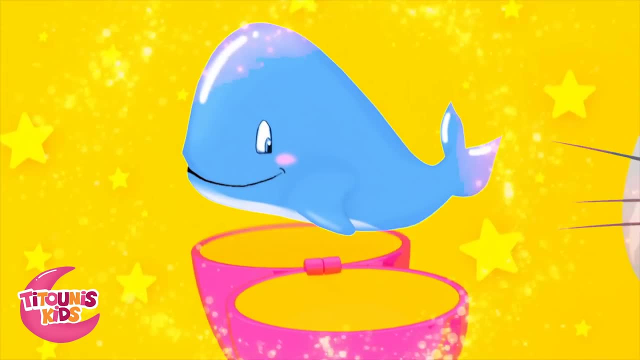 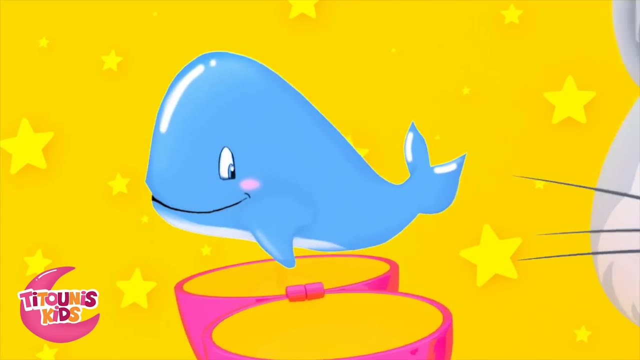 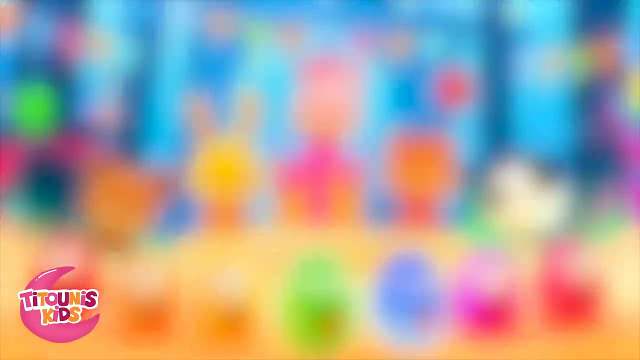 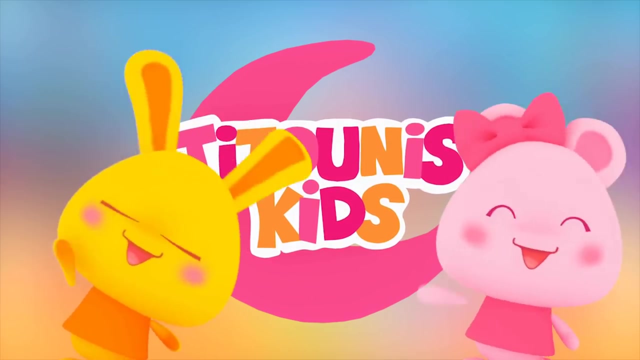 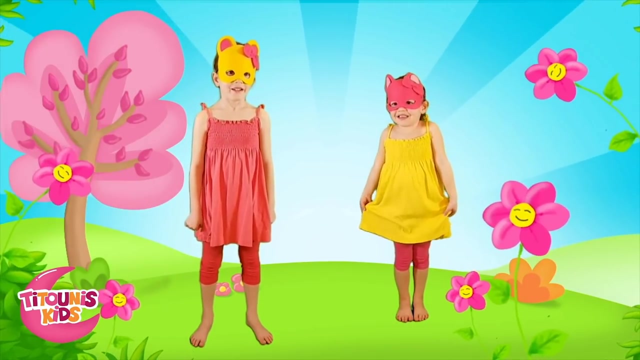 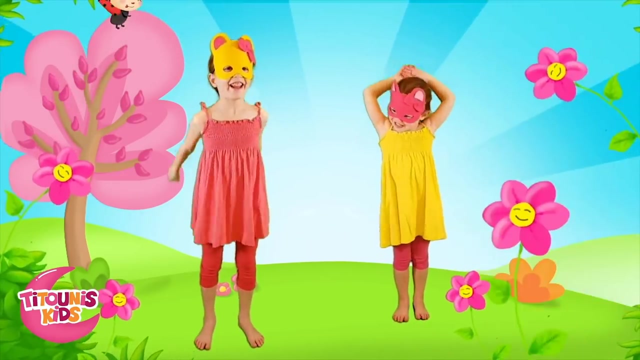 One, two, three And here there's a whale. Bravo, Bravo. Thank you for this great birthday And see you soon. girls and boys, Hi, Today we're doing some exercise. Are you ready? Let's warm up. 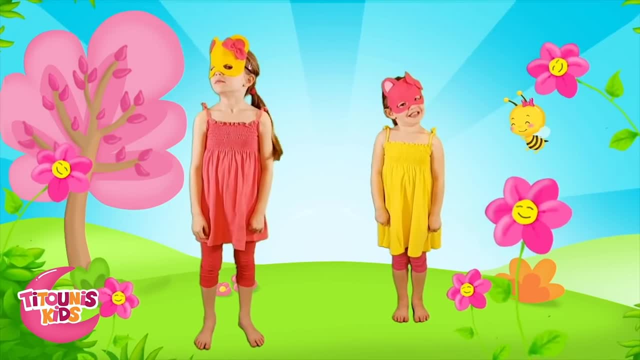 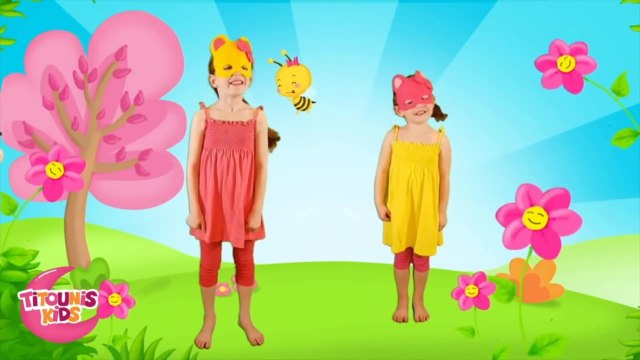 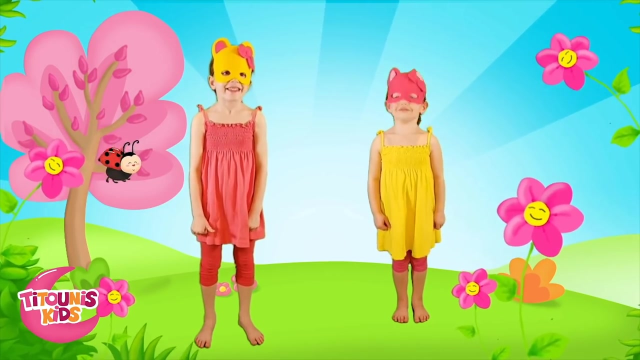 Move your head from left to right Like if you were a little girl, Like if you were saying no, Bravo. Now shake your head up and down As if you were saying yes, Perfect, Now bend your arms and move from right to left. 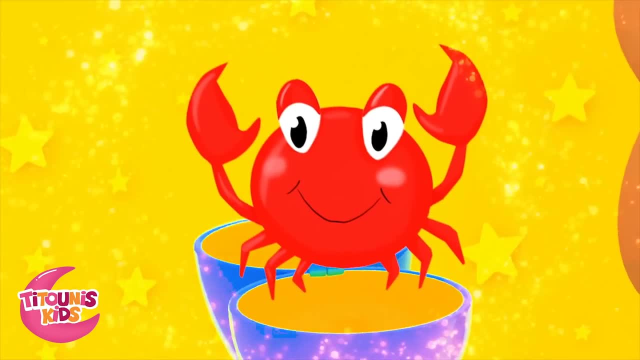 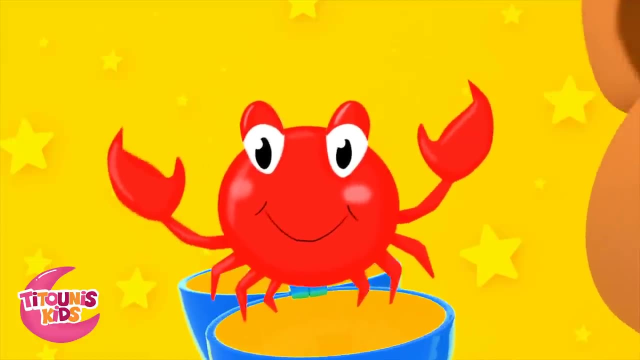 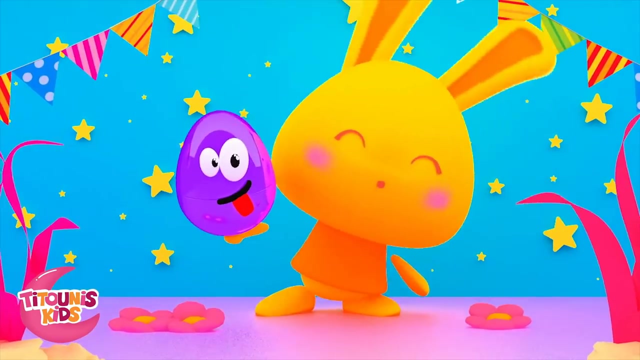 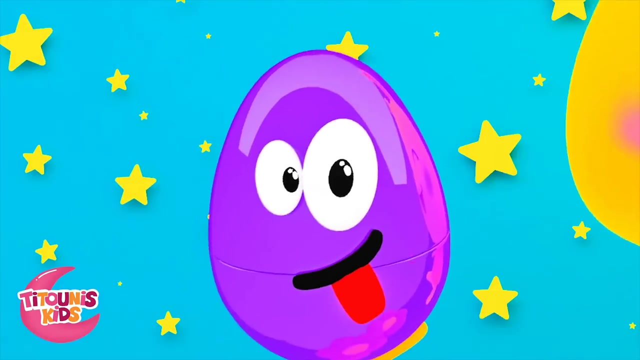 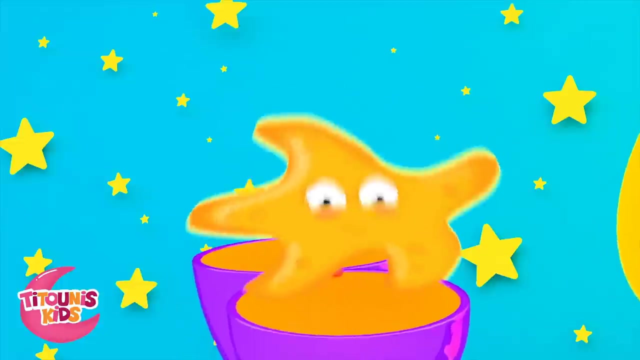 One, two, three. A big red crab. Wow, Let's open another surprise egg, The purple egg. Mech mech mech was hiding in the egg. Mech mech mech was hiding in the egg. One, two, three, A little starfish. Let's open another one. 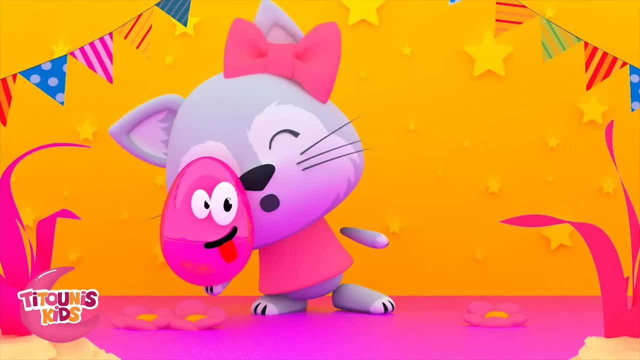 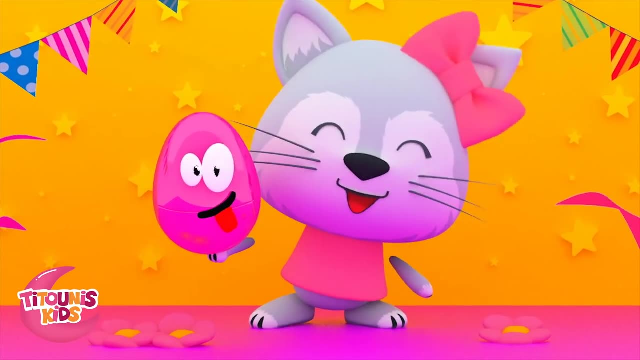 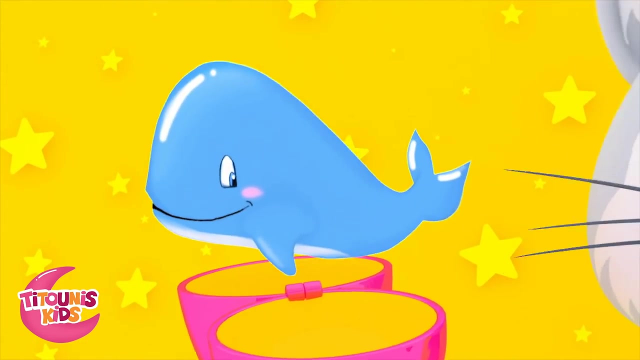 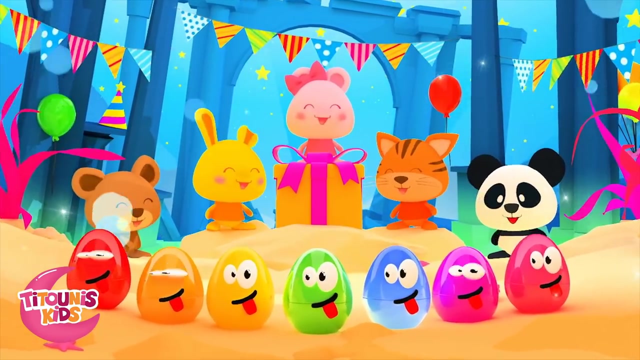 The pink one: Mech mech mech was hiding in the egg. Mech mech mech was hiding in the egg. Mech mech mech was hiding in the egg. One, two, three, And here there's a whale. Bravo, Bravo. Thank you for this great birthday gift. 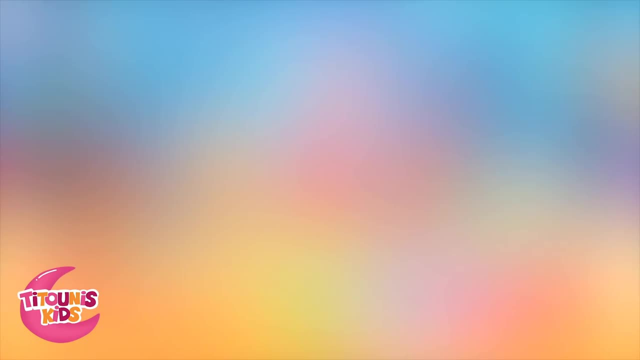 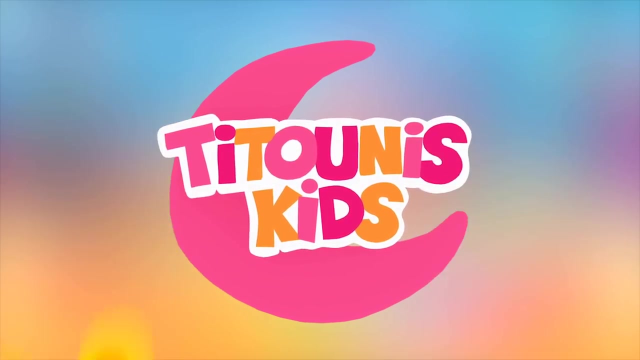 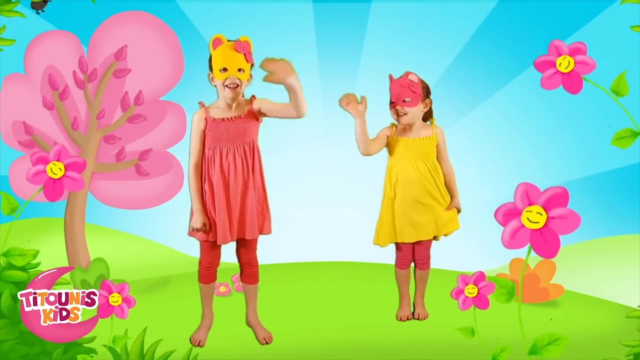 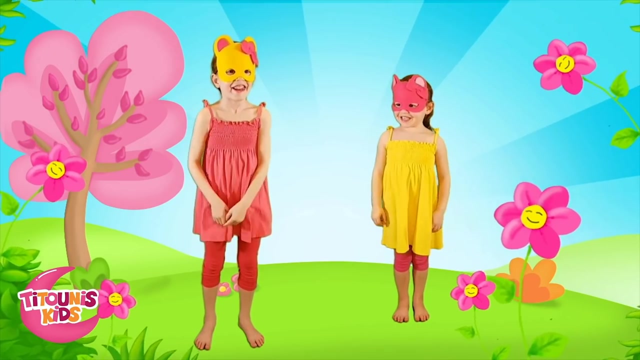 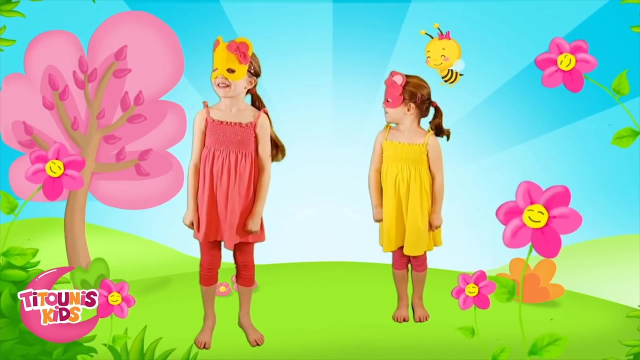 See you soon. girls and boys, Hi, Today we're doing some exercise. Are you ready? Yeah, Let's warm up. Move your head from left to right like if you were saying no, Bravo, Now. shake your head up and down. 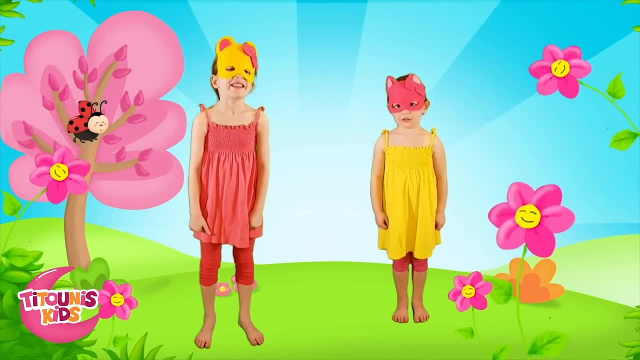 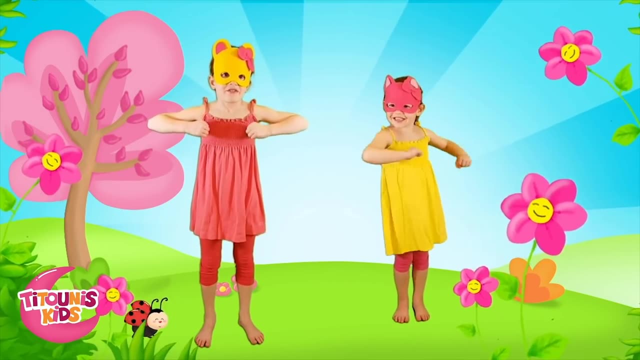 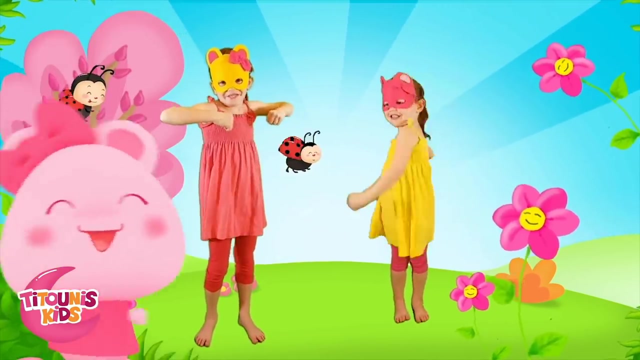 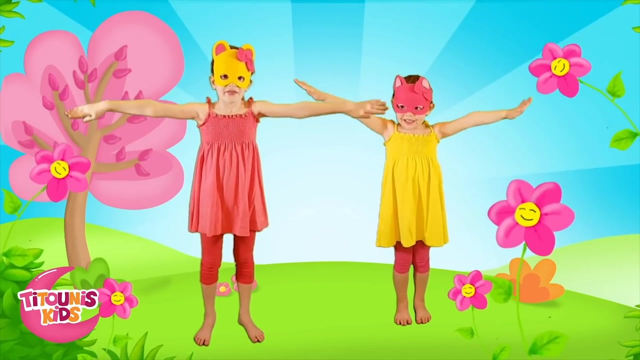 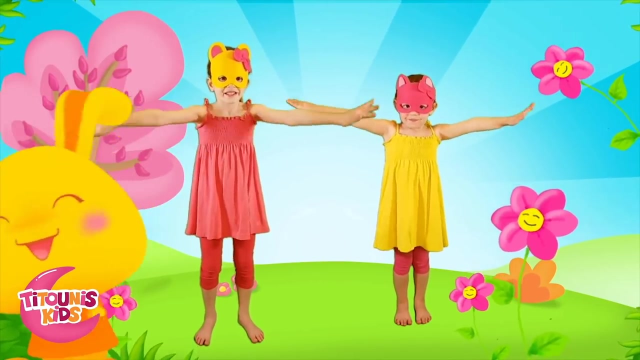 as if you were saying: yes, Perfect, Now bend your arms and move from right to left, Just like that Great, Let's raise our arms and make little circles. Well done, All right, we are done. warming up. Do you know what's next? 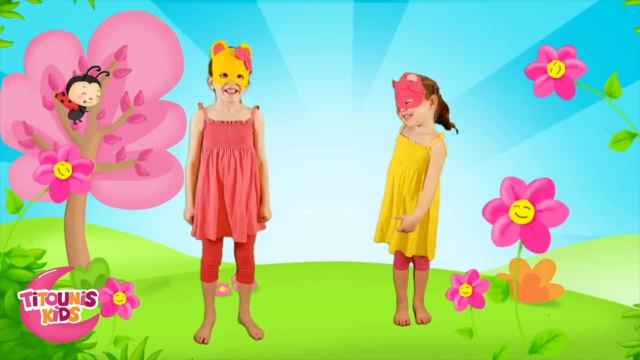 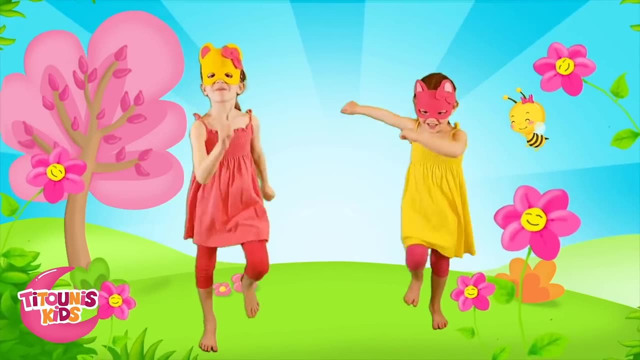 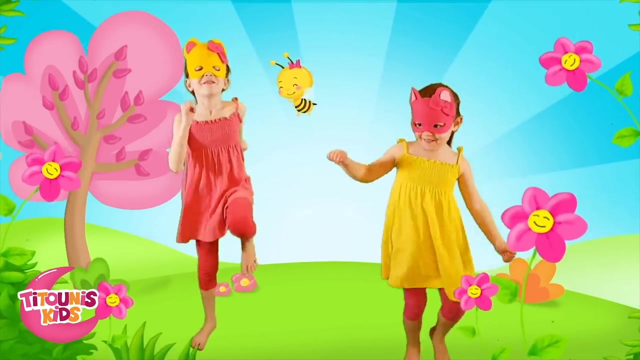 We're going to meet the characters from our favorite songs. Come on, let's march, But without moving from our spot. You have to lift your knees very high, Very good, Now start marching faster. Remember, don't move from your spot. 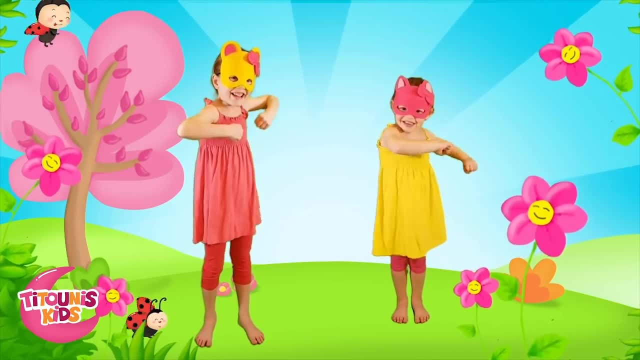 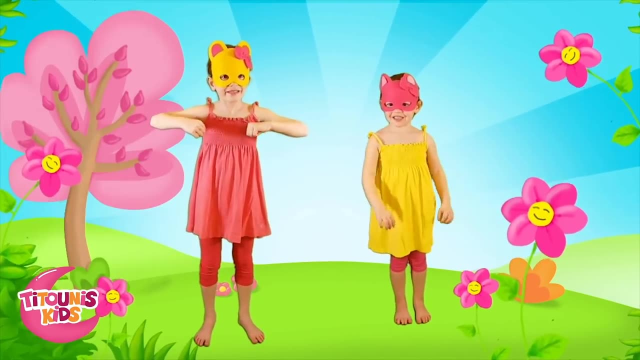 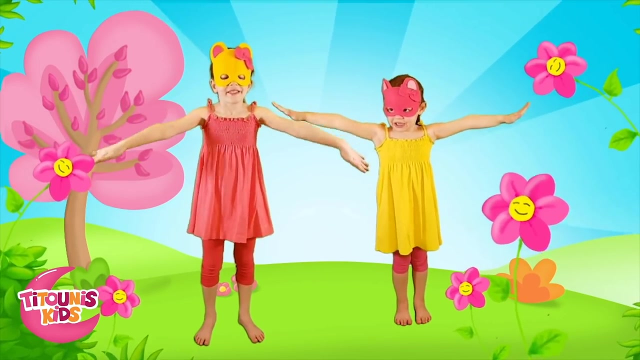 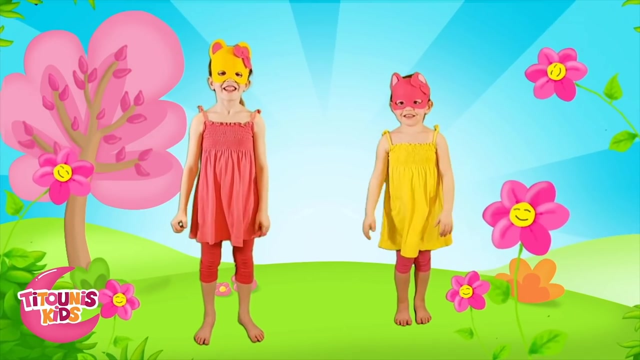 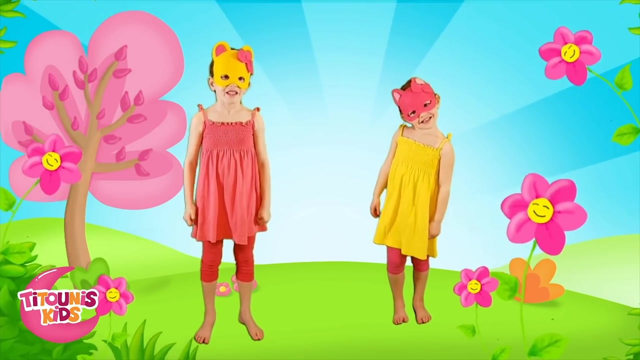 Just like that Great, Let's raise our arms and make little circles. Well done, Alright. we are done warming up. Do you know what's next? We're going to meet the characters from our favorite songs. Come on, let's march. 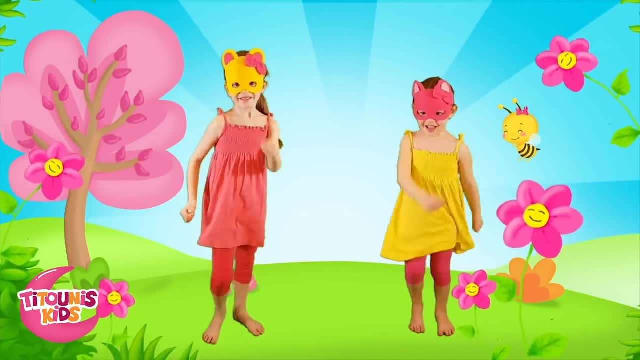 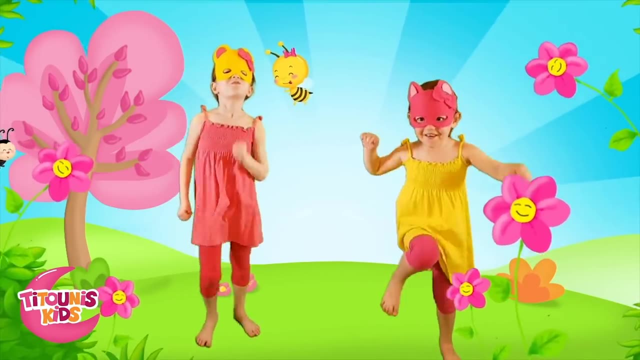 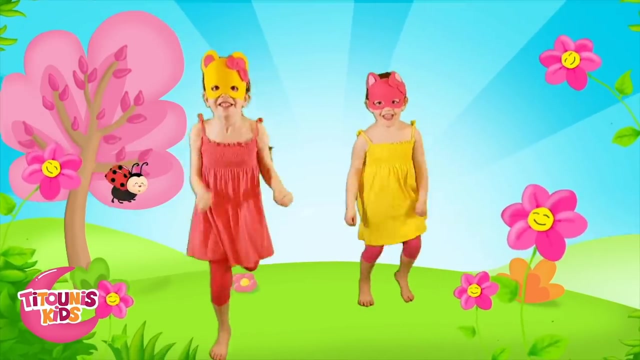 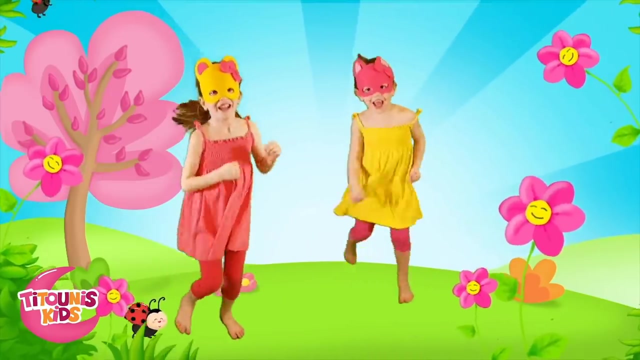 But without moving from our spot. You have to lift your knees Very high, Very good. Now start marching faster. Remember, don't move from your spot. Wow, You're going so fast. Let's pause for a bit and breathe deep. 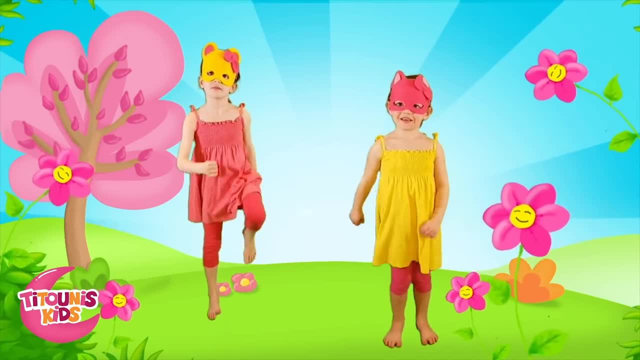 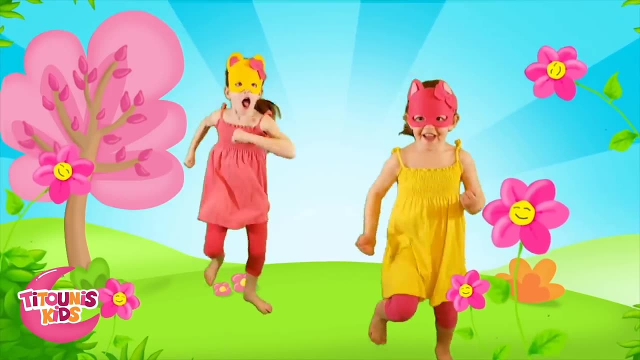 Then start to walk again calmly. Come on, now we're going to the beach And we have to run. Woof, It's so hot. How about we cool off? Let's go have some fun with the fishes, Sit down on the floor and swim. 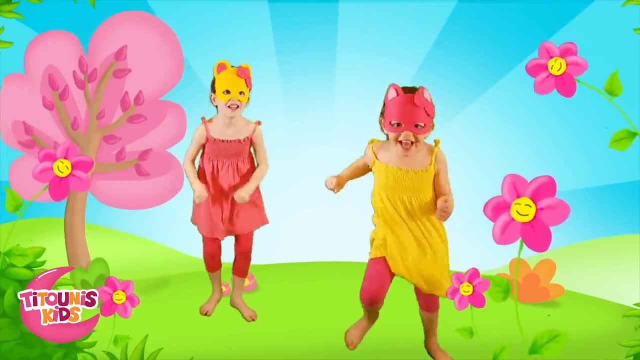 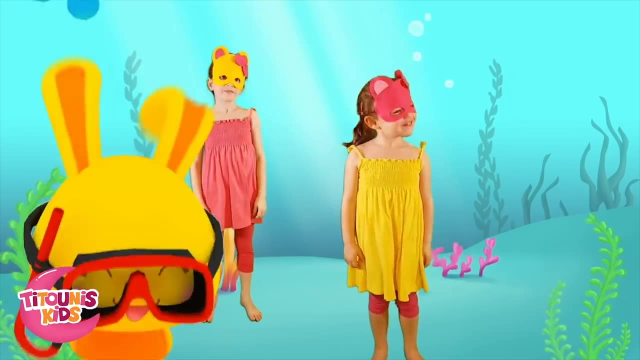 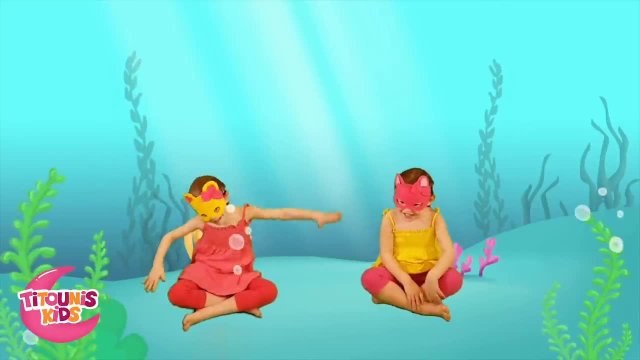 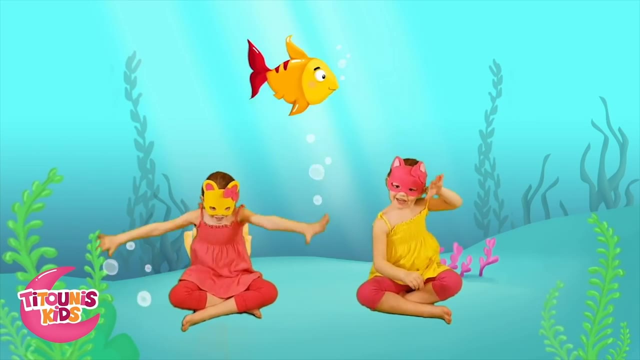 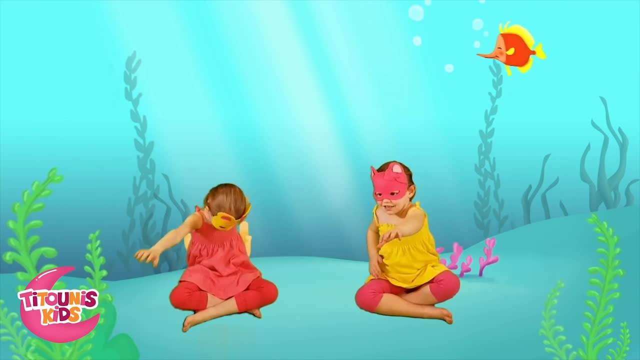 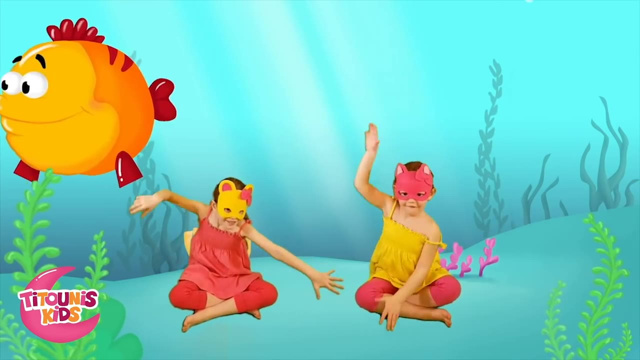 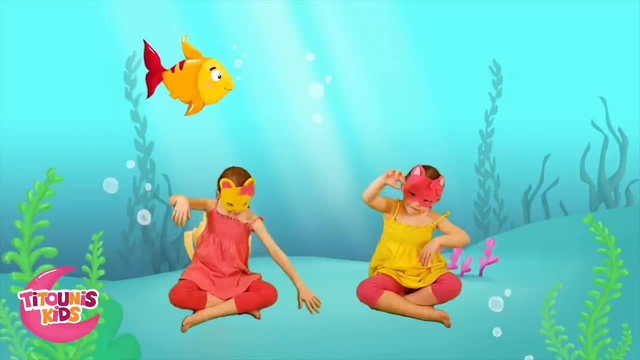 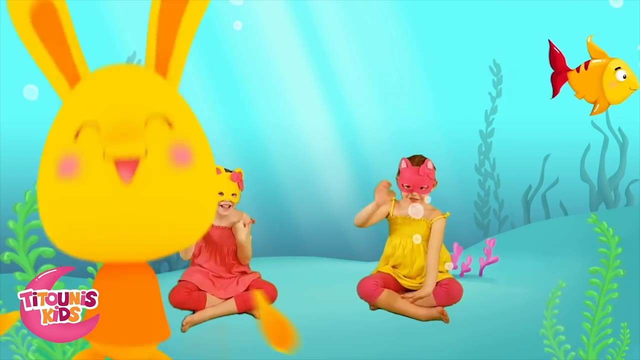 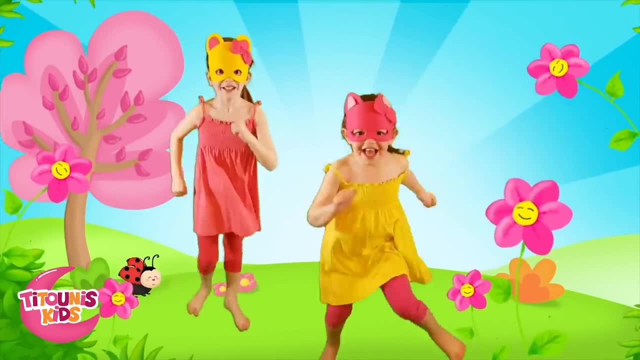 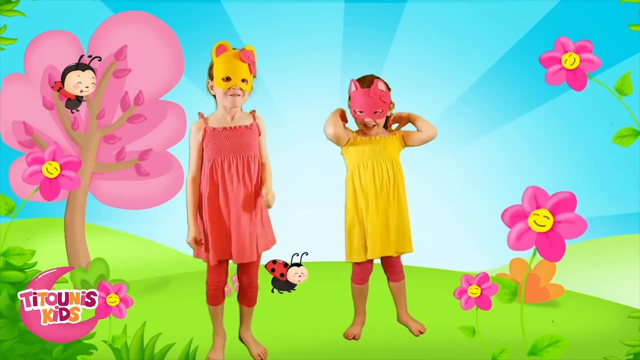 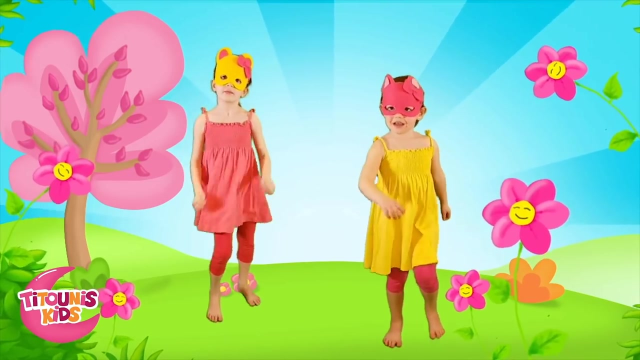 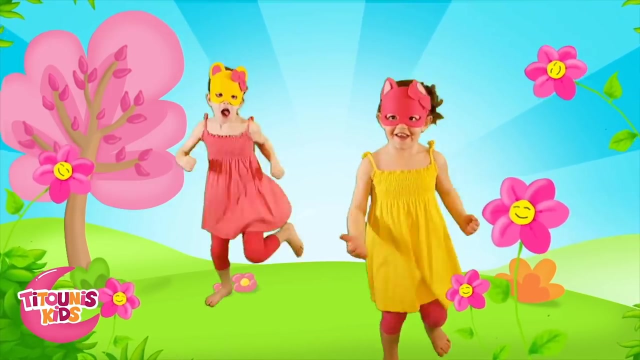 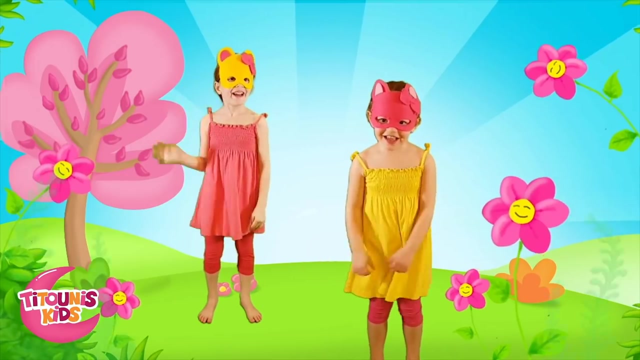 Wow, you're going so fast. Let's pause for a bit and breathe deep, Then start to walk again calmly. Come on, now we're going to the beach and we have to run. Phew Woof, It's so hot. How about we cool off? 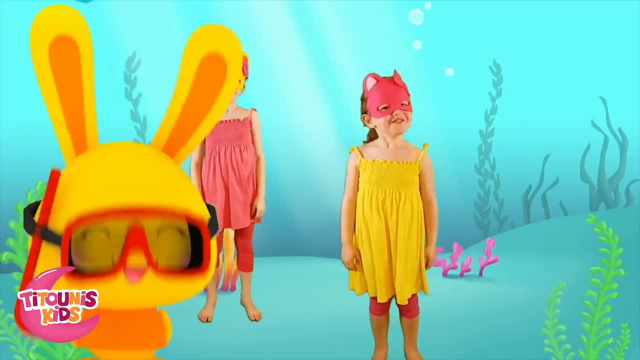 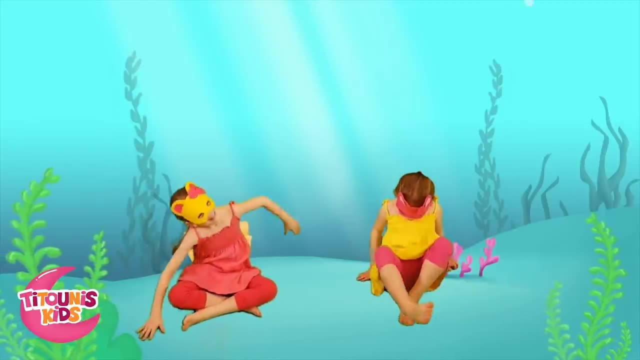 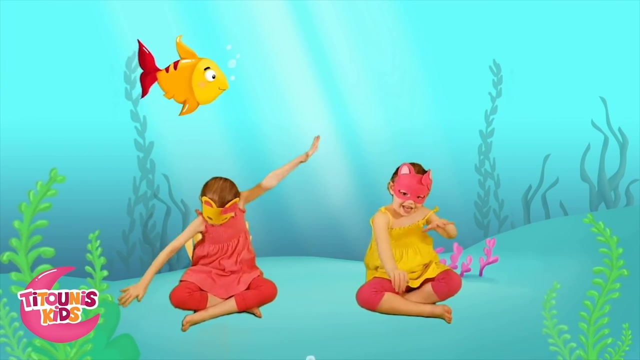 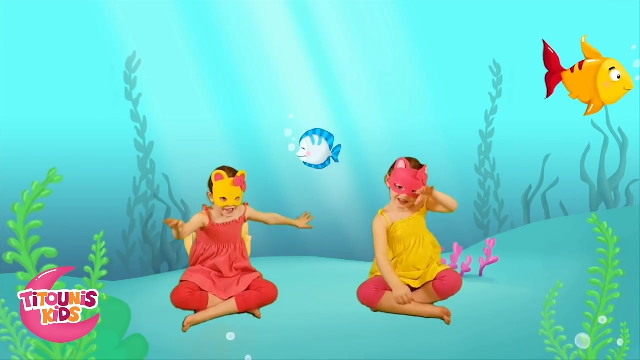 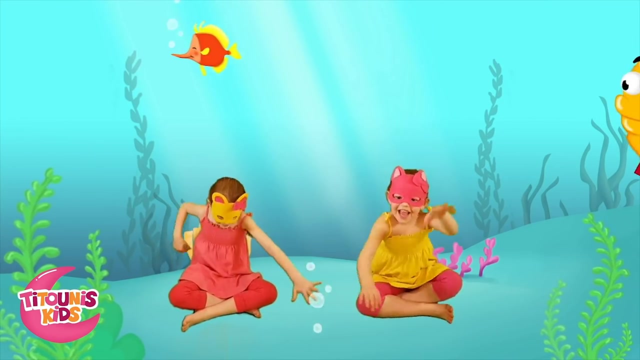 Let's go have some fun with the fishes. Sit down on the floor and swim. Oh, Look at that pretty little fish. Can you say hello? Let's keep swimming Faster. There's a big fish in the water, Can you see it? 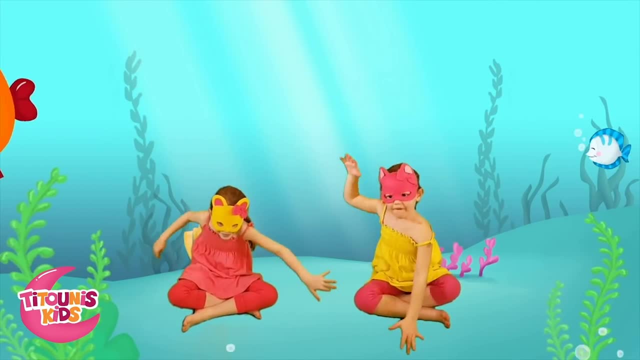 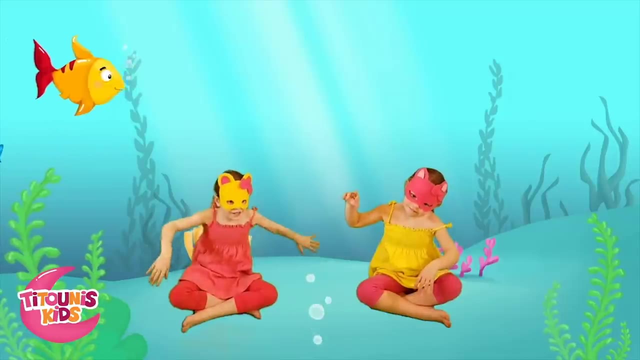 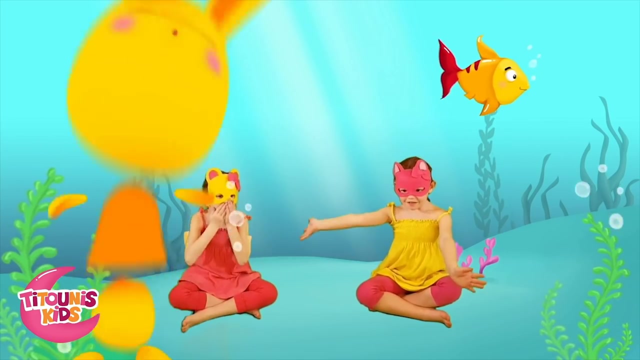 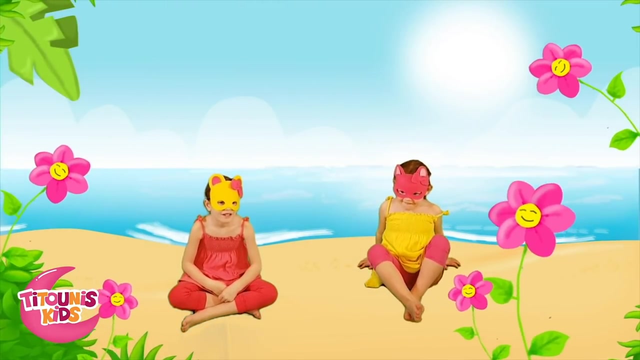 We have to catch it. What about swimming very slowly now? Great, Just like that. Look, The little fish is back. Let's blow a kiss and say goodbye. Now we are in the seashore. What if we pedal for a while? It's so much fun. 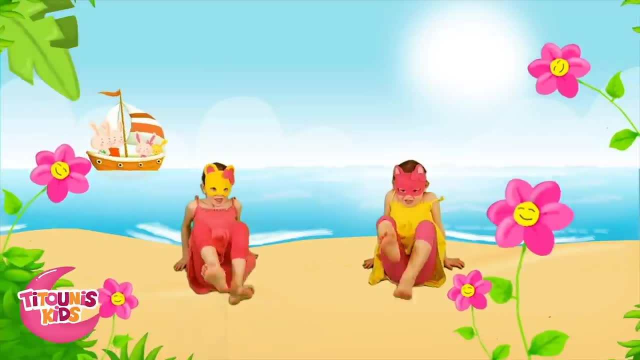 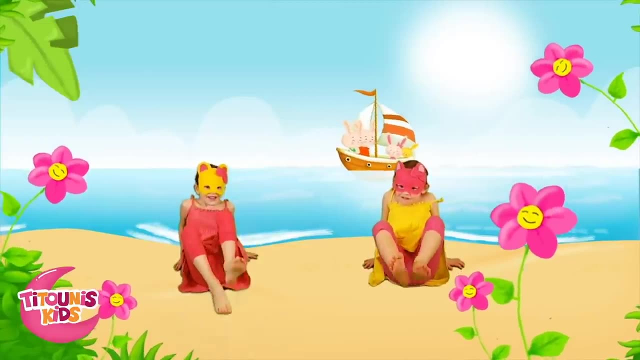 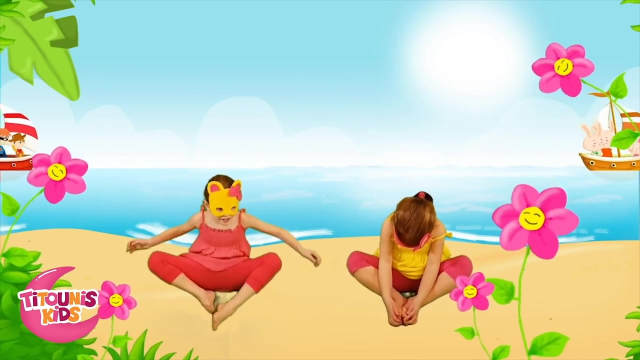 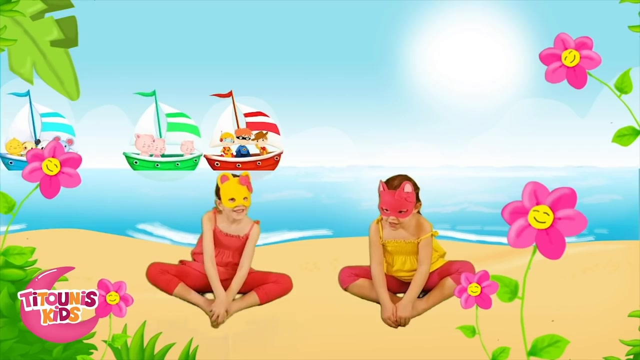 Put your legs up and move your feet. Look, There's a little boat in the sea And it's swinging. Can you swing too? Bend your knees like this, hold your feet and swing like a boat. Let's try something a little harder. 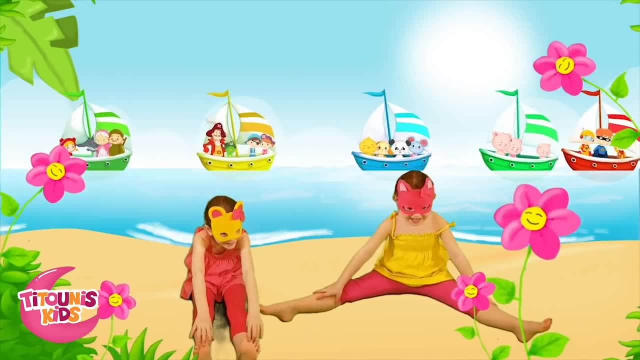 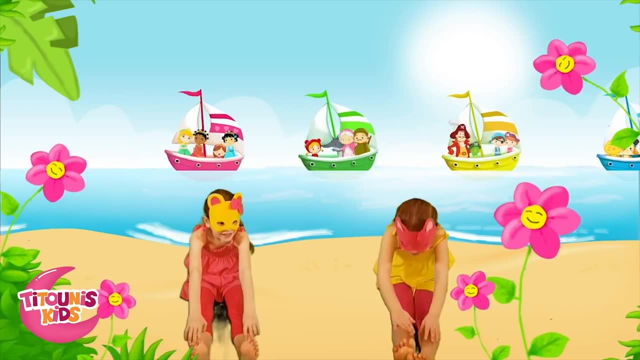 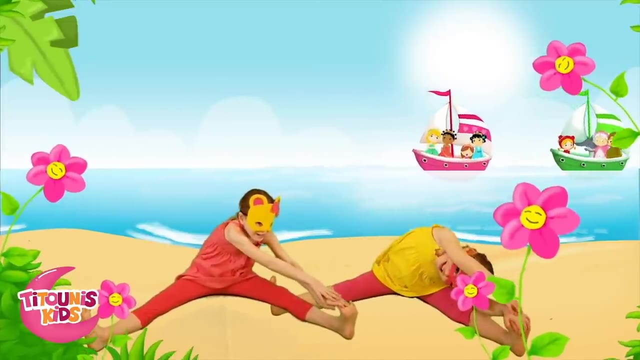 Stretch your legs as much as you can And try to touch the tips of your feet with your fingers. You're doing a great job. Now spread your legs and touch your right foot. There you go, And now switch and touch your left foot. 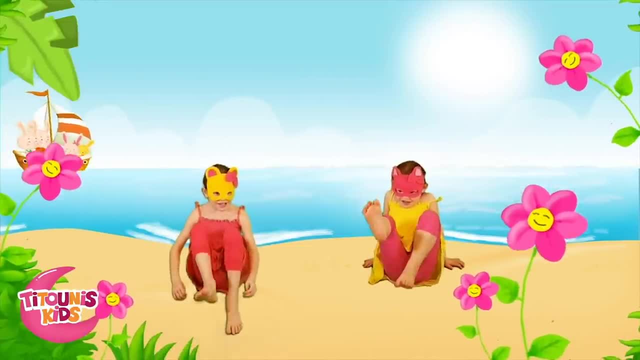 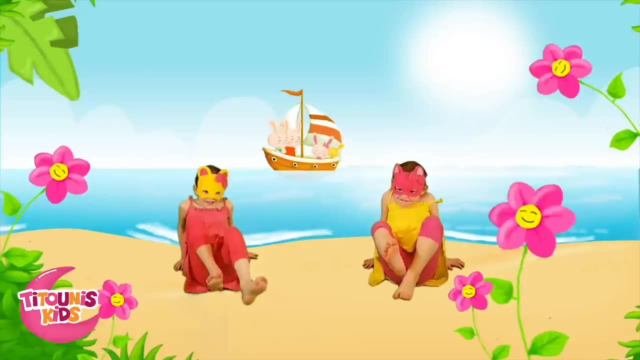 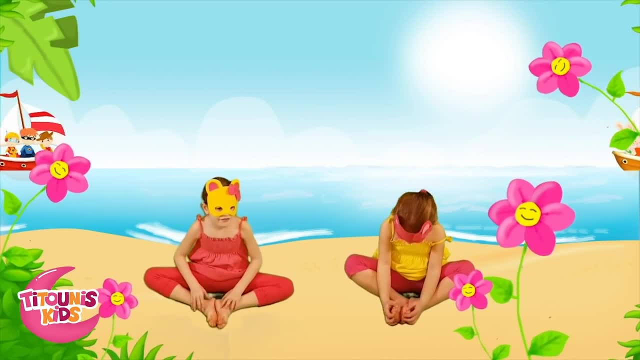 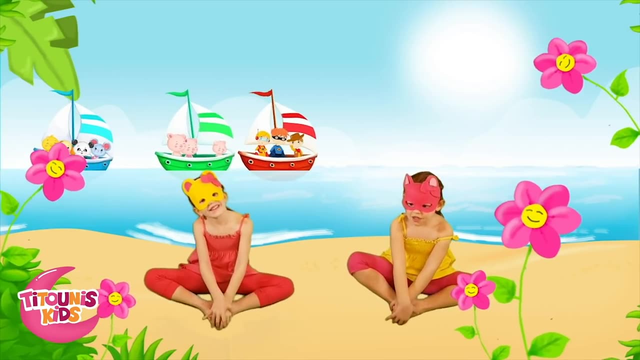 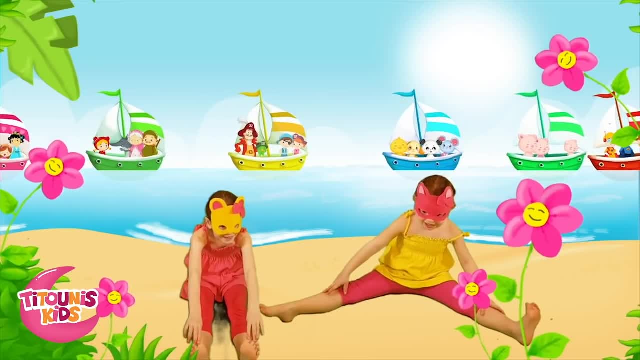 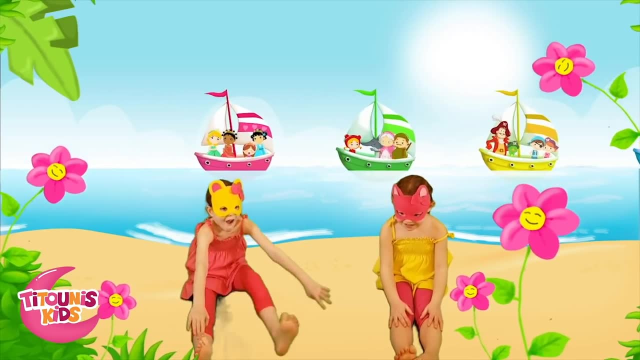 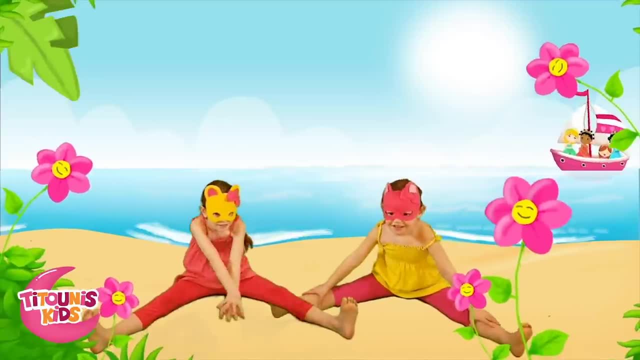 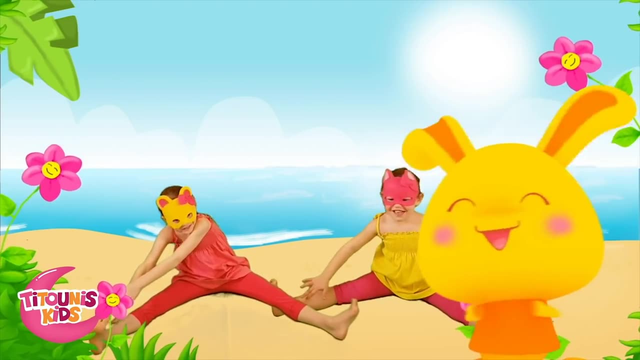 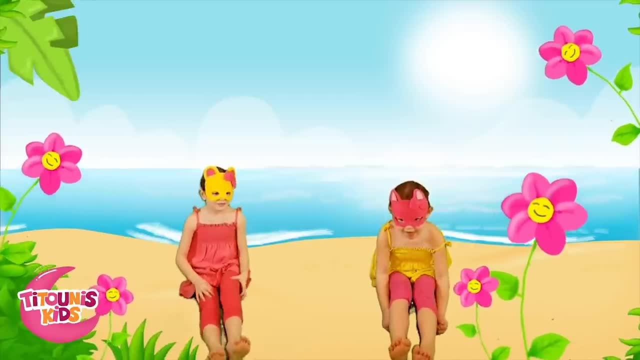 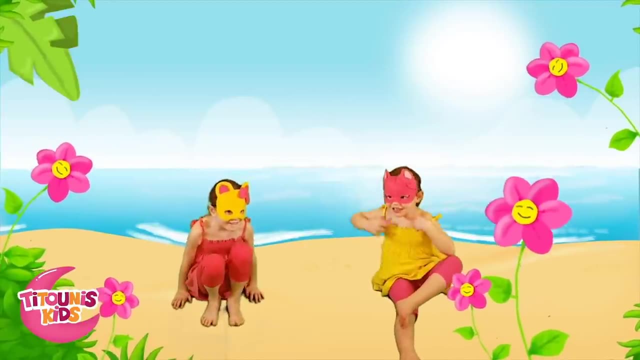 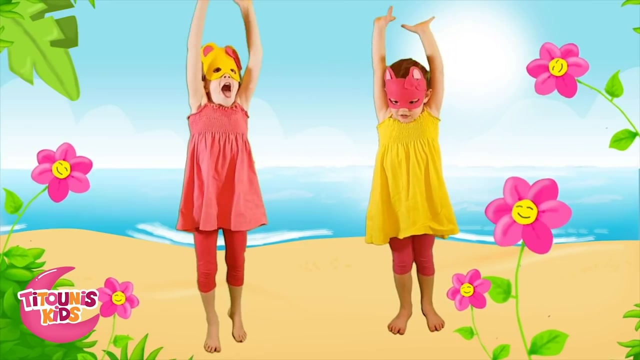 Woof, Woof, Oh wow, Did you hear that They're little birds? Should we try to catch them? Stand up and stretch your arms out as much as you can. Try and touch the sky just a little bit more. 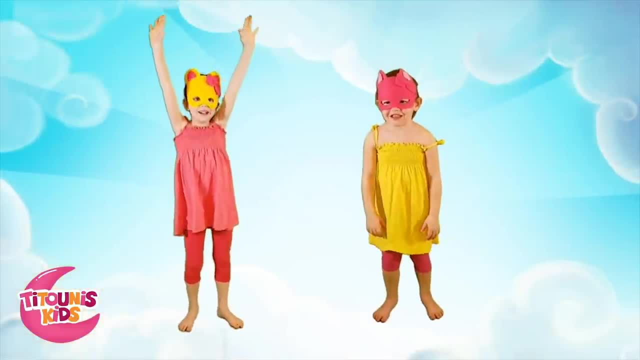 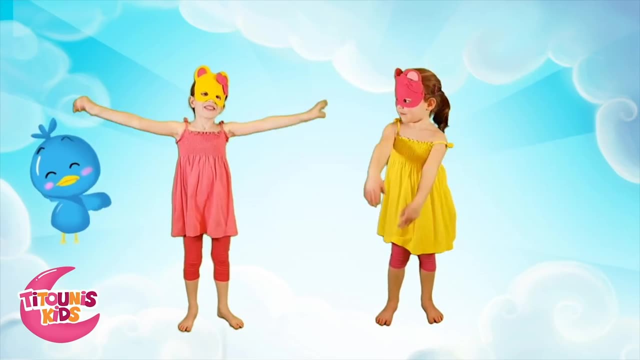 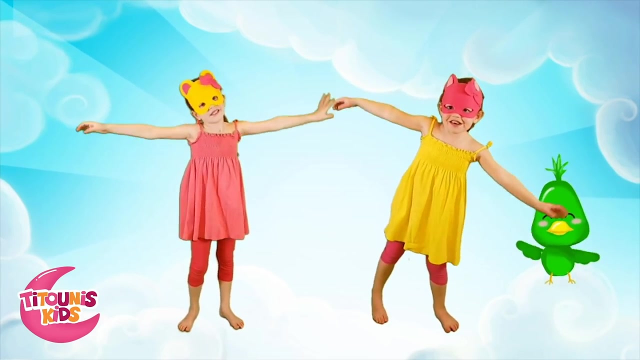 Stand on your toes. Wow, Look how high you've climbed. Now we're on top of a cloud. Stretch out your arms again and fly like our bird friends. do Turn. a little to the right and now a little to the left. Again to the right and now to the left. 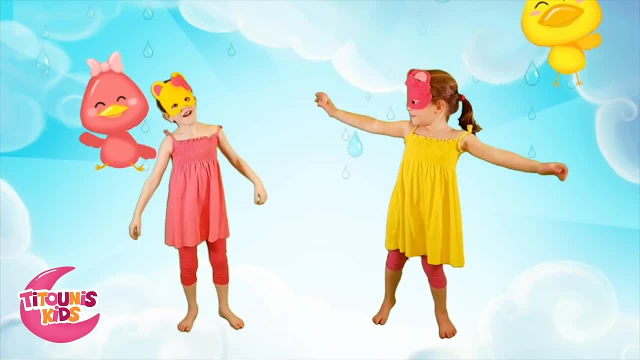 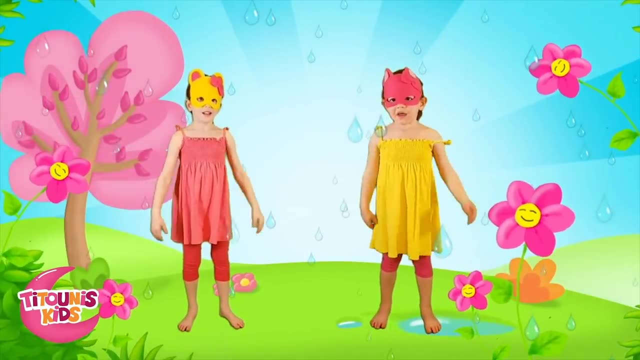 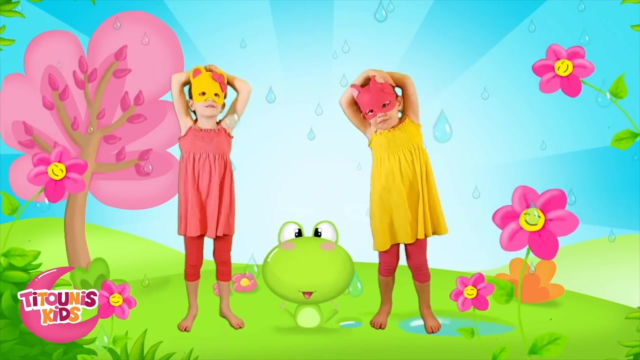 Perfect. Oh no, It started raining. Fly a little more, and then let's land. Put your arms over your head to protect you from the rain and fly a little more And move from left to right. Oh look, who's come to visit us. 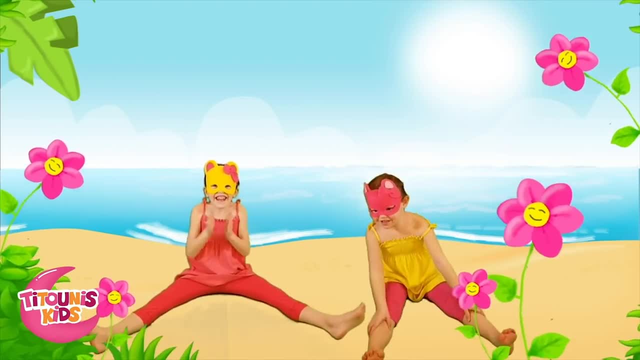 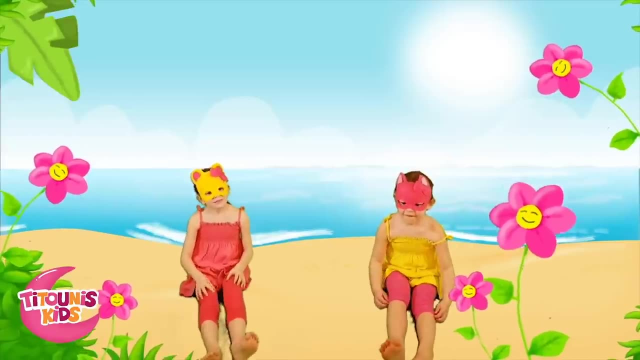 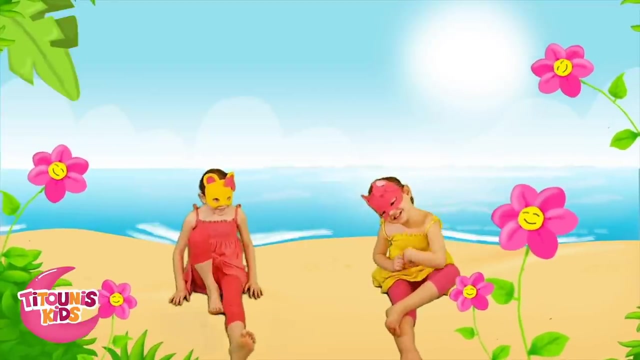 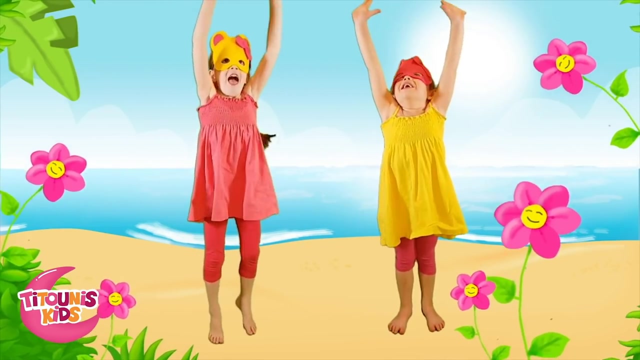 Great, Let's take a deep breath. Oh Wow, Did you hear that? They're little birds? Let's try to catch them. Stand up and stretch your arms out As much as you can. Try and touch the sky Just a little bit more. 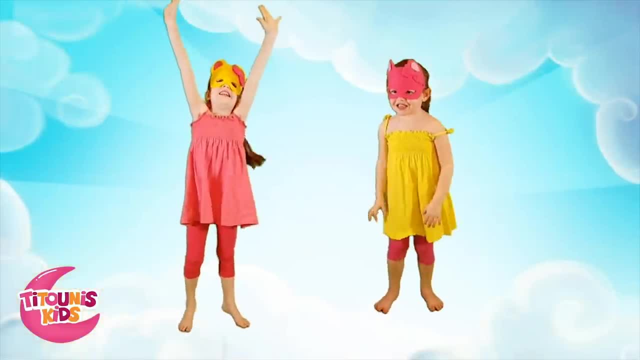 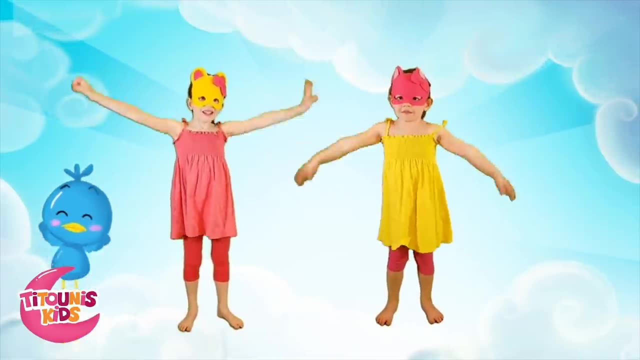 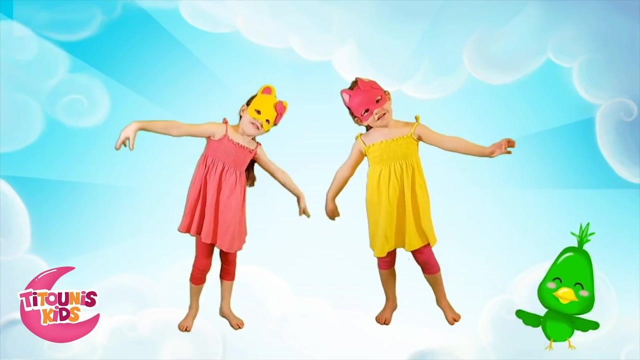 Stand on your toes. Wow, Look how high you've climbed. Now we're on top of a cloud. Stretch out your arms again and fly like our bird friends do Turn a little to the right And now a little to the left. 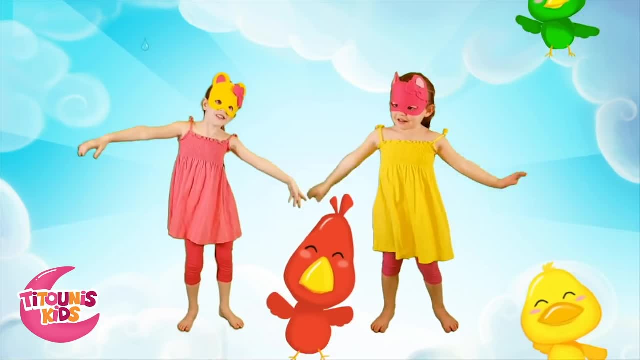 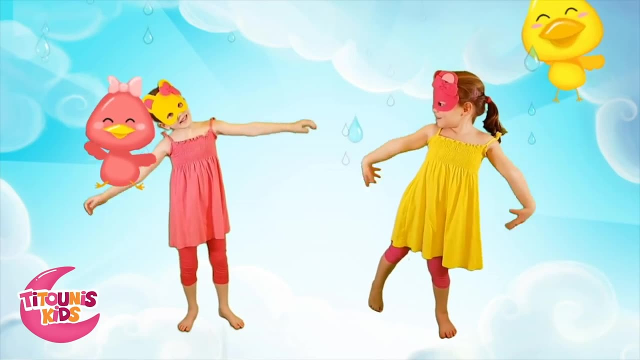 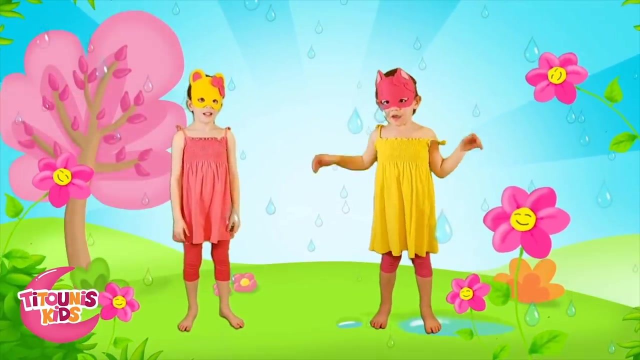 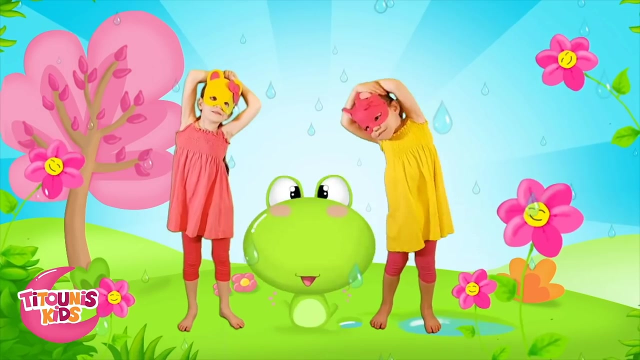 Again to the right And now to the left- Perfect. Oh no, It started raining. Fly a little more and then let's land, Put your arms over your head to protect you from the rain And move from left to right. Oh Look, who's come to visit us. 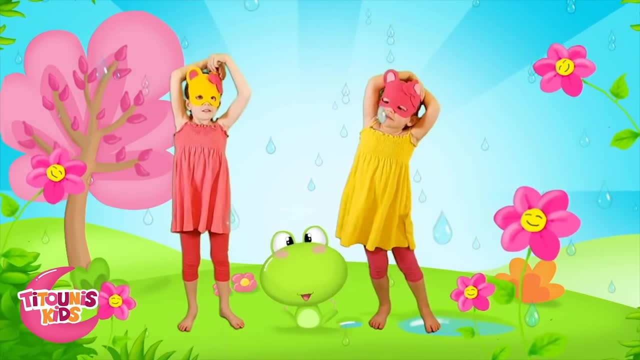 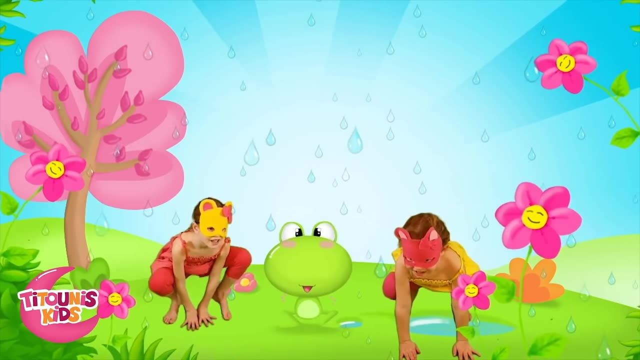 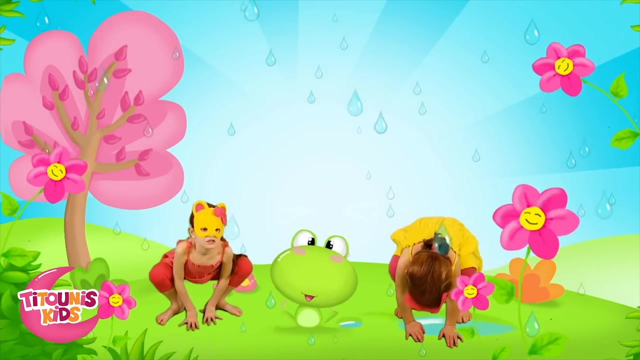 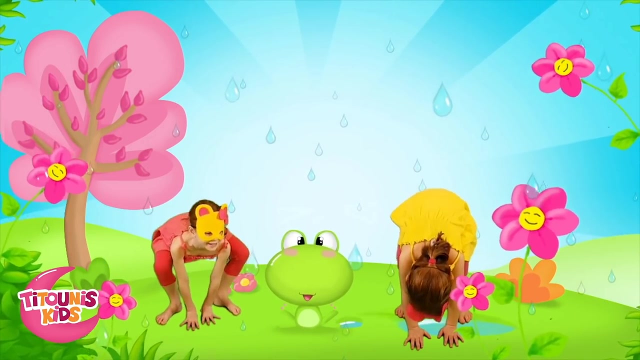 Mrs Frog, Hello, Mrs Frog, Let's copy: Mrs Frog Squat down just like frogs do. Great, Now go up and down like you're going to take a big jump. How nice You look like real frogs. Shall we sing a song. 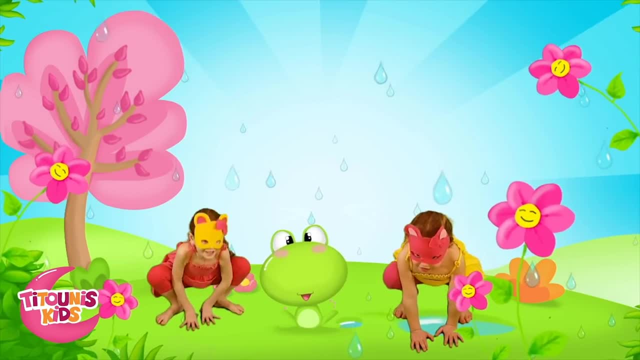 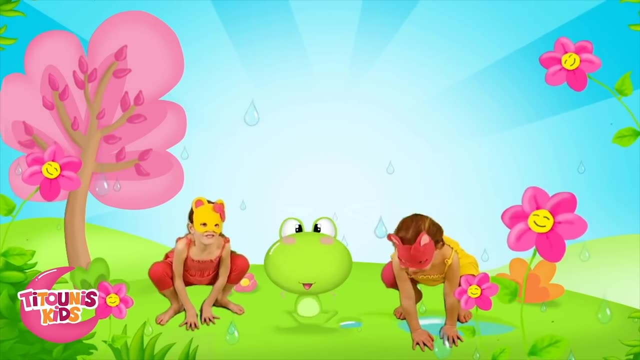 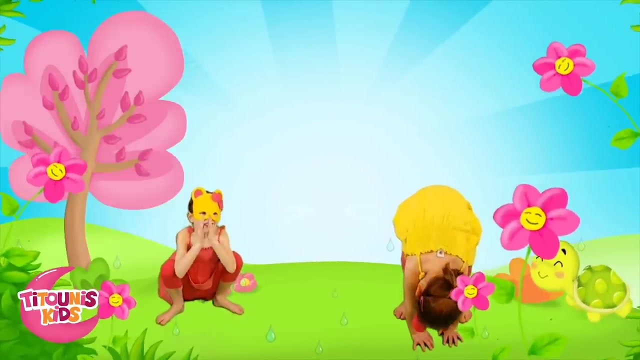 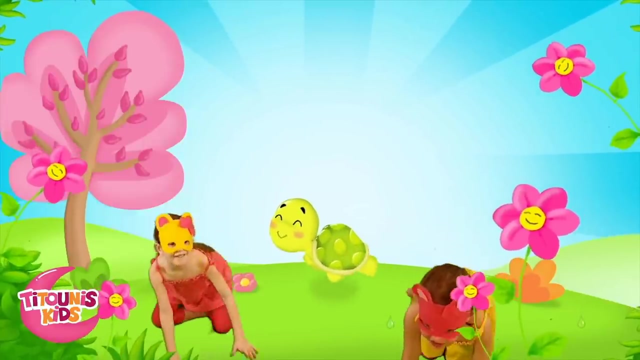 It rains a lot, It's the party of the frog, And if it rains a little more, You should join your friend the frog. Look, It's not raining anymore. And since it's not raining, A turtle has gone for a walk. We're going to mimic her. 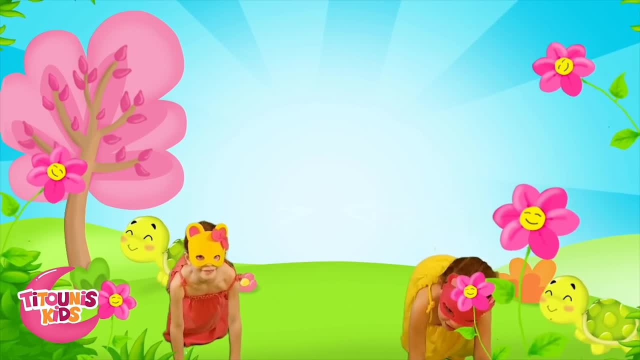 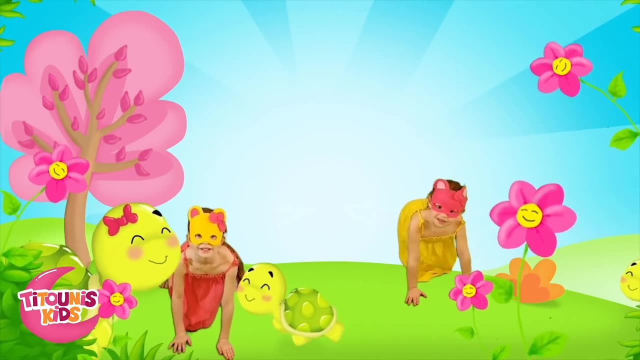 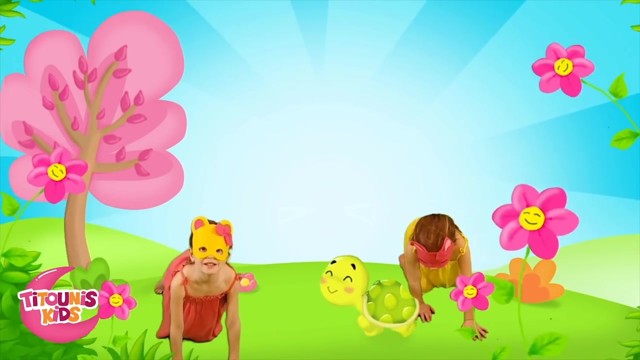 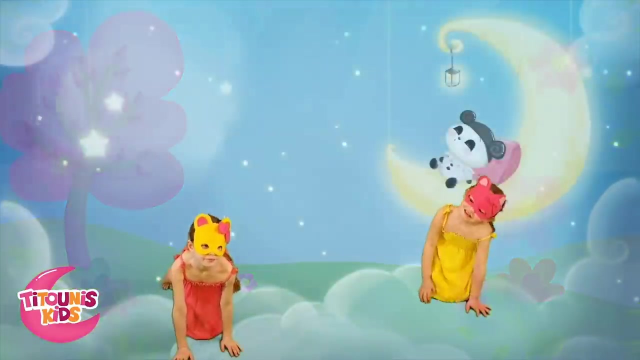 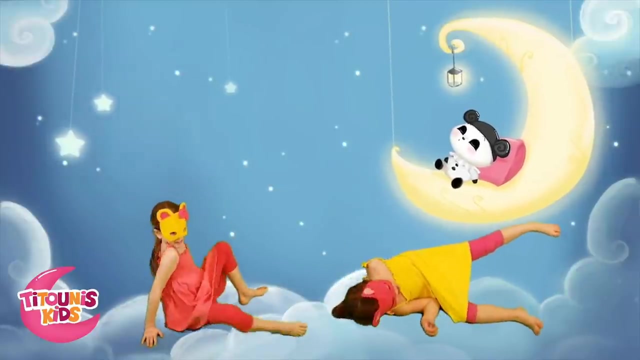 Get down on all fours And move forward very slowly. Amazing, Wow, The whole turtle family is out for a walk. Let's keep walking too. We're a little late And night is falling. Let's go to bed, Breathe deep. 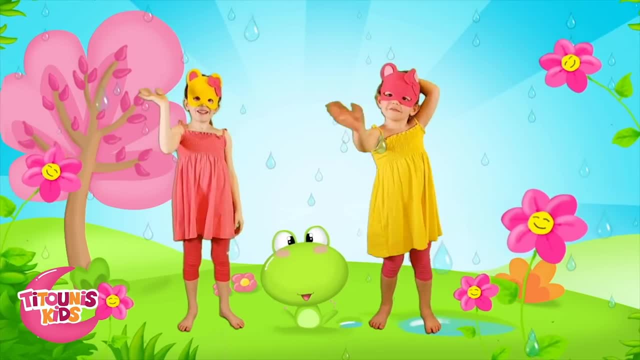 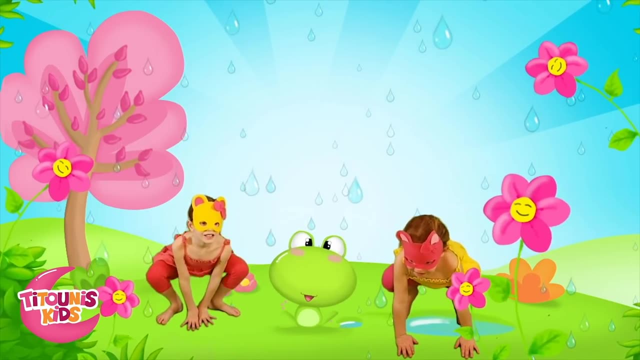 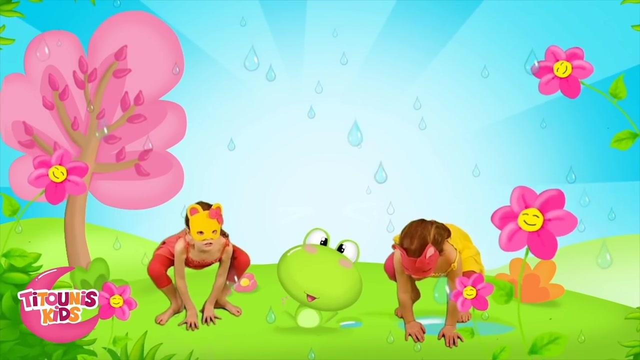 Mrs Frog. Hello, Mrs Frog, Let's copy: Mrs Frog Squat down just like frogs do. Great, Now go up and down like you're going to take a big jump. How nice You look like real frogs. 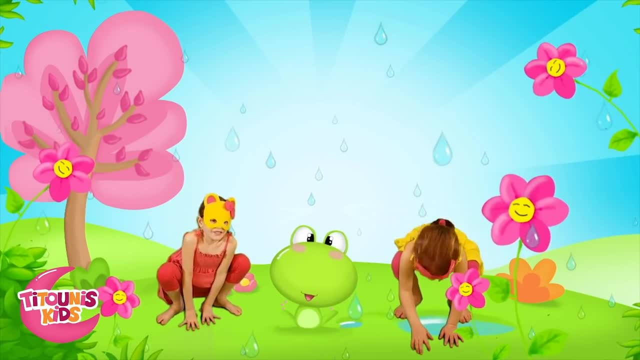 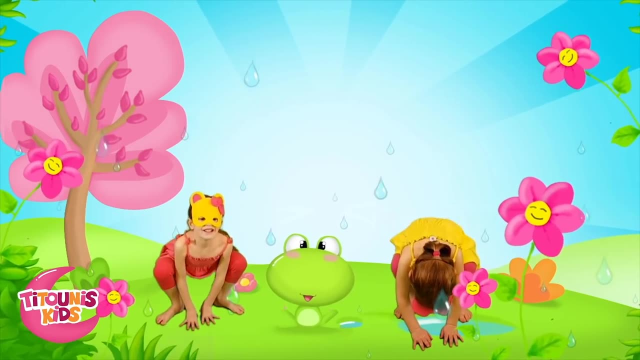 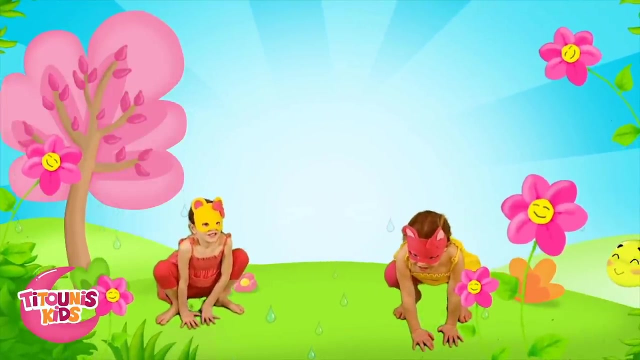 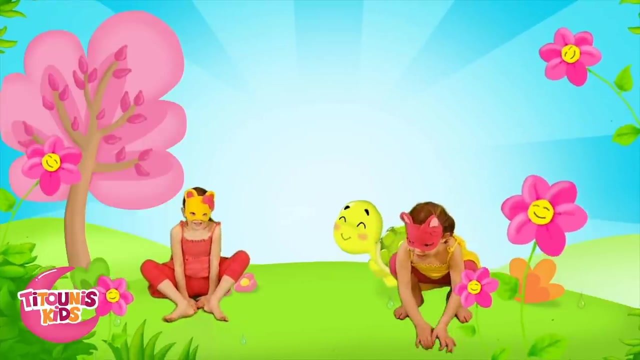 Shall we sing a song? It rains a lot, it's the party of the frog, And if it rains a little more, you should join your friend the frog. Look, It's not raining anymore. And since it's not raining, a turtle has gone for a walk. 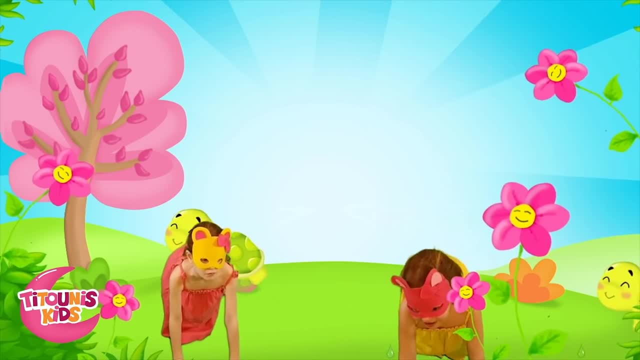 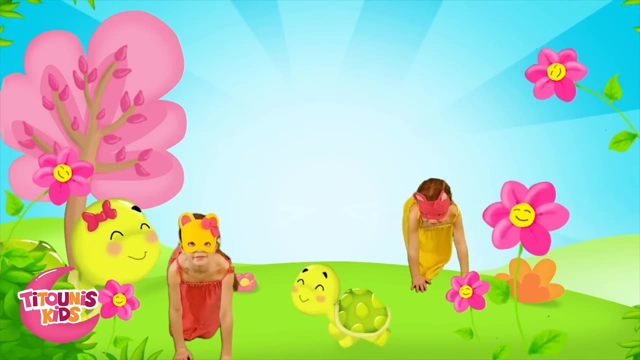 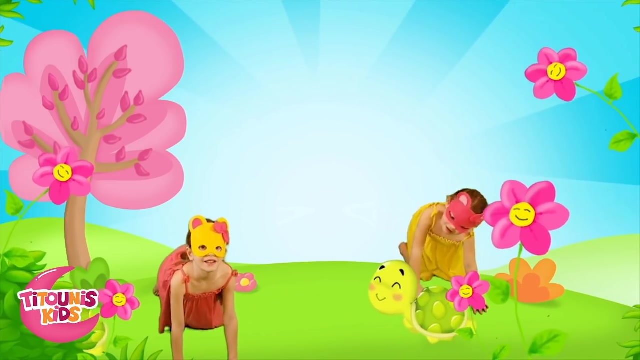 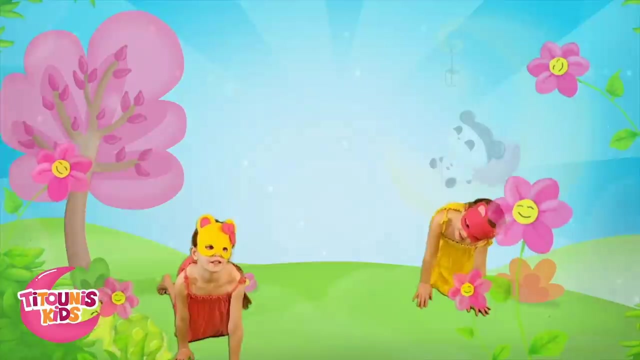 We're going to mimic her, Get down on all fours and move forward very, very slowly. Amazing, Wow, the whole turtle family is out for a walk. Let's keep walking too. We're a little late, A night is falling. 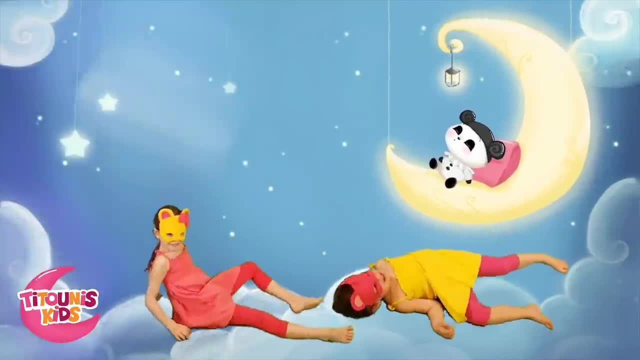 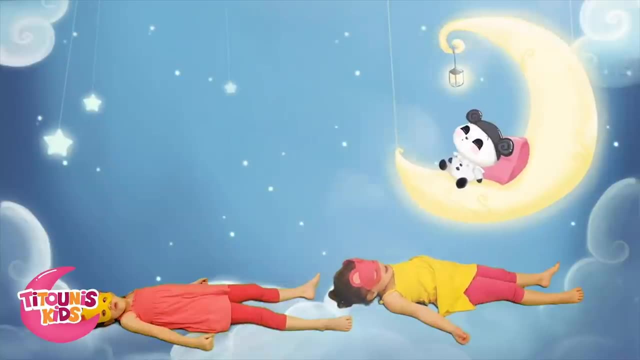 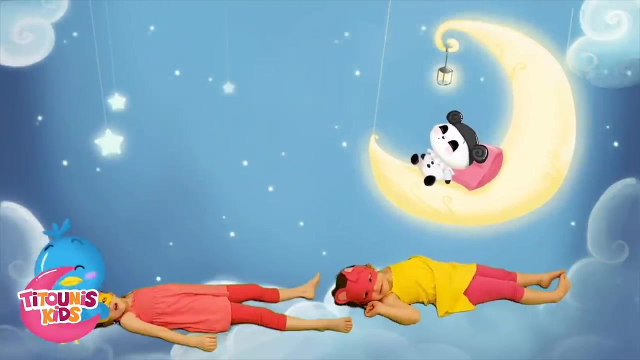 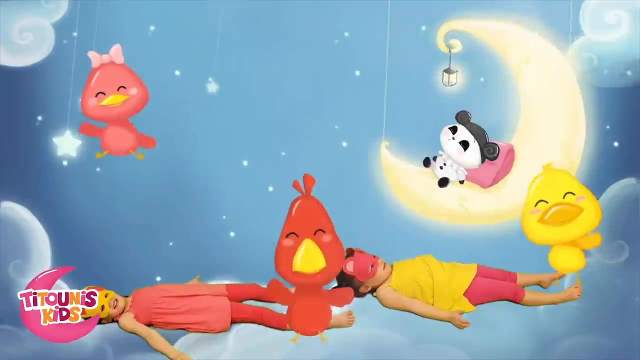 Let's go to bed, Breathe deep, Breathe in and out. Oh, are you hearing that? Look up, It's the little birds we saw before. They're saying goodnight to us. Goodnight, little birds. 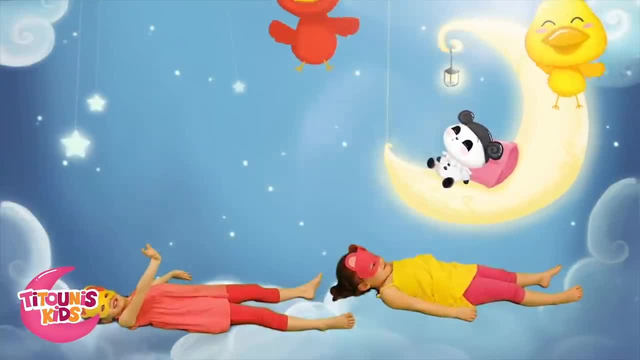 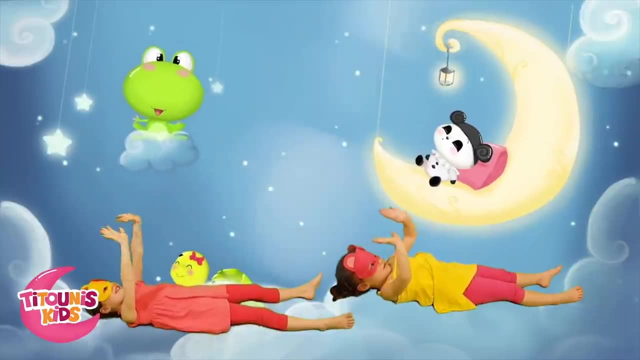 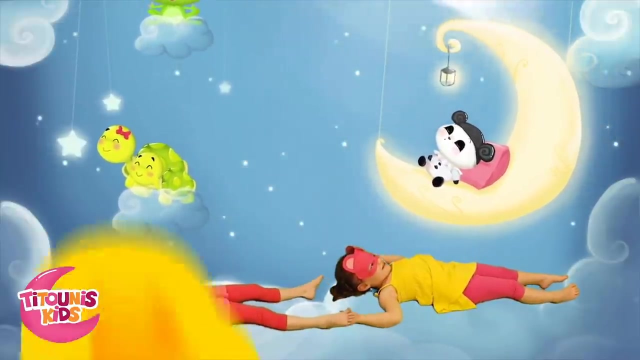 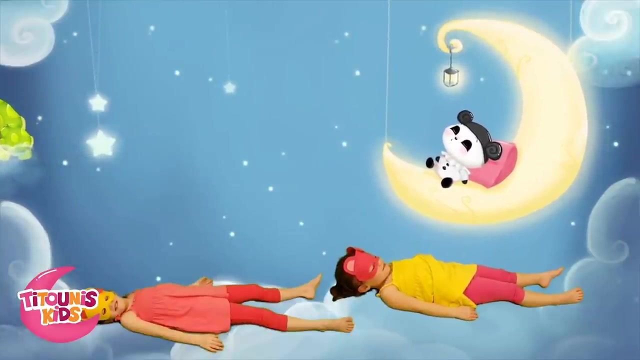 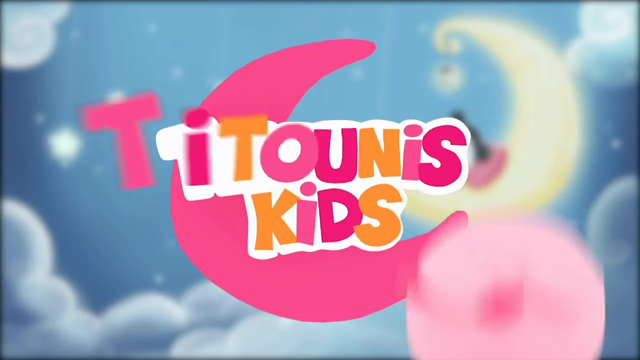 Sweet dreams. And also Mrs Frog And the turtle family Go to sleep. Sweet dreams, Goodnight everybody. Goodnight everybody.